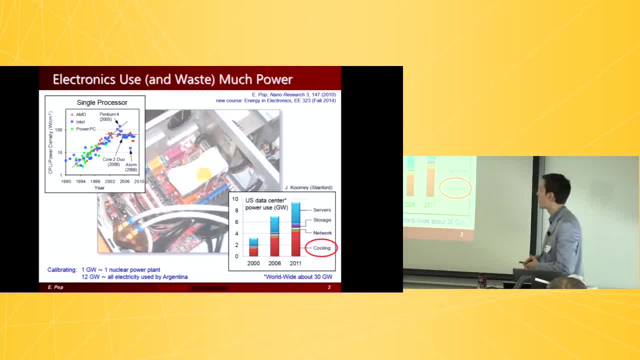 Of course, for ATOM, ARM and other kind of mobile processors At the other end of the power spectrum- and I'm not going to talk about data centers today, but the other end of the power spectrum- are data centers, And here's some numbers about data centers in the US. 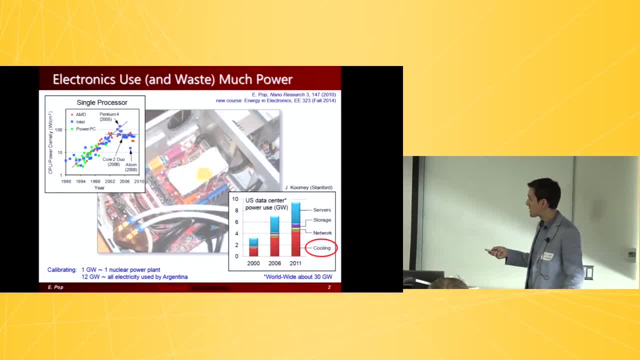 These are very large numbers. by the way, These are gigawatts. So if you look over the last 10 years or so- 15 years actually- data center power usage in the US has been doubling about every five years. okay, 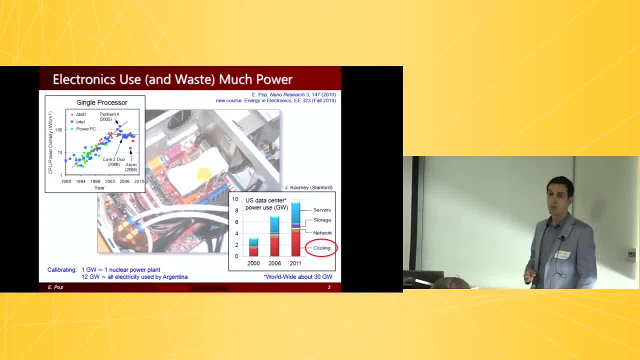 We've gone from about 3 gigawatts per square centimeter to about 5 gigawatts per square centimeter. We've gone from 5 gigawatts all the way to about 10, 11 gigawatts today. About half of that is used for cooling actually. 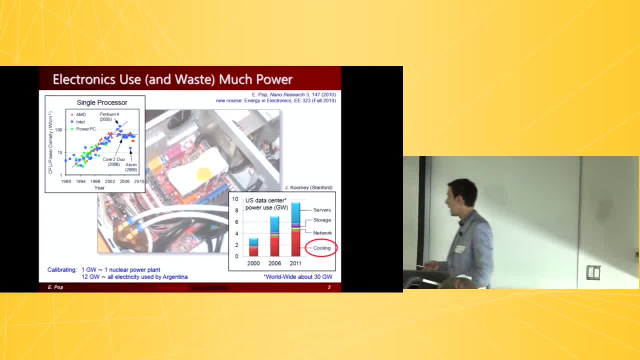 So not all of it is used for computing right Worldwide. I am told by people who study these things that the data centers in the whole world are about 30 gigawatts And again, like I said, these are very large numbers. 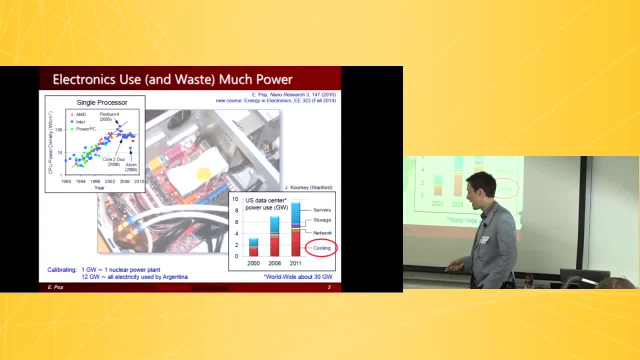 And I'm more used to working with nanojoules and femtowatts, and you know femtojoules and nanowatts, those kinds of numbers, So I looked it up. A gigawatt is the power generated by one large nuclear power plant. 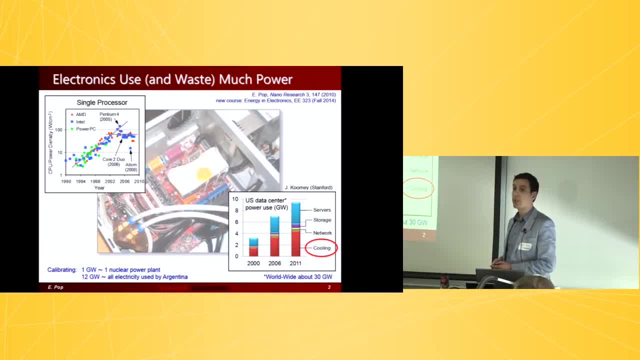 And 12 gigawatts is the electricity used by the entire country of Argentina, right? So the data centers in the US today are using as much electricity as the country of Argentina, just to kind of put things into perspective. Okay, So you know, we're obviously an academic group. 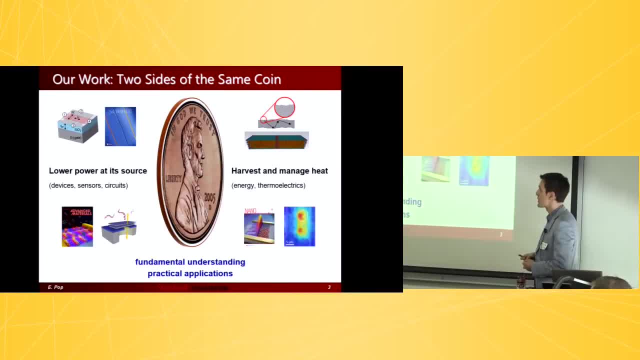 We don't work necessarily on data centers, although I find these things interesting. The way I like to think about what we do is sort of looking at two sides of the same coin. On one thing, we sort of wonder where the power comes from and what we can do about that. 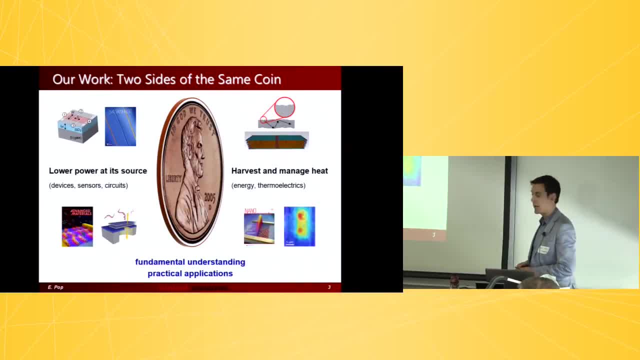 And on the other side, which is obviously more of the topic of this talk, is how to harvest and manage the heat that is generated in electronics anyway. Of course we're academic, so we're always interested in fundamentals, But we're engineers so we also want to make sure. 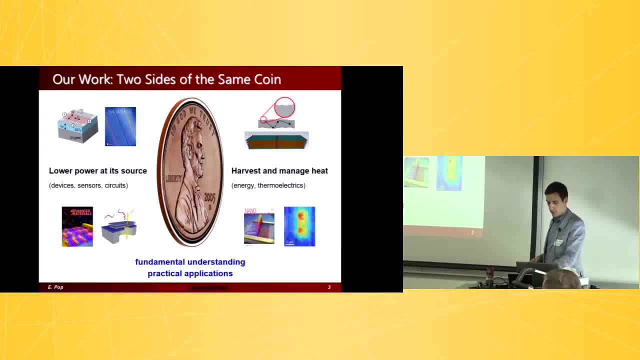 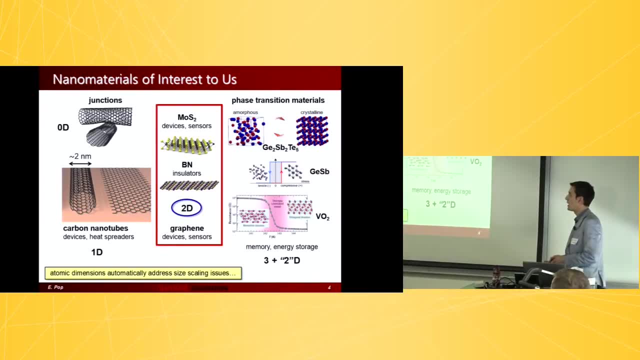 that what we do is connected to practical applications, And so you know, really quickly moving into materials, The materials that my group typically looks at are shown over here. I like to group them by dimensionality, so they range from 0D all the way to 3.0.. 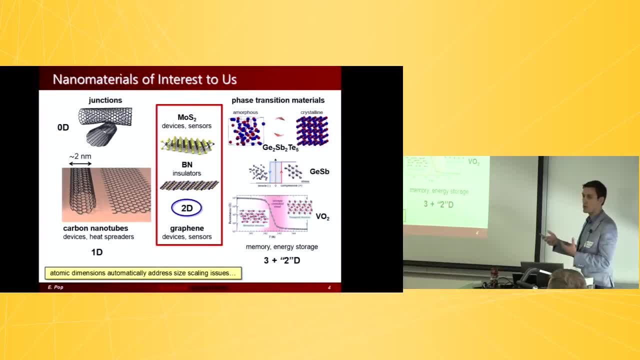 Okay, So these are what I call plus 2D. These are 3D materials that have two extra degrees of freedom in terms of phase change, metal insulating, essentially materials, But the subject of today's talk is 2D materials, and here's a bunch of them. 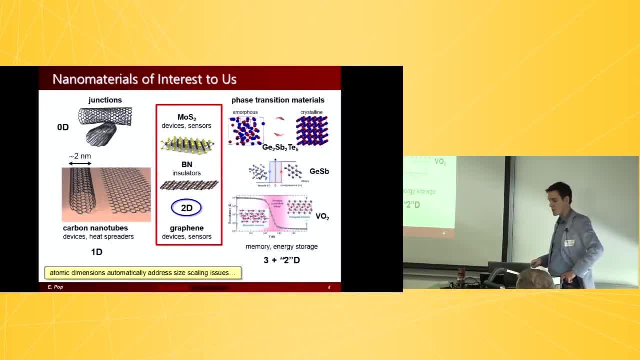 And of course these require no introduction, especially after the two really nice talks this morning. I just want to mention that one thing that sort of sometimes is on our mind is that the atomic dimensions of especially 1D and 2D materials automatically in some way address some size scaling issues. 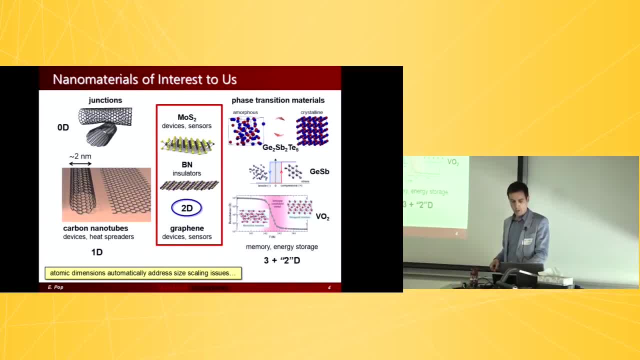 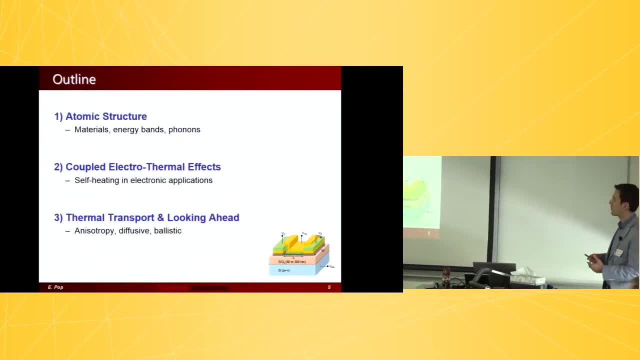 which Moore's Law obviously has been driving us towards for many, many decades now. Okay, So as an outline of my talk, here's essentially what I'll be talking about for the next 40 minutes or so: Atomic structure, energy bands and phonons. some electrothermal effects in the context of devices. 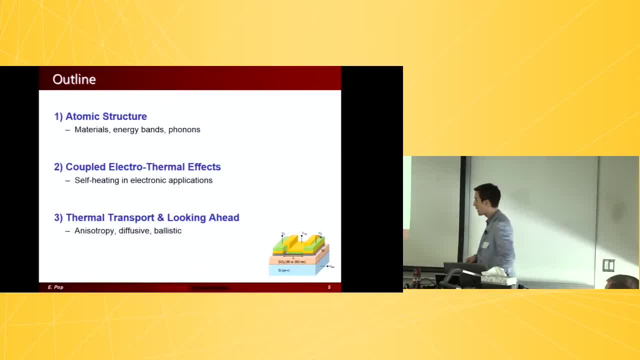 Right, So I'll be trying to tie into the earlier talk And then looking at some of the basics, more fundamentals, of thermal transport and also trying to look ahead What these are, What these might mean from a functional point of view for these materials. 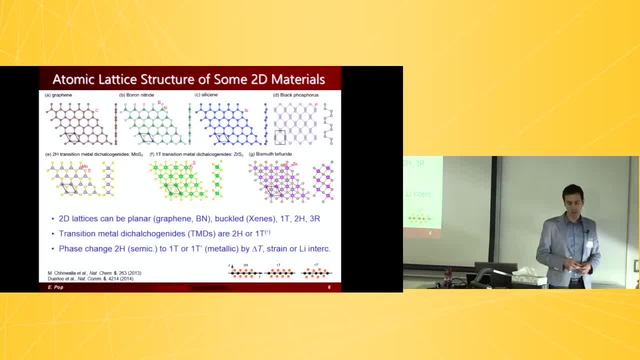 So this is the first part of my talk. Okay, I think you've seen this before as well, So just kind of a recap. The atomic lattice structure of some 2D materials- graphene, of course, is shown there. boron nitride. 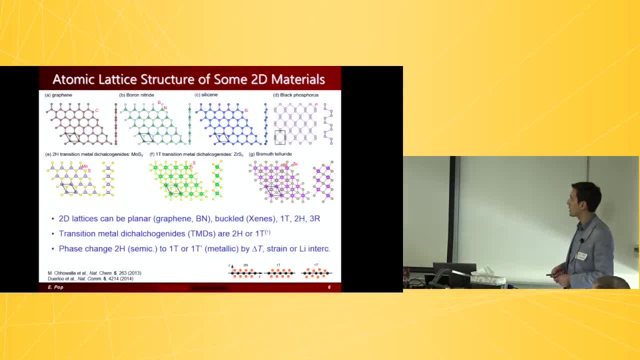 silicene, these TMDs, transitional metal dichalcogenides, black phosphorus and isotropic, of course, Right. So these things are typically 2H or 1T, sometimes 1T prime, which is a distorted 1T lattice. 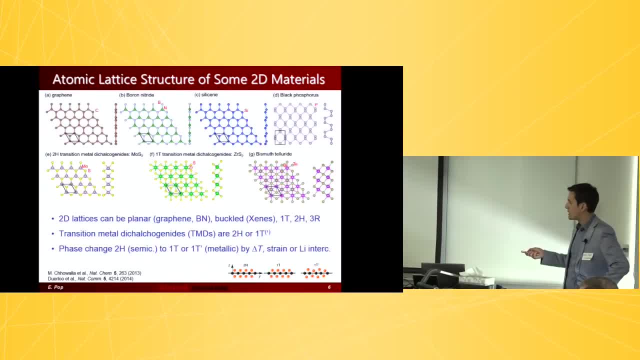 There's also phase change properties of these TMDs between the 2H semiconducting state and the 1T or 1T prime metallic state. These things can be induced, for example, in molybdenum telluride by temperature strain. 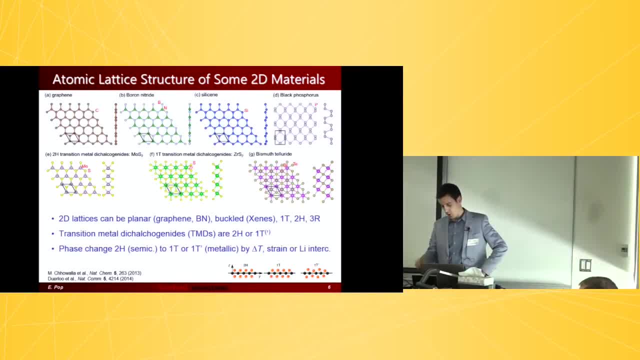 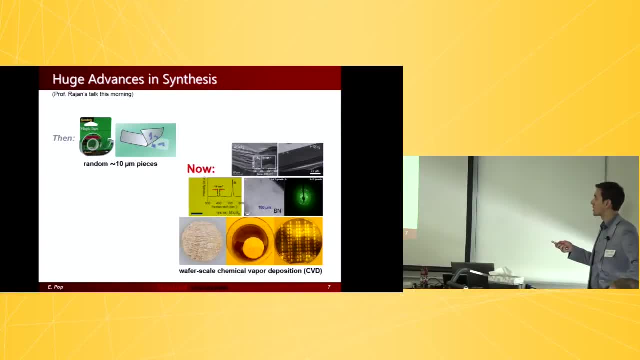 or by lithium intercalation, as people have shown, Actually also in MOS2.. This is really just a tribute to Professor Rajan's talk this morning, or rather my tribute to his talk. Then you know back maybe 10 years ago or so, right when this whole field kind of started. 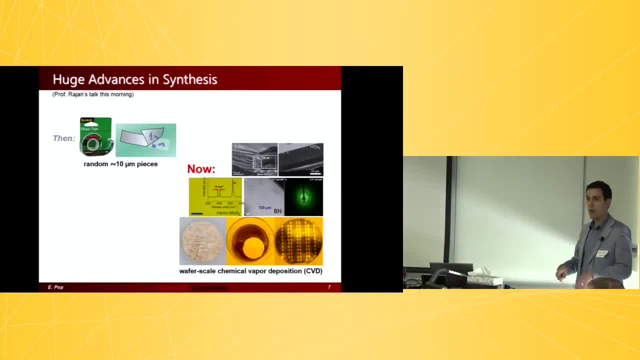 we were working with a whole bunch of scotch tape and getting sort of random, you know, 10 micron at best- pieces of junk. you know that we would make devices on. And today of course we have large scale, mostly CVD methods, at least in my group. 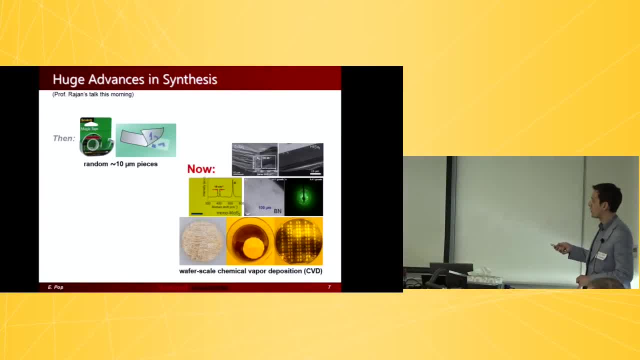 And this is graphene, of course, on 4-inch sort of copper foils: boron nitride, molybdenum sulfide, and this is graphene, And then some of the weirder TMDs that I'll talk about a little bit later. 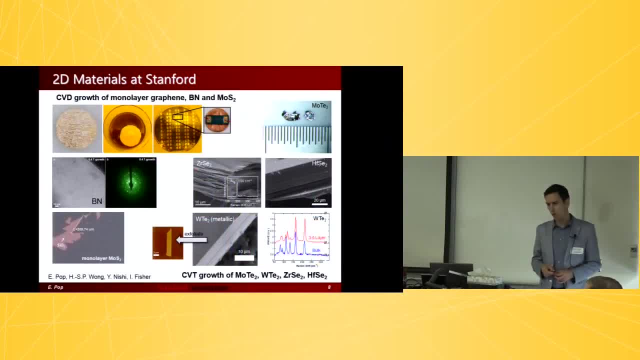 In fact, just kind of to highlight some of the growth that is happening at Stanford. this is more of a Stanford-specific slide. This is our collaboration with Philip Wong, Yoshua Nishi and Ian Fisher in the physics department- Basically the capabilities that we have right now at Stanford. what we're playing with? 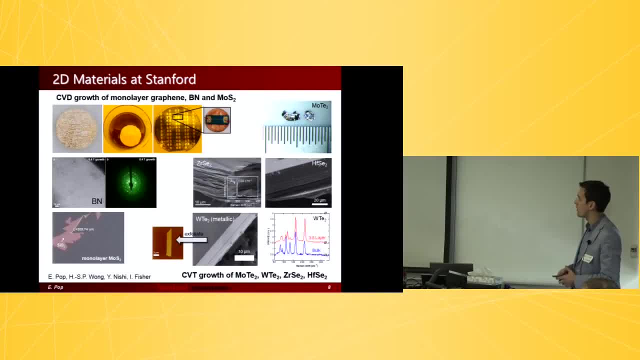 are these 4-inch graphene growth system for, actually for circuit applications? That's where we're driving that. We have a 2-inch boron nitride growth system And that's coming online nicely. We're really looking forward to actually making devices on CVD-grown boron nitride monolayer. 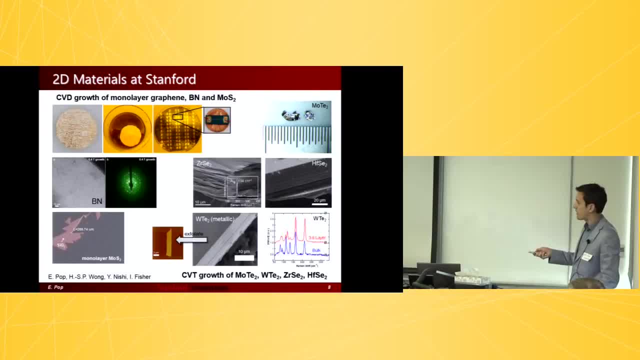 self-limiting stuff. And then, I think like a lot of people, we've been able to grow monolayer molybdenum sulfide by CVD with properties almost approaching those of the exfoliated stuff. And then we have another thing called chemical vapor transport. 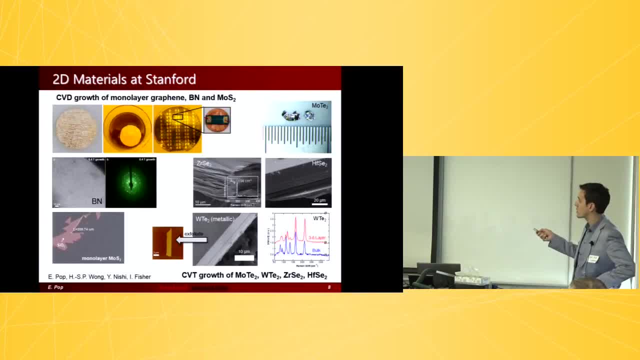 And here we don't actually grow monolayers, We grow multilayer, sort of thick millimeter scale films. And then we still have a lot of things that we're working on. We still have to rely on the scotch tape to essentially peel these apart and do individual devices. 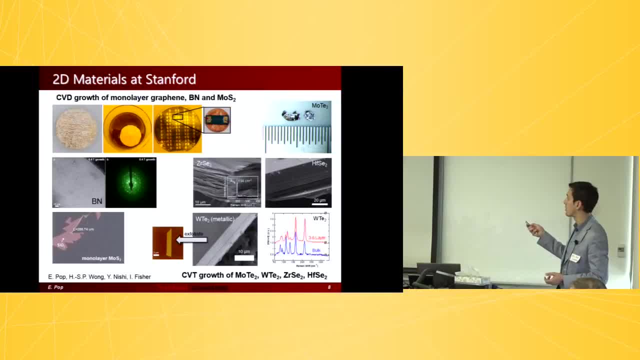 But these are some of the what I call the weirder TMDs. These are molybdenum telluride, which is a phase change material, Zirconium selenide, hafnium selenide, which have lower band gaps among the TMDs. 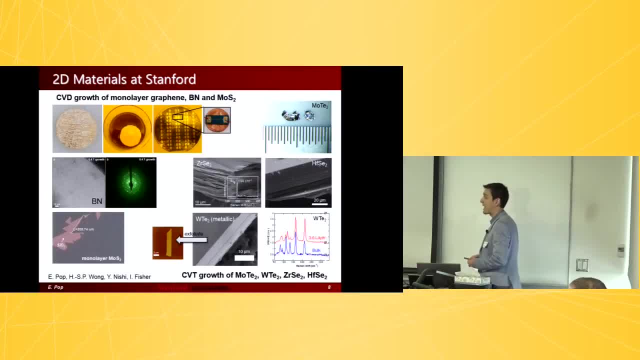 And then tungsten telluride, which shows up as a 1T prime metallic phase every time we grow it, And it's kind of an interesting material by itself, Probably the only 2D material other than graphene that we've worked with. 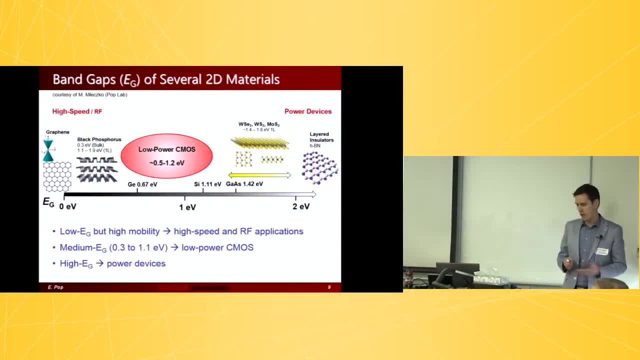 Okay, This is. you know how do you look at 2D materials? I've sort of always scratched my head trying to you know kind of put together the zoo of materials. This is a slide put together by Michael Mletsko in my lab. 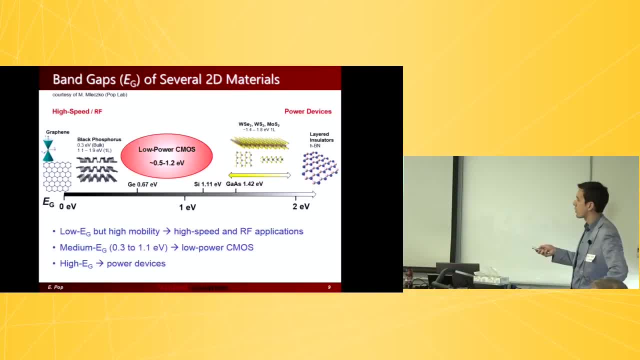 He basically likes to look at these things, as you know, in terms of band gap, for instance, You know, ranging from, obviously you know, very small band gaps, medium, smaller band gaps- Sorry, zero band gap- to small band gaps. 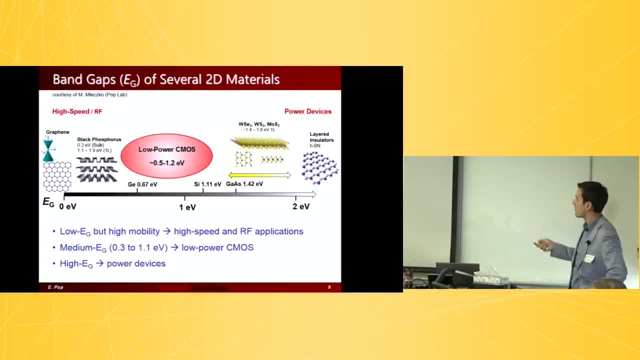 You know, low power CMOS is somewhere in here, And then we have all these Other TMDs with band gaps between 1 and 2 EV, And then, of course, we have the insulators and so on towards the right. 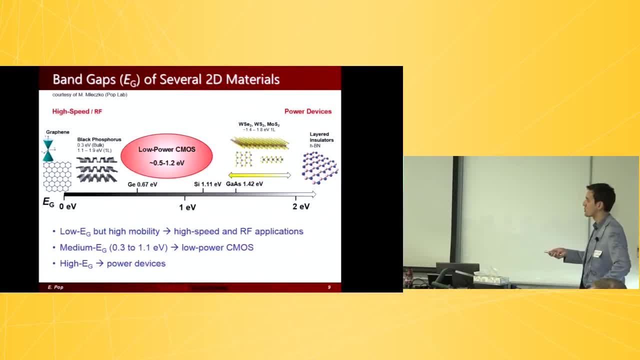 I think you all know this already, especially from Professor Zhu's presentation. But you know, low band gap but high mobility. you could go for high speed or RF applications, Medium band gap, of course, low power CMOS And then larger band gap for power devices perhaps. 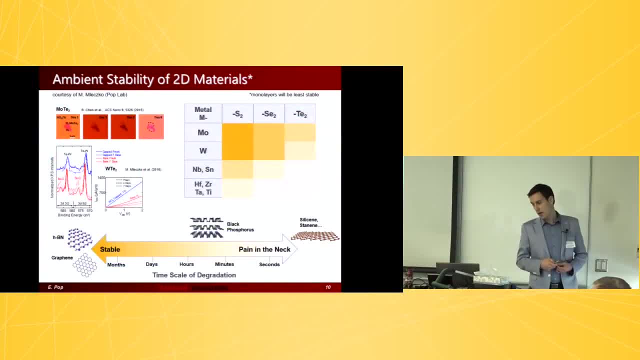 But maybe a more whimsical way to look at 2D materials, Also put together by Michael Mletsko In my lab, is to basically look at them, you know, on a scale from stable to complete pain in the neck. And you know, we know, that boron nitrate and graphene are pretty stable. 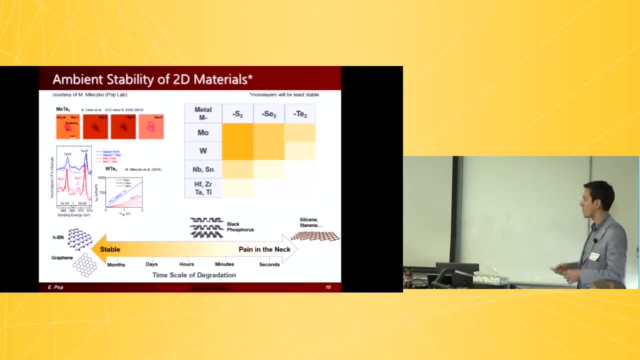 You know you exfoliate or you grow these things and that you can go back and the samples are fine after months. Black phosphorus: you know hours to minutes degradation And then some of the silicene stannine stuff that we've seen seems to be almost instantly degraded. 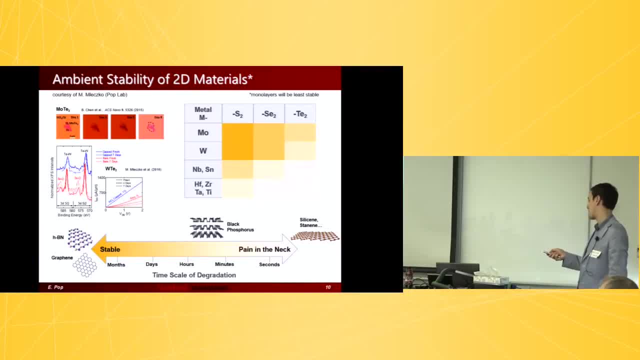 And so this is. you know, I think this is a little bit more complicated. I think this is a little bit. the coloring scheme is not exactly what's on my laptop screen, But you can imagine the color here corresponds to the color down here. 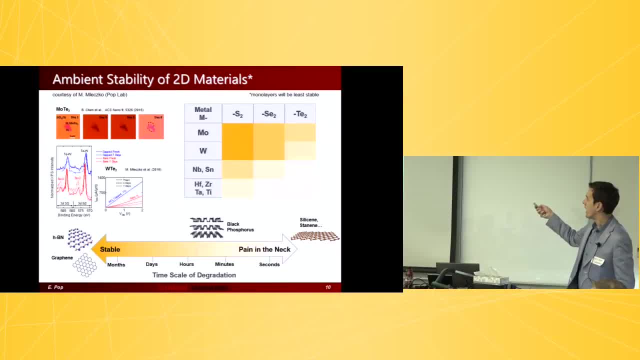 So you know, if you go by the metal and if you go by the chalcogen, like that, Basically, molybdenum sulfide is probably the most stable among these things, And then these zirconium tellurides or hafnium tellurides and so on, going like this: 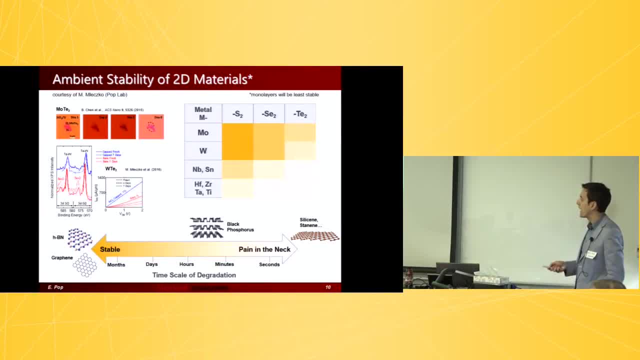 Our experience seems to be the least stable And this sort of goes down. you know the periodic table In terms of the chalcogen Column. I'm sorry, And this seems to roughly scale with a metal reactivity, Especially the metal reactivity with oxygen. 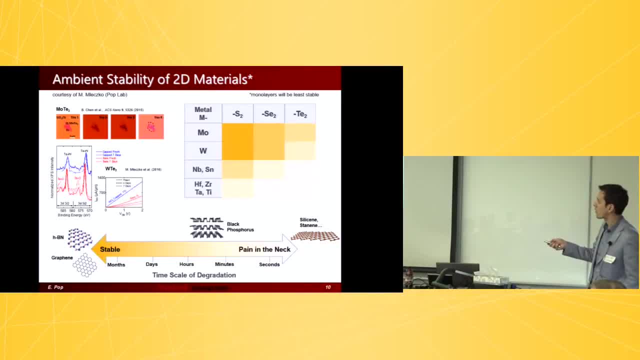 That's what we kind of seem to see, Although it's a little bit harder for me to form sort of an intuitive picture of what's happening there. And again, take this with a big grain of salt because this is quite qualitative, But here's a nice picture from the literature. 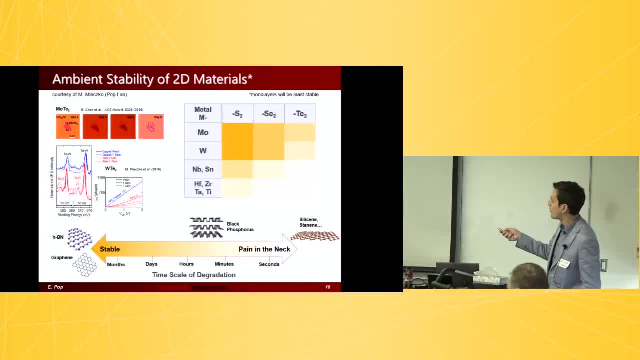 This is molybdenum telluride. I don't know if you can see this in the back. Over a couple of days, you know, monolayer molybdenum telluride essentially disappears, And we see this as well. 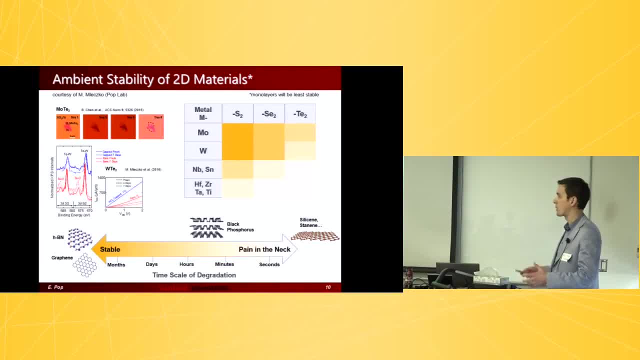 So whenever we work with molybdenum telluride in our lab, you know we try to do the measurements like the same day, right. But if you do them the same day it's kind of okay. Tungsten telluride a little bit more tricky to work with. 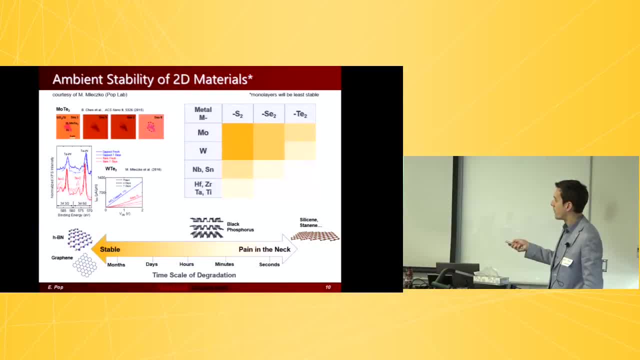 This is work, actually Michael's work. in my group We've done XPS, for instance, after a couple of days And we see tellurium oxide peaks forming. So it's very, very clear what's happening over here. This is the you know, exposed unencapsulated tungsten telluride. 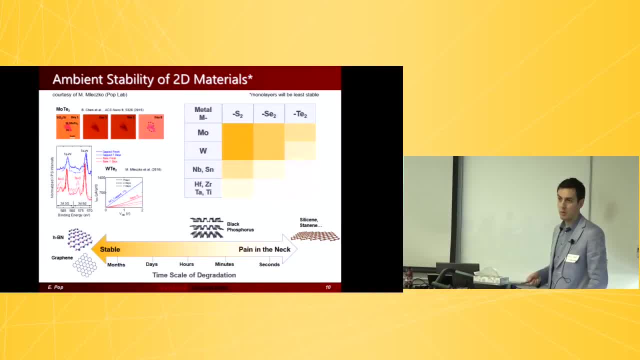 If you cap it with aluminum oxide, it seems to be stable, At least for a week. So aluminum oxide, we found, if you work in a glove box and then you immediately cap it with aluminum oxide, it seems to actually be, you know, relatively stable. 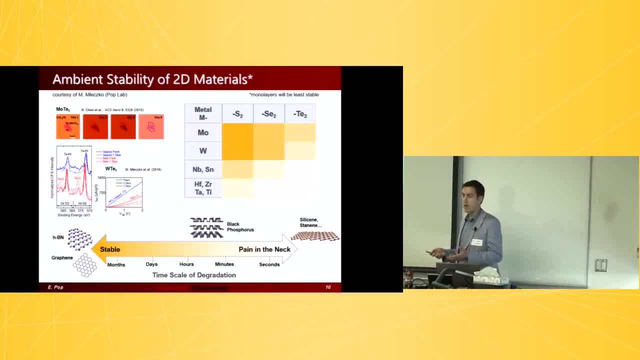 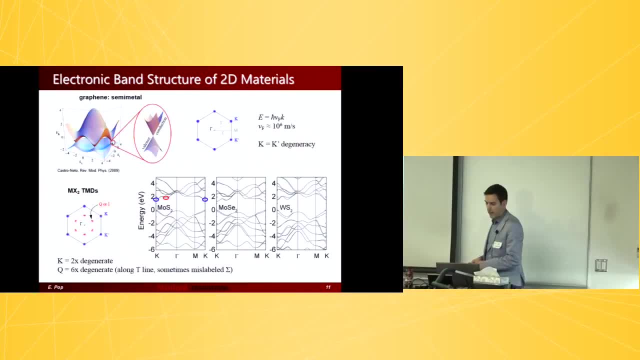 So then it actually enables you to do something with it. But otherwise tungsten telluride is basically, it's quite difficult- Tungsten tellurium, you can see, would be quite difficult to work with. Okay, Just a couple of words about electronic band structure. 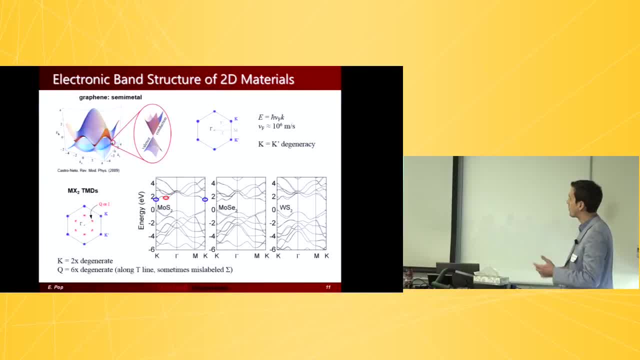 My talk is really more about phonons than electrons anyway. But a couple of words on electronic band structure. I'm sure you're familiar with the one in graphene, the KNK prime degeneracy. The KNK prime degeneracy, The nice beautiful linear bands, at least around the tips of the Dirac cones. 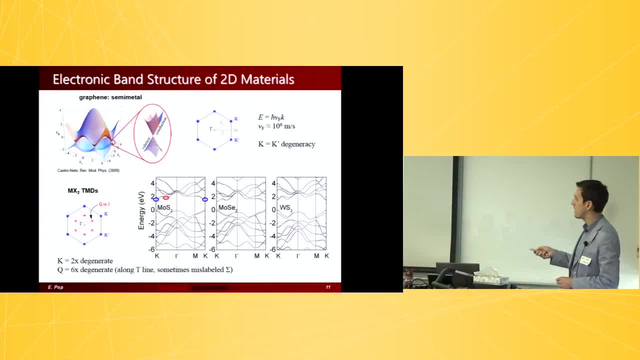 And then these are the energy bands in the MX2, transitional metal dichalcogenides. And the K bands are 2X degenerate. The Q valley, I'm sorry, is 6X degenerate. I should say K valley and the Q valley is 6X degenerate. 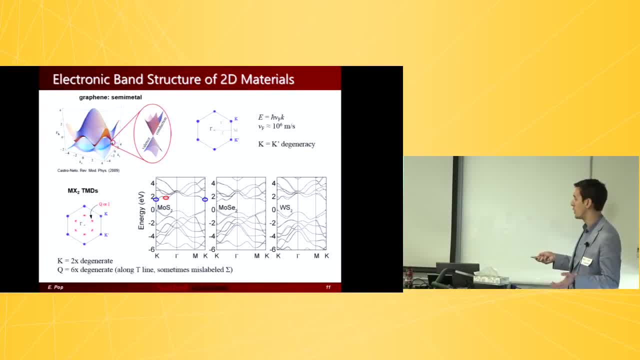 The Q valley. sometimes people call this Q. I've seen it mislabeled sigma. I think that's actually an error. I would say it's basically: this is what's along the T line Inside the Brillouin zone of the TMDs. 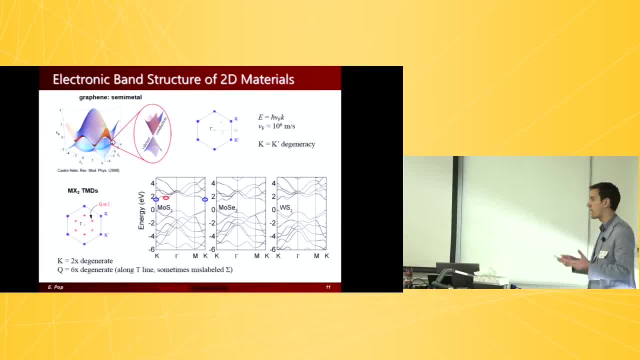 I've also seen it labeled as I actually, And I'm actually not sure why some people call it Q, Some people call it I, But I'm pretty confident sigma is actually not correct Because sigma comes from a different type of Brillouin zone arrangement. 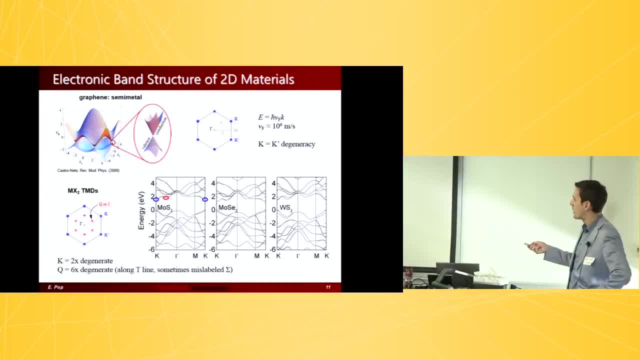 Some of the questions that remain kind of open are: what are these energy valley spacings, for instance- And that's why I highlighted these things- For different materials, different layers and so on? What is their dependence on strain, in fact? 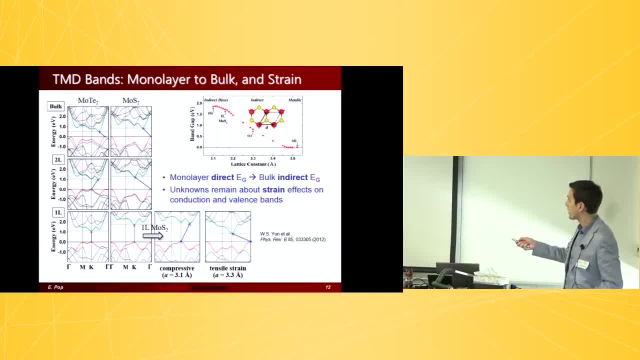 This is some other nice computational work. Here, for instance, is molybdenum telluride, Here's molybdenum sulfide. You can see that as you go to monolayer, and I think you all know this. 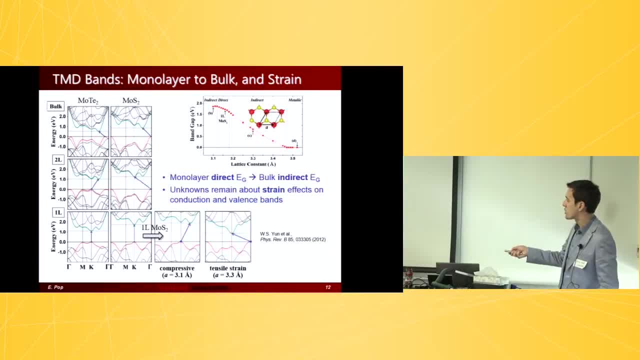 As you go to monolayer the bands are direct. But then if you take these direct band gaps and then you strain them- This is compressive strain, This is tensile strain- You essentially have different shifting of the K and Q valleys. 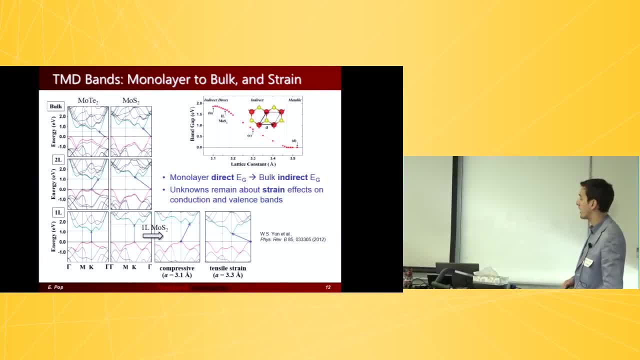 And you can end up again with the indirect band gap In monolayer materials. And so, like I said, some of the unknowns that remain as far as I'm concerned in these materials Are the strain effects on the conduction and valence bands. 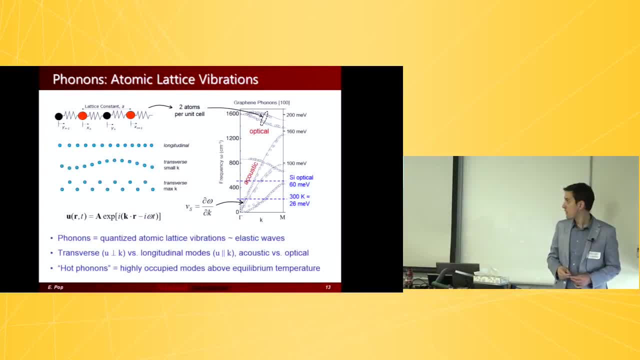 Phonons. Phonons are the lattice vibrations Right, And you have sort of there's a cute cartoon here of what these things essentially look like. These are the atomic motions, right Waves and so on. We have longitudinal phonons which are essentially these compressive waves. 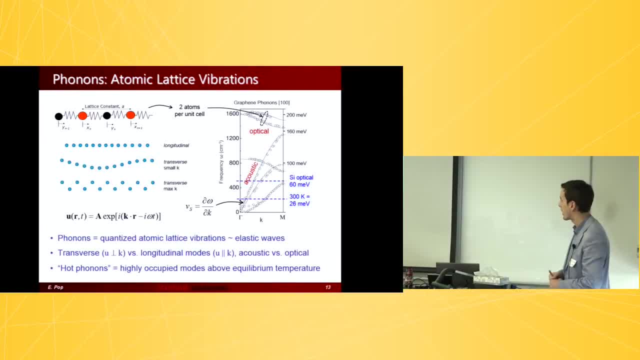 And then you have transverse phonons, Which are these shear waves essentially Right Here on the right I'm showing the phonon dispersion of graphene. Right, These are the acoustic modes Which essentially carry the heat in the lattice. 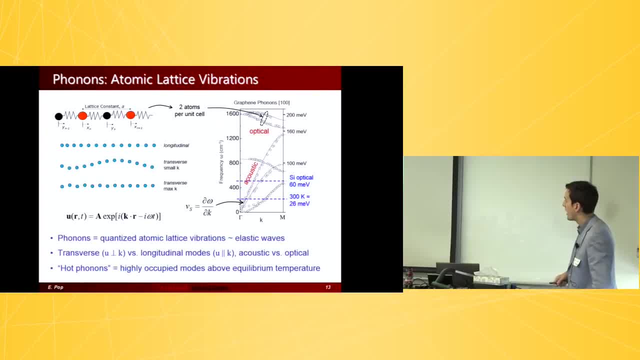 And these are the optical modes Which, as you can imagine by their name, interact fairly strongly with light, Largely because of their large density of states here at zero K vector, So around the gamma point, This is actually what you pick up as the G mode in graphene. 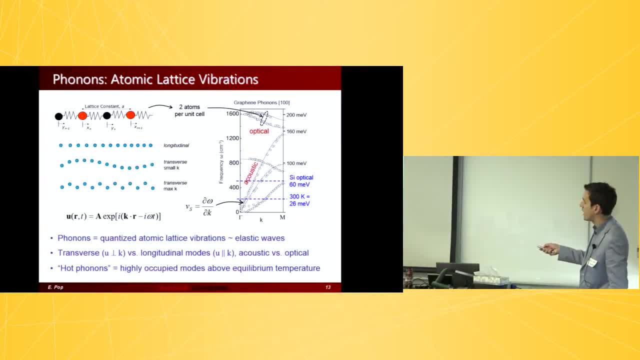 The slope of the bands. right here This is important- Is the sound velocity in the material. So no wonder graphene has very, very large thermal conductivity, Because essentially the slope of the acoustic phonons, Or the velocity of acoustic phonons In graphene is extremely large. 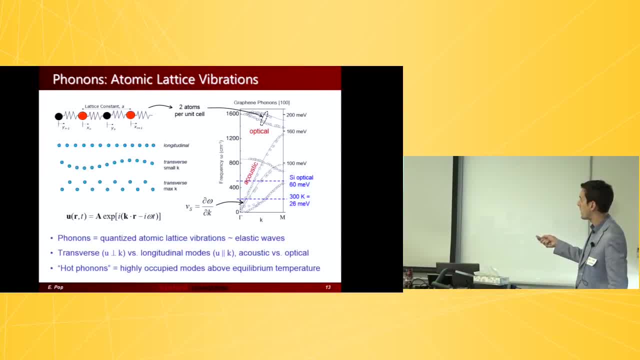 And just for comparison. I can't really overlay two dispersion relations Because it's going to look like a mess. But for comparison, The optical phonons in graphene are over here. The silicon optical phonons will be down here somewhere, So you can imagine the silicon bands will actually have significantly lower slope. 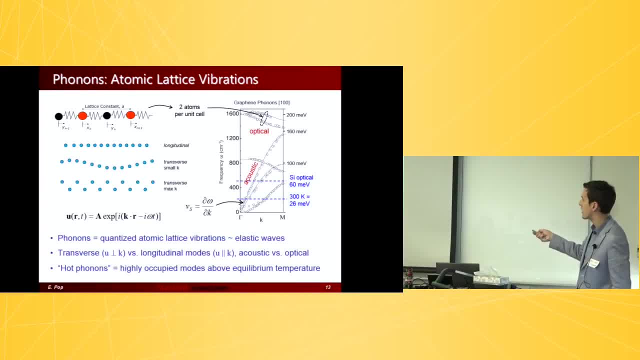 And also So you can see where 26 MeV is on this. It's roughly around down here, So that kind of gives you an idea of which phonons are conducting at the most at room temperature, If you can say something like that about bosons, of course. 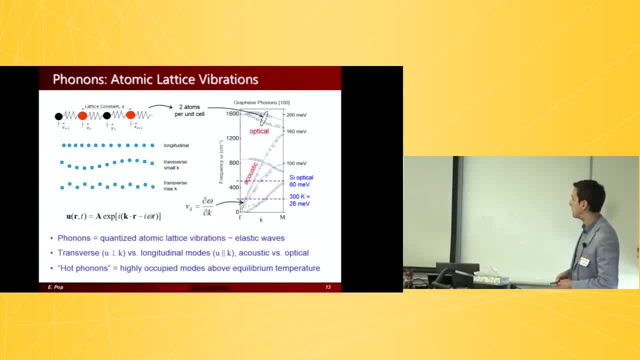 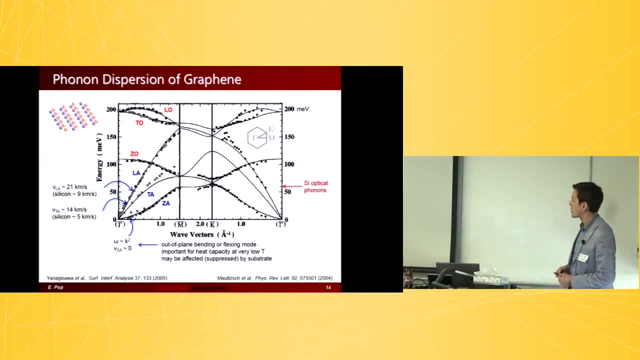 It's not really like a Fermi level, But it kind of gives you an idea. Okay, So, having said that, Here's a slightly deeper look at the phonon dispersion in graphene. As I mentioned earlier, The phonon velocities for phonons are actually quite large. 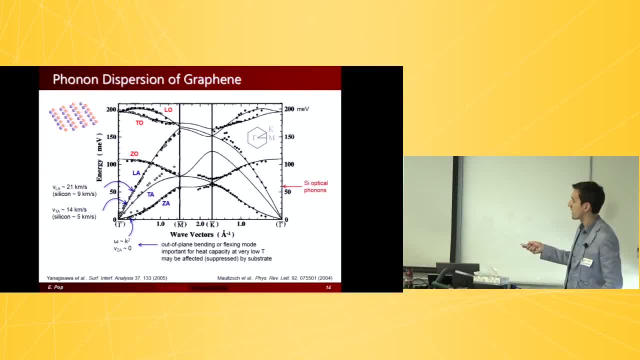 The longitudinal acoustic modes about 21 kilometers per second. In silicon that's 9.. The transverse acoustic modes 14 versus 5. So about a factor of 3. Larger phonon velocities than in silicon. What is unusual about 2D materials? 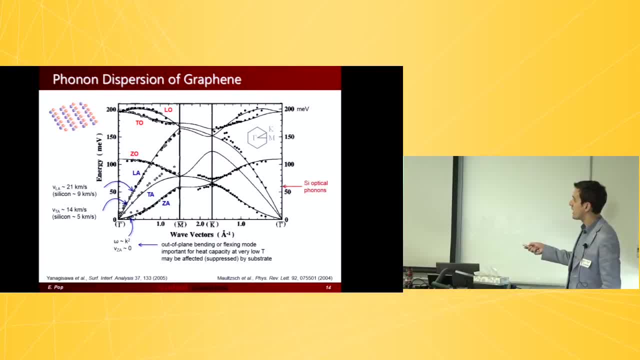 And you actually do not see this in 3D materials- Are the ZA and ZO modes, And so these are the out of plane bending or flexing modes Which, as I'll show in a moment, Are actually quite important for heat capacity. 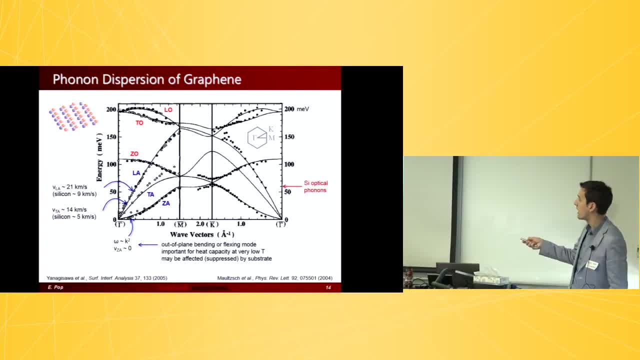 Right. So the density of states in these things is actually quite high, Both in the ZA as well as the ZO modes, And the ZA mode actually has an effect on thermal conductivity as well. This wasn't originally recognized for graphene. 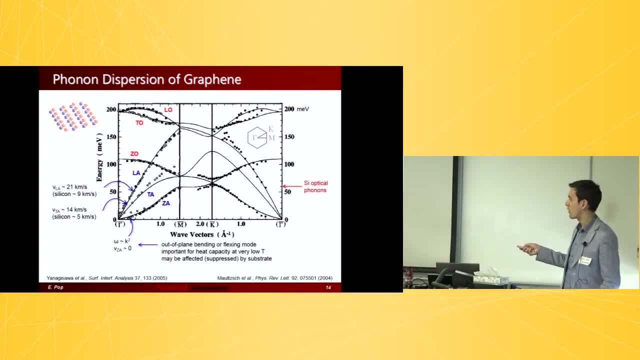 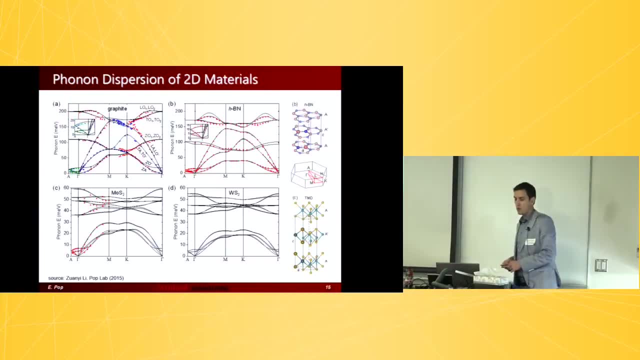 But it does have an effect on thermal conductivity as well, Because these are very highly occupied modes At relatively modest temperatures. Here's the phonon dispersion of other 2D materials. Again, it's very difficult for me to show these sort of side by side. 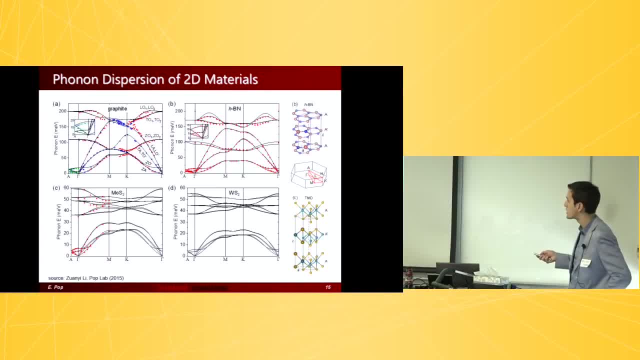 But I tried my best. I know this looks a little bit. This is probably one of my messier slides. So there again, that's graphite. You see the transverse modes, I'm sorry, The Z. Well, the flexural modes. 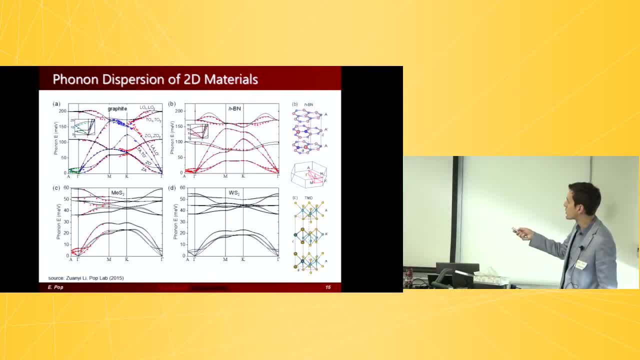 ZA and ZO and so on. Here's boron nitride. Notice that the vertical scale is about the same. It deliberately shows the same. This is 200 MeV, That's 200 MeV. So boron nitride has. 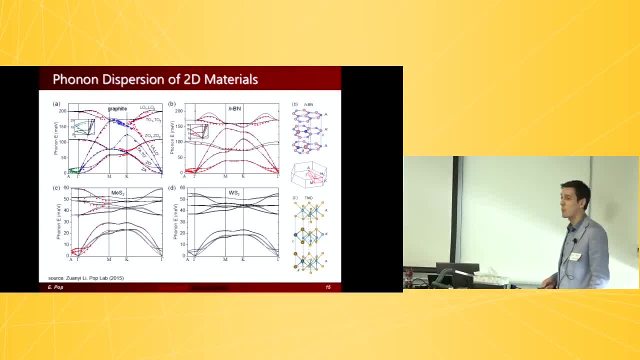 It's probably the only other material that has phonon modes that keep up with graphene Or graphite, Right. So again, you automatically expect boron nitride to have very good thermal properties Just by looking at the phonon dispersion, Right. The one other thing I want to point out, by the way, is this gamma to A thing that shows up. 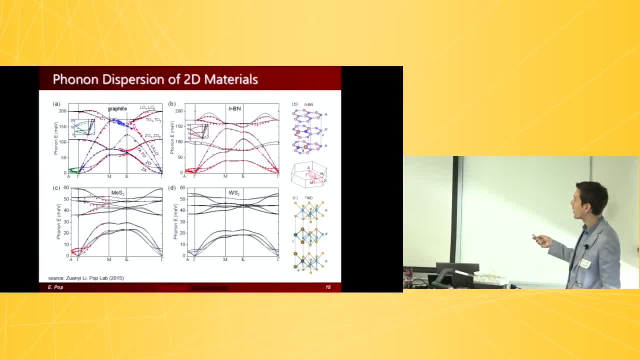 Gamma to A is the out of plane component of phonon dispersion Right, Look how small those phonon modes are. So A- those are fully occupied at room temperature And B- they have incredibly slow sound velocities. Right, Which means again, just intuitively looking at this. 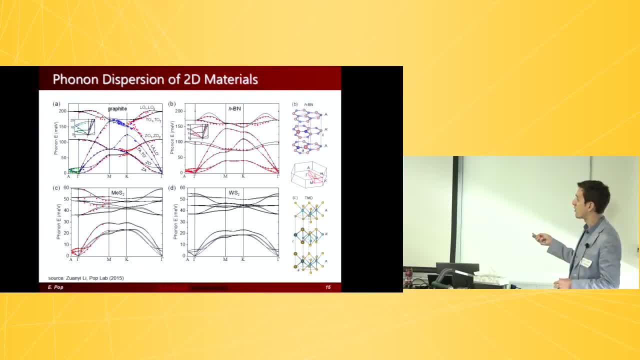 Means that the out of plane thermal conductivity component of these layered materials is going to be tiny, Right? So you can kind of already imagine That These materials are thermally very anisotropic, And I'll show you some numbers for those a little bit later on. 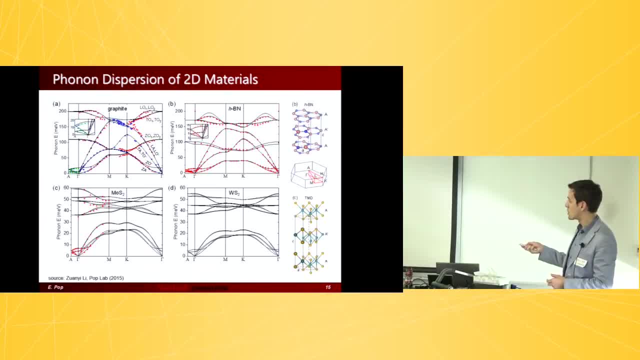 Here's MOS2.. This is the phonon dispersion MOS2 calculated as well as measured. Again, you see the out of plane phonons. Same thing: Gamma to A Very, very small group velocities, All thermally occupied at room temperature. 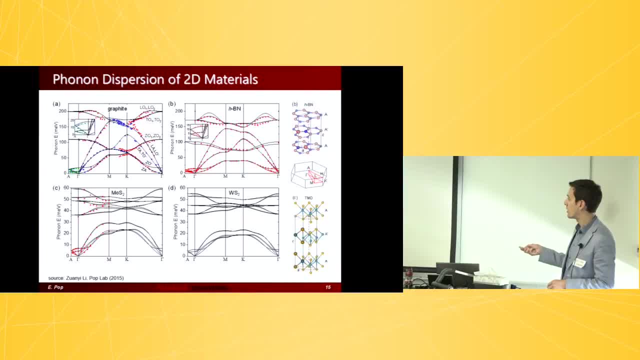 Tungsten disulfide. We could not find experimental data, But we do have calculations from one of our collaborators So you can kind of see graph. Of course graphite's been a lot more studied And then sort of This is a little bit less so from the point of view of phonons. 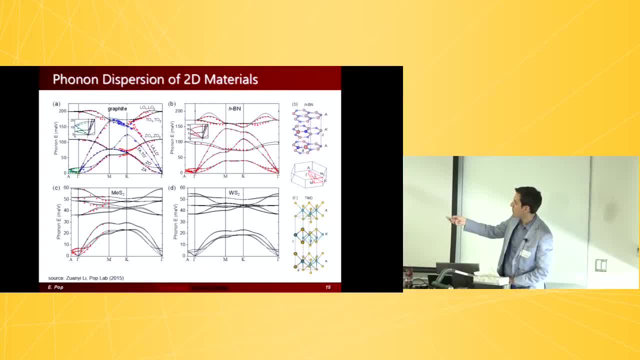 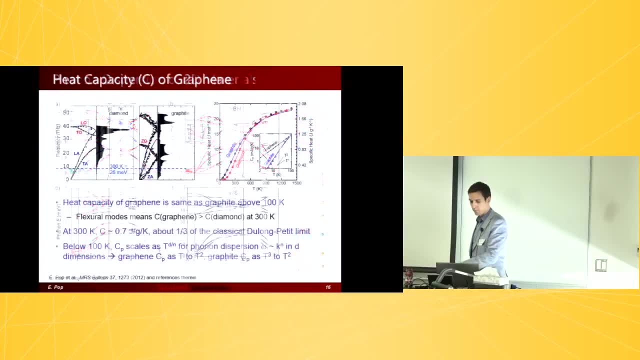 But notice the vertical axis: 60 MeV. 60 MeV, These are 200.. Right, So these are going to have significantly lower phonon energies. The heavier materials, of course. I want to say just one word about heat capacity. 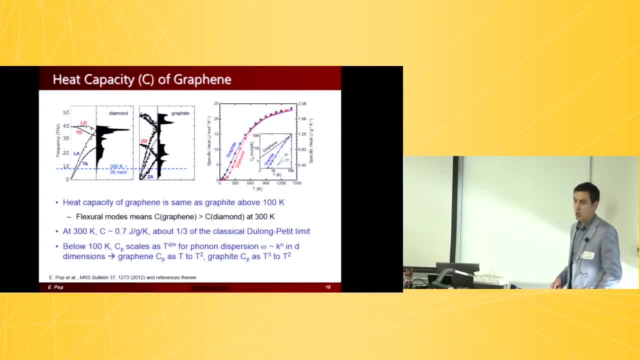 Heat capacity is basically? Well, it's basically the ability to store heat, Right, It's the energy per degree Kelvin, per unit I guess, per unit mole, if you will, Or per gram, Or per cubic centimeter, Depending which units you prefer. 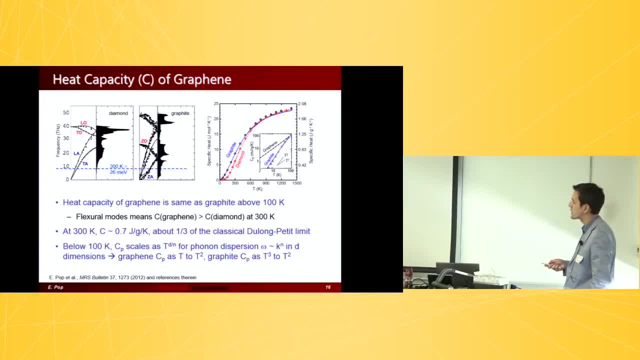 This is where the ZA modes are a little bit interesting. Look, for example, diamond And graphite, Right. So here's the density of state, Here's the phonon dispersion For diamond And here's the phonon dispersion for graphite. 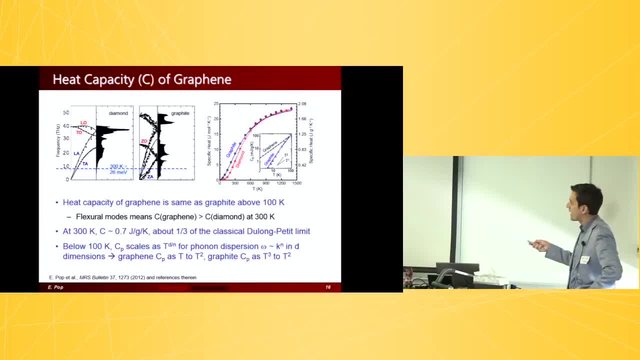 And the corresponding density of states. You will see that in graphite, At the same temperature as in diamond, You actually have significantly larger density of states Than in diamond. That's because of the flexural ZA modes Right there, Which are these bendy modes? 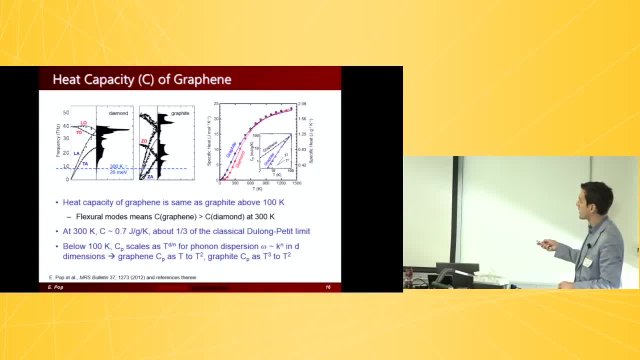 With a quadratic phonon dispersion And so If you actually look at the specific heat For graphite and for diamond At room temperature, The specific heat in graphene is about 30% higher, Or graphene or graphite Is 30% higher than in diamond. 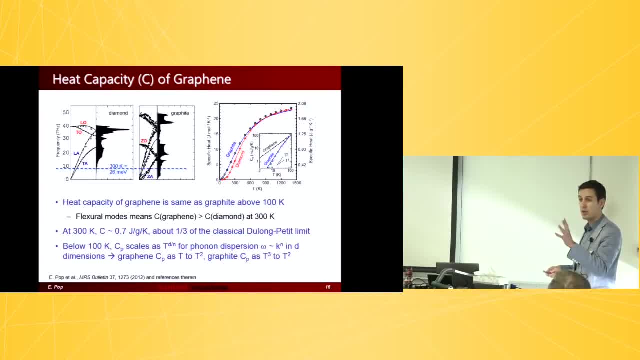 And then eventually they converge Only at temperatures about Above about 1000 degrees Kelvin. At really low temperature There's actually very subtle differences Between graphene and graphite Heat capacity, But these are below Temperatures, below about 100 degrees Kelvin. 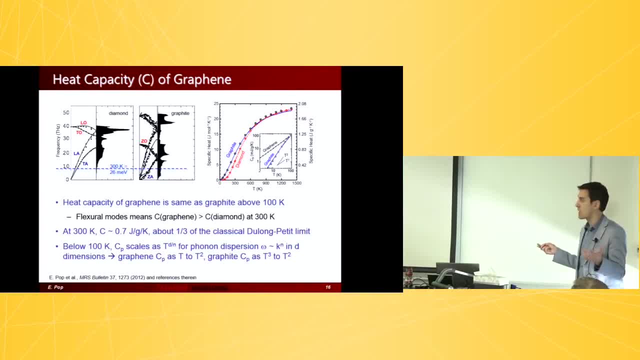 And so at room temperature, Graphene and graphite Essentially have the same heat capacity. At lower temperatures There's these subtle dispersion differences Because in graphene You actually have a slightly more free Out of plane flexural modes, Whereas graphite. 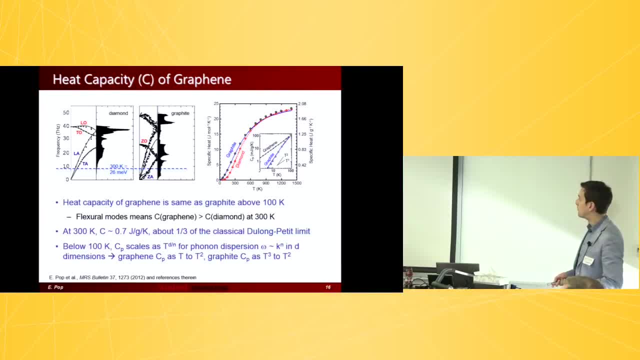 They're a little bit more confined, As you might imagine. Right, What else should I say, The? There's an interesting rule of thumb In the phonon world Which you can look up, For example, In the solid state physics books. 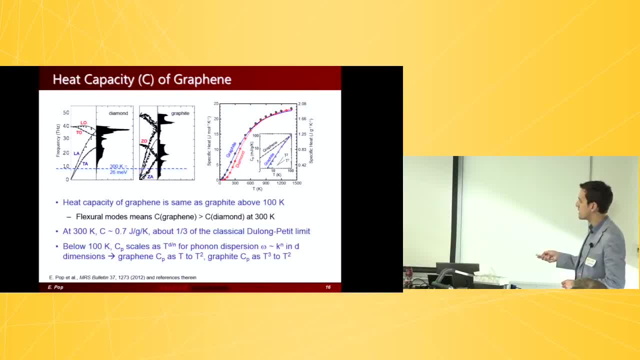 Like it tells, The heat capacity tends to scale As T to the power D over N, And this is for a phonon dispersion Omega Going as K to the power N In D dimensions. That's what this, This funny term, means. 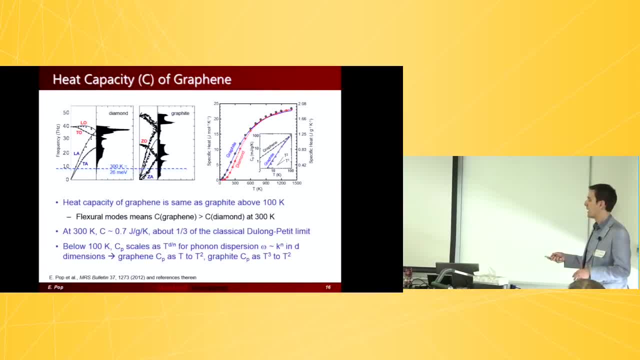 Right. So, for instance, You know, In silicon This would be a linear dispersion And it's 3D, So it would be T to the power, 3. Right, But in graphene And graphite You actually have some funny. 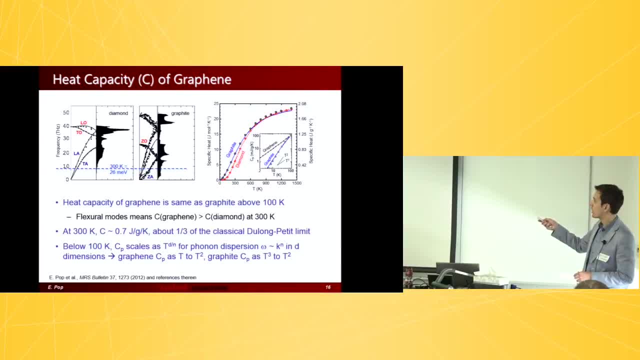 Exponent terms And, like I said, You really only notice those At really really low temperature. At sufficiently high temperature, All the The heat capacity Is essentially Approach What is known As the classical DeLong-Petit limit. 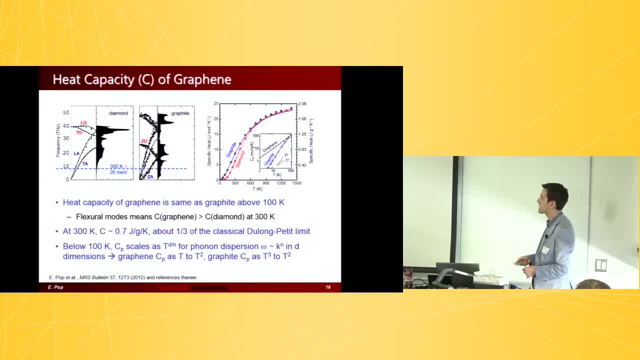 Of course Graphene And diamond Really become classical Only at temperatures About, About Above About A thousand degrees Kelvin. Okay, That was supposed to be circled there, But That was the same thing, Doesn't matter. 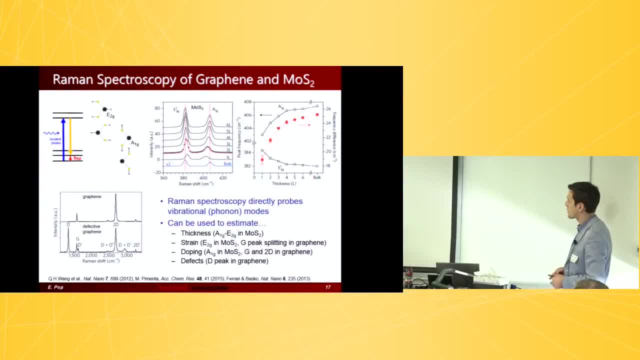 Or I already said it, Raman spectroscopy. So Raman spectroscopy Is something that, Obviously, I don't have much time To talk about, But It is something That we use quite frequently- Not just us Quite often. 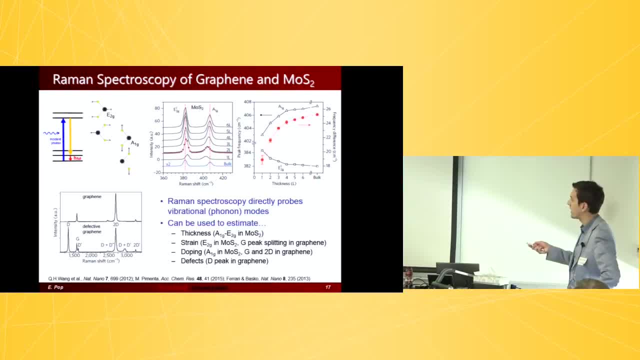 Because It allows us to probe The phonon modes Directly In a way, And I think Professor Zhu Already showed this. You have these In plane modes, Labeled the E modes, And you have the out of plane modes. 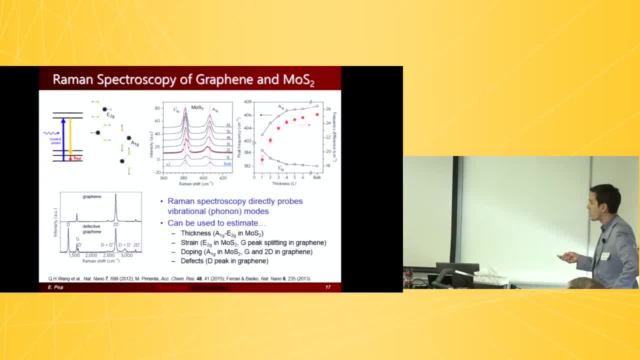 Labeled the A modes In some of these TMDs, And There's a lot of. There's really a wealth Of information That can be gained from this, And here's some of my favorite reviews, Which I: 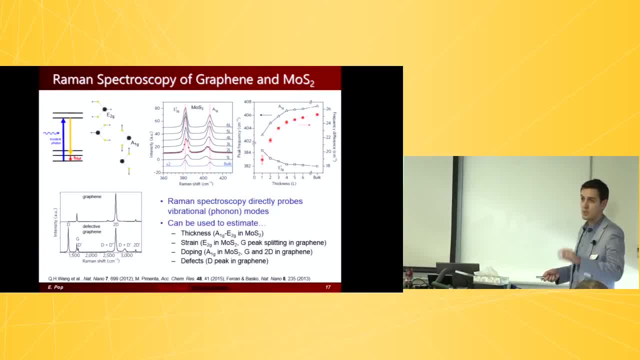 I just listed at the bottom Of the slides For your convenience. But we can estimate, For example, The thickness Of the Dents. So MAOS2.. But you can see. You can see, I have subtle differences. 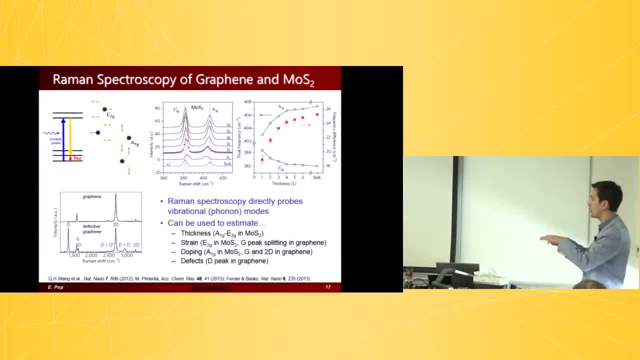 That basically Allow us to map This Through a number Of layers. We can, For instance, Study strain Right. So the E mode In plane mode And MAOS2. Is sensitive to strain, As you might imagine. 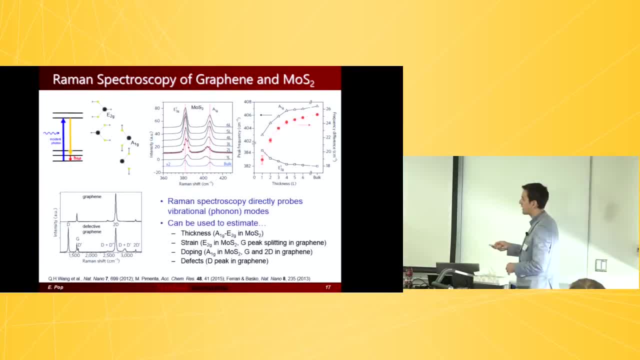 And also The G peak Becomes split In graphene, Also due to strain Doping. The out of plane mode Is sensitive To doping And MAOS2.. And unfortunately for us, there isn't, to my knowledge, an equivalent mode in MOS2.. 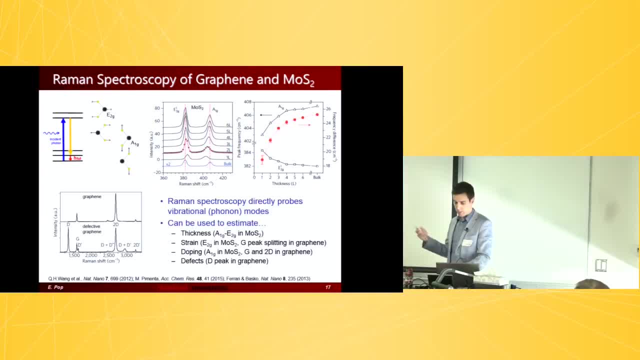 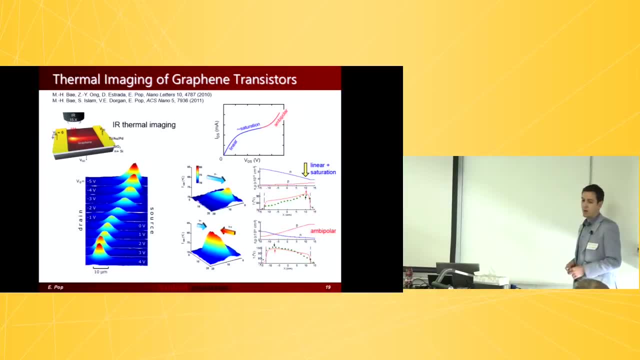 So it's not as easy to map out your defects by Raman in MOS2.. Photoluminescence perhaps, but not Raman. Okay, so a couple of words about where these thermal effects play a role in devices, And hopefully I can make some bridges with the presentation by Professor Zhu a little bit earlier today. 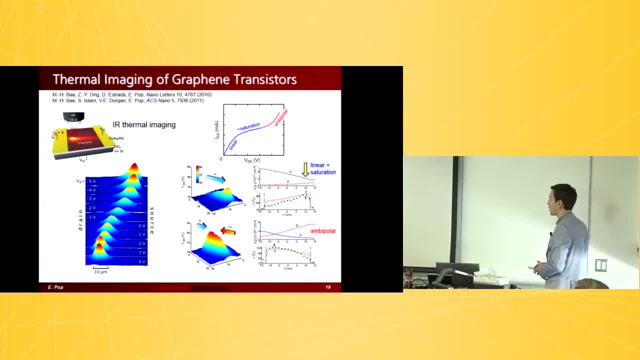 Okay, some work that we did a few years ago now- so almost five years ago now- actually was. we took some of our earliest graphene transistors and we stuck them underneath an infrared thermal microscope And, frankly, I'll be honest with you, I didn't expect to see anything. 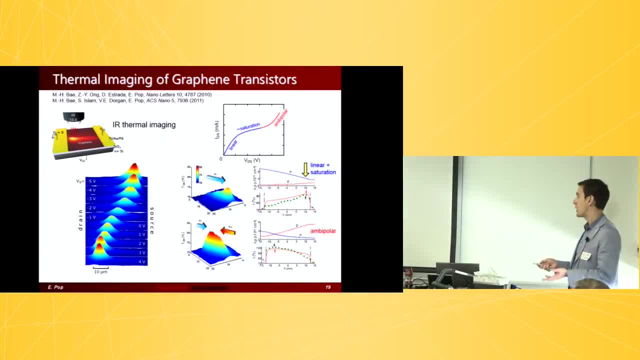 I said graphene's transparent, I'm not going to see anything, right. But we had an infrared thermal imager nearby and we said, well, let's just see if we see something. And amazingly we actually saw quite a bit of infrared thermal emission. 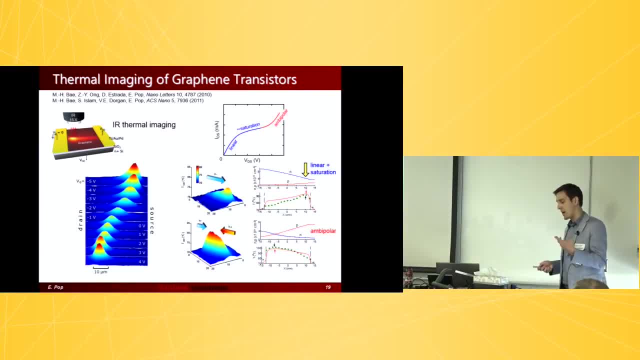 from the graphene. Later on we realized what was actually happening is: yes, graphene is transparent, mostly transparent to infrared, But actually what's happening is the graphene is heating up the silicon substrate underneath And we're actually imaging the heating of the silicon substrate, which is a you know. 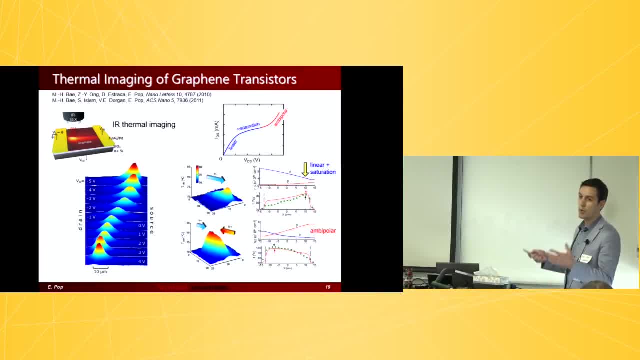 this is free care emission from the silicon substrate, which is heavily doped, But regardless, the point is you see a huge signature of heating And this is actually a hotspot that dances around the channel. If you go to our website, you can see a movie of this thing. 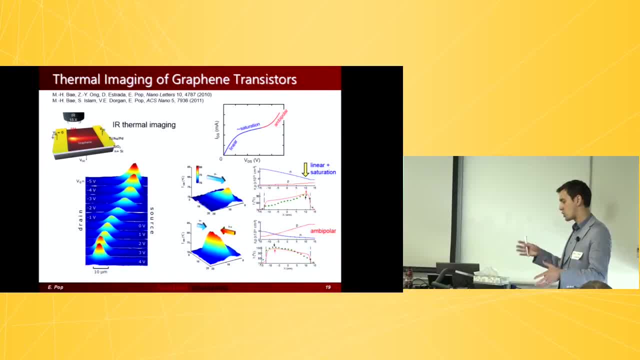 It dances around the channel, depending on the source, drain and gate voltage that you apply on these transistors. And so, just to kind of make a long story short, what we realized is that, you know, graphene transistors are ambipolar. 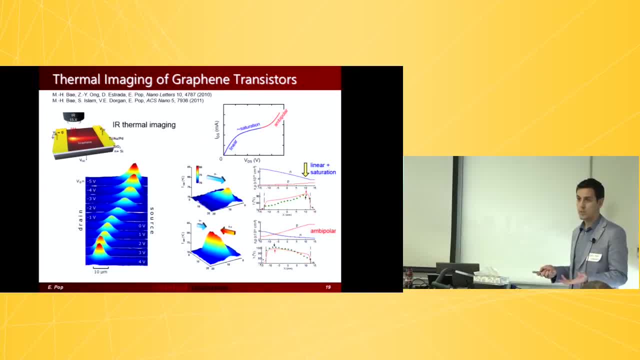 And so when you operate them as a unipolar transistor, the hotspot occurs near the source or near the drain, which is pretty much what you expect in like a conventional silicon or gallium arsenide or gallium nitride type transistor. You essentially get a slight carrier depletion near the drain. 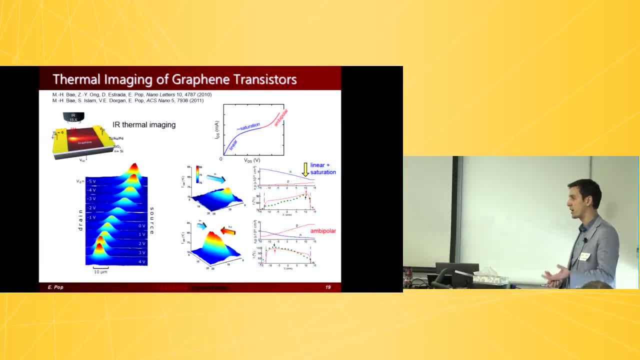 I wouldn't use the word pinch-off, because in graphene you never really get real pinch-off right because there's no band gap, But you get a slight carrier decrease right And so there's a hotspot that forms at the point of minimum carrier density, because that's where the maximum field is. 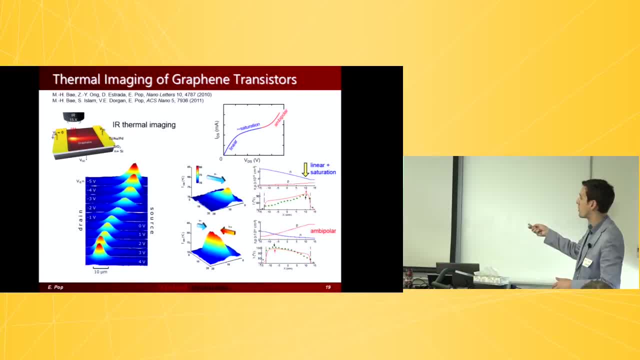 And so that roughly corresponds in the IV curves to the saturation regime. But this again looks very, very similar, if you're familiar with other 2D semiconductor, I'm sorry, with other semiconductors in general. Where graphene is a little bit bizarre is that you can actually inject electrons from one terminal. 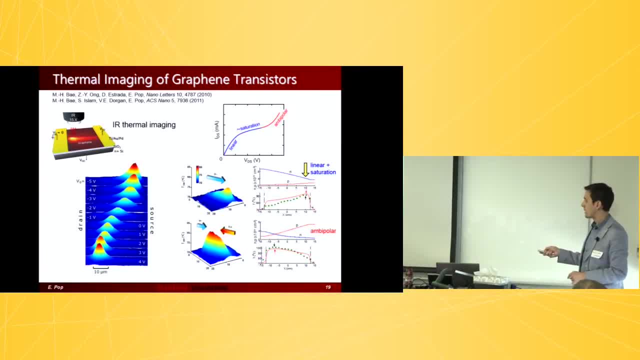 and holes from the other terminal. And so if you do that, it turns out the electron and hole carrier densities arrange themselves in an X. okay, And this can be calculated using fairly simple computer codes. And so if they form in an X, the electrons and holes, there's going to be a point of minimum carrier density that's actually in the middle of the channel. 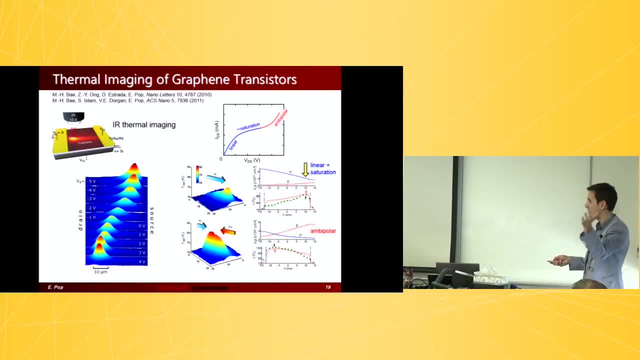 And that's going to be the point of the hottest, you know, highest electric field, hottest region and so on, And that's when the hotspot dances to the middle of the channel, And so we see, And so it's kind of a nice way to thermally observe the carrier densities inside the channel. 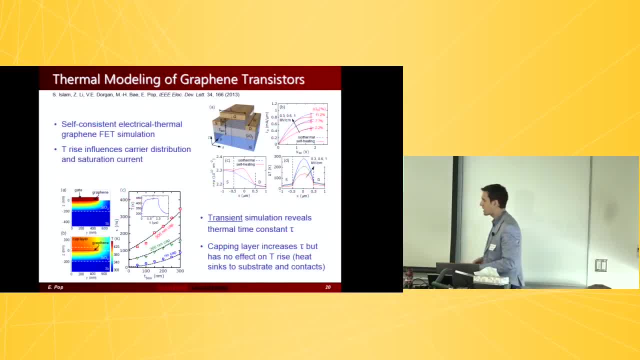 That's essentially what is happening over here. We actually put together a model, obviously for that work. That's how we were able to explain it. We took that model one step further a few years later. And we took it a step further because I really wanted to look with the model to device dimensions which we couldn't thermally image right. 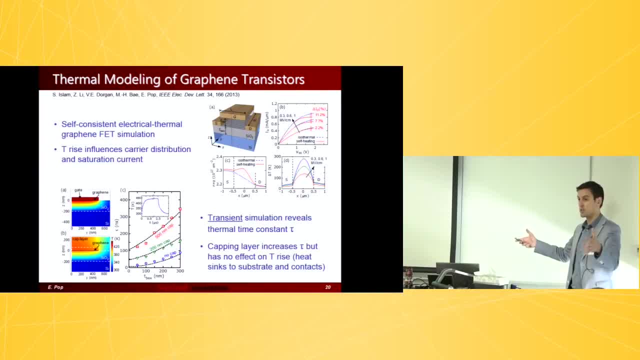 Imaging things with infrared You can only really do on really really large devices. Even with RAMA you really need micron-scale devices to see anything right. With the model you can study something submicron And you know. as long as the physics is right, probably what you're going to get is going to be pretty reasonable. 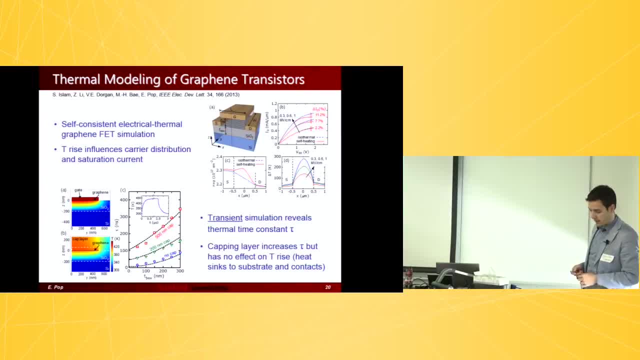 Anyway, one question that you know I frequently used to get when I was showing the previous slide was: you know well, if you put a gate on the device, like a top gate, isn't the top gate just going to suck away all the heat and therefore your device will no longer heat up? 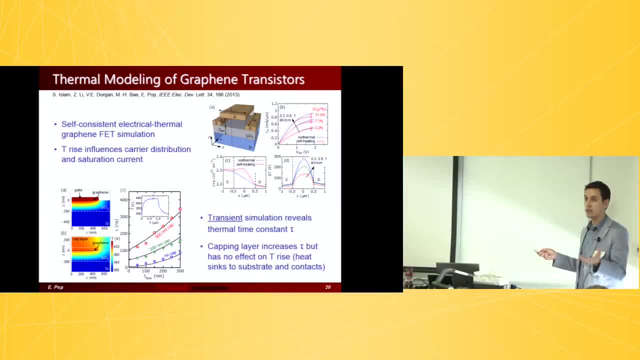 Or the other question that I would get, of course, is: doesn't graphene have a really high thermal conductivity and carry the heat to the contacts right? So this actually kind of set out to answer both of those. If you have a gate on top, what happens is the gate is really not a really good heat sink actually. 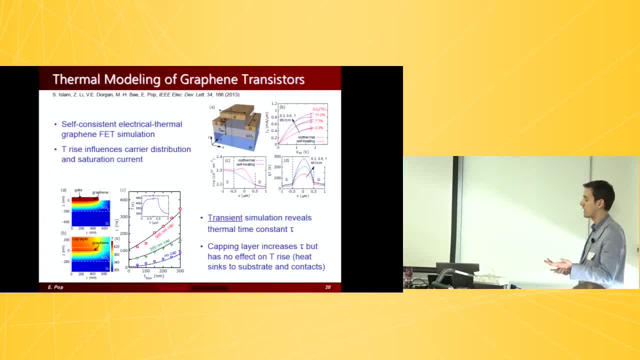 It turns out, the heat still goes to the substrate, The gate itself. you can think of the gate as the egg sitting on the pan. you know that well. earlier it was an egg on a computer processor, But you can imagine an egg on a pan right. 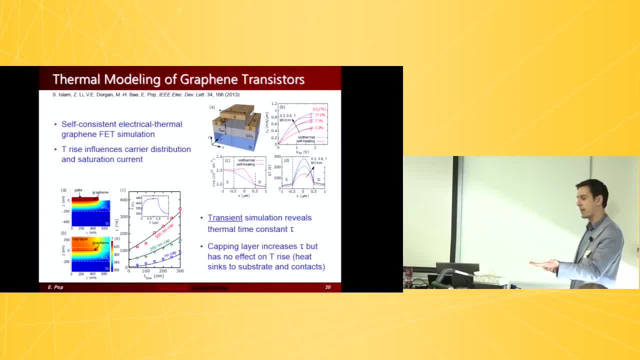 You put a pan on the stove, You put an egg in it, right, The pan heats up. It heats up the egg to the same temperature, right, But the egg itself is not actually a heat sink, right? However, what the egg does do, or whatever's in the pan, you know your favorite. you know pasta dish or something like that. 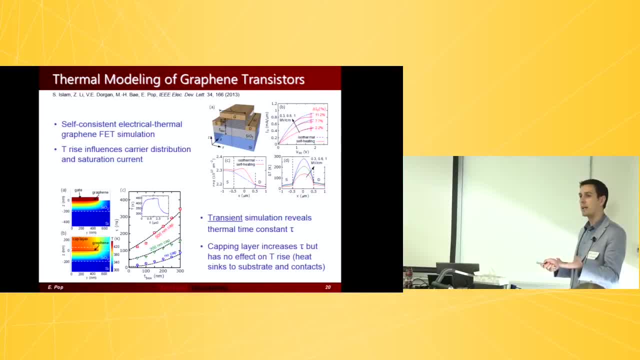 what it does do is it actually slows down the rate at which the pan heats up. So there's actually a thermal capacitance component that the gate actually brings in. Not only the gate, but also, if you have this encapsulated in some sort of a capping layer like you might have inside a real transistor. 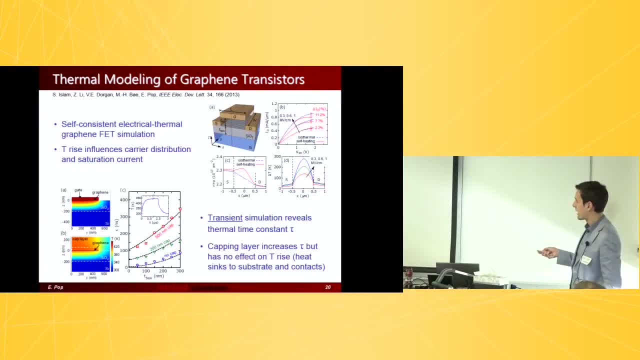 So what we realize? What we realize is that the gate and the capping layers actually affect the transient, not the ultimate temperature of the device for a given power density, but the transient- how the device actually gets there. So we did these transient simulations. 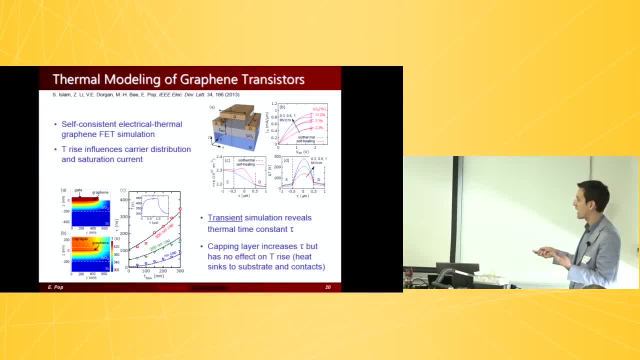 You know, the devices have, you know, fairly fast thermal transients if they're not capped. But if you put a cap and a gate and so on, then the thermal transients actually slow down quite a bit to the order of you know, hundreds of nanoseconds. 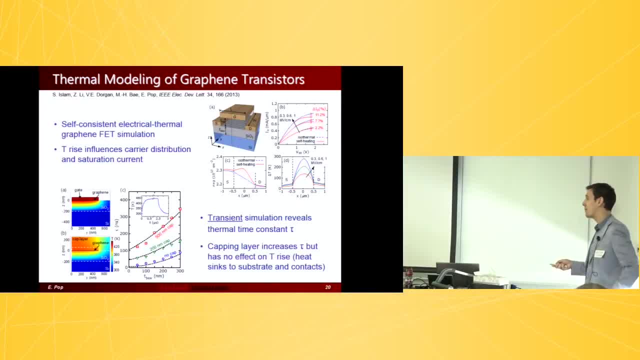 Otherwise they could be tens of nanoseconds or something like that. And, by the way, the graphene itself has such a small heat capacity In this case, because it's a monolayer- that really, even for an uncapped device, most of the heat capacity is the one in the substrate. 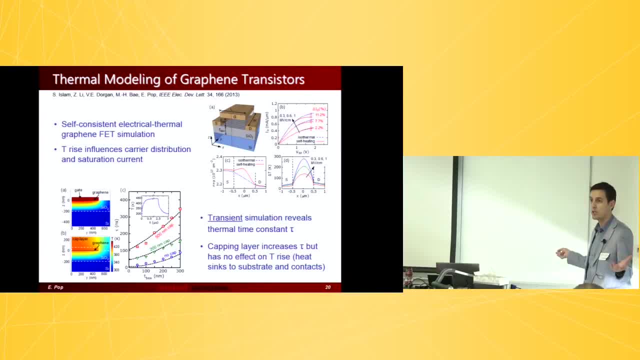 It's the SiO2 and the silicon substrate that actually takes some time to heat up. Otherwise, the graphene itself would heat up in less than a nanosecond, So it'd be almost instantaneous. To answer the heat dissipation to the contacts part, I guess I don't have a good. it's not really shown over here. but essentially what we found out is that, yes, you can get significant heat sinking to the contacts. 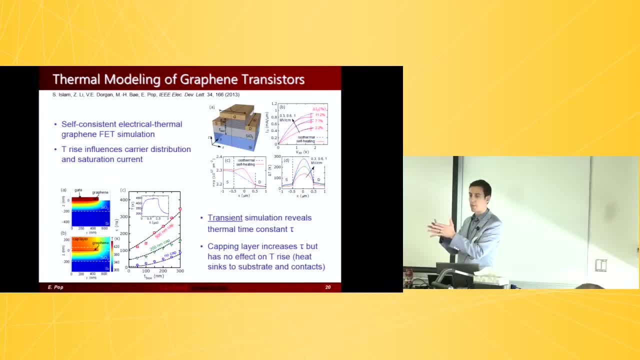 But only in devices that are shorter than about half a micron. For any device longer than about half a micron, most of the heat actually goes into the substrate. For short channel devices, of course, the contacts do play a significant dissipation role. 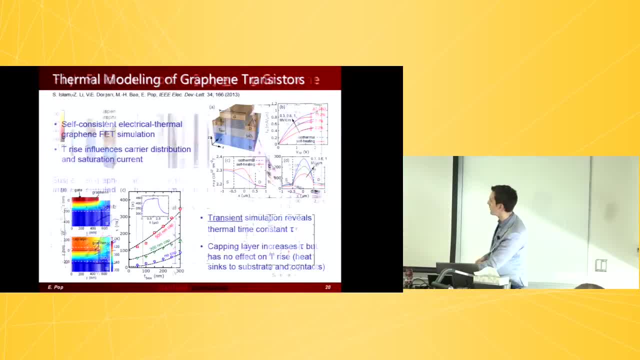 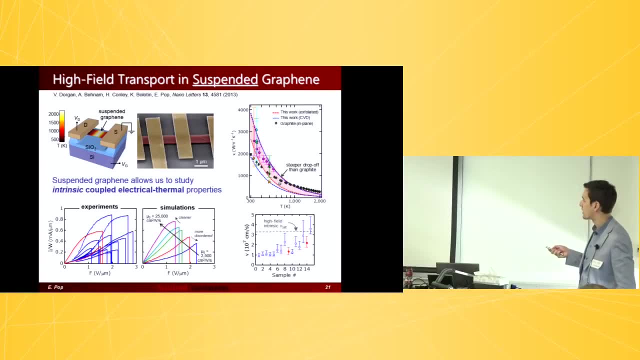 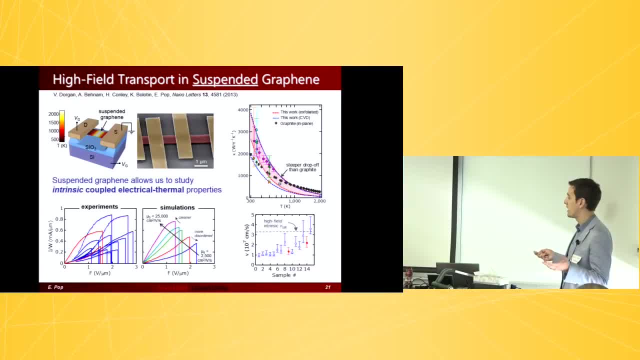 kind of as an extreme case, because by getting rid of the substrate we said: look, this is going to allow us to study the intrinsically coupled electrical thermal properties. Right now, the heat cannot go into the substrate, now it really can only go to the contacts. We have a simulator. great, let's compare. 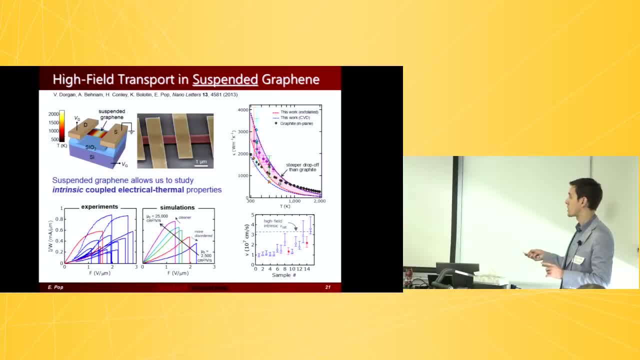 experimental data for high field transport with simulations for high field transport, and what we realize is that, essentially, comparing, going back and forth between these two, we could actually fit the thermal conductivity of the device of the graphene, because heat can only go laterally. so in this case, 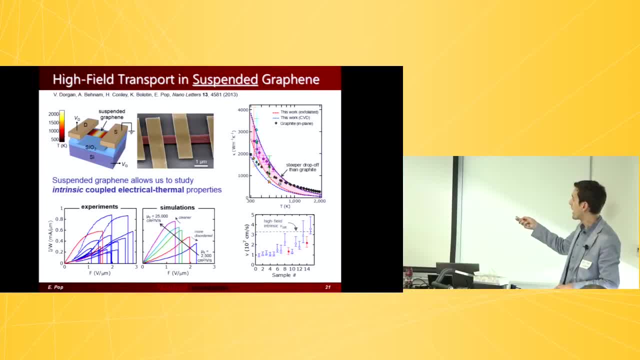 you're really forced to heat sink to the contacts and we can actually fit the thermal conductivity of device all the way from about room temperature all the way to the breakdown temperature of these graphene devices, which we estimate to be about 2,000 degrees Kelvin. By the way, this was all done in vacuum of 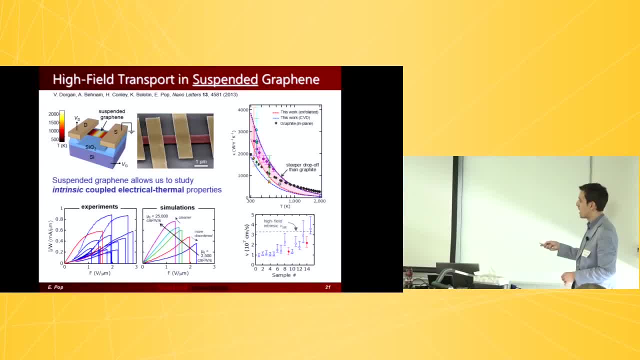 course We could also fit for various devices. what we thought was the high field drift velocity- and it was something approaching on the order of 3 times 10, to the 7 centimeters per second which is predicted, was predicted to be the intrinsic sort of maximum. 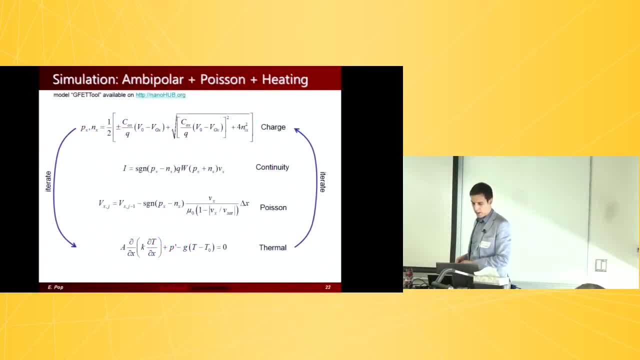 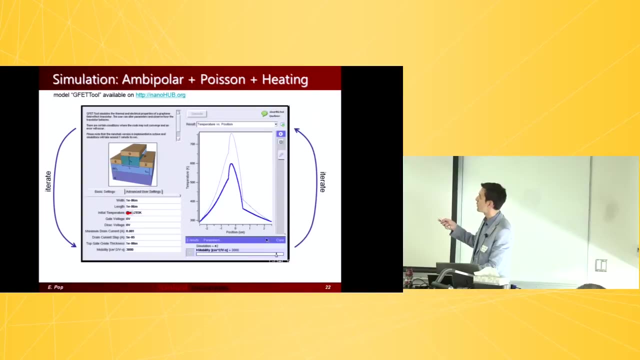 velocity you would get. Okay, I mentioned this model. I don't want to say too much about it, except that it's an iterative solution of the charge continuity Poisson and, of course, the thermal equations. This model is actually available on the nanoHUB right now. It's called, you know, GFET tool, graphene FET tool. so if you 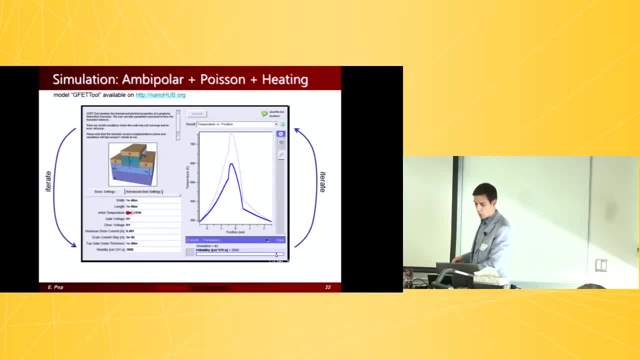 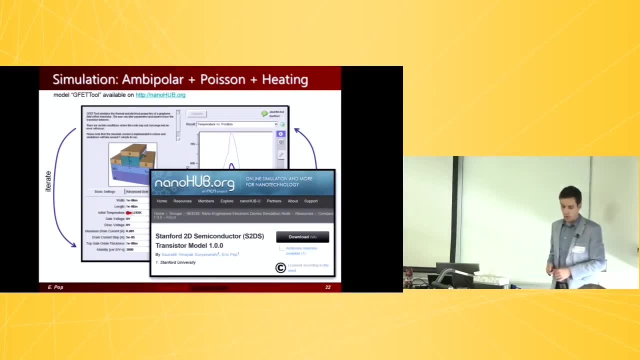 really find this useful, or if you simply don't like the rest of the talk, you're welcome to try it out right now and let me know how it works. More recently, we've also released a a slightly more compact model called the Stanford 2D Semiconductor Model S2DS. 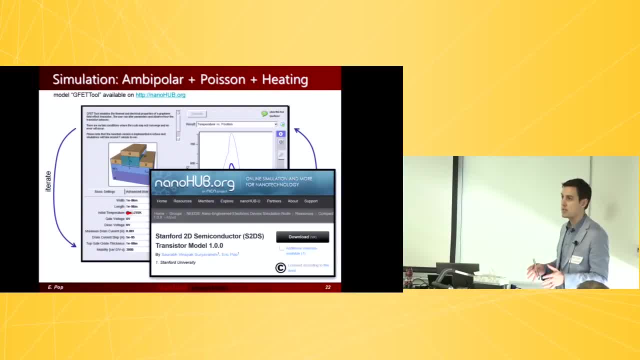 This is actually based. this is actually specifically aimed at TMDs, right? So this is: this is obviously for graphene simulation, This is for TMD two-dimensional semiconductor simulation. They're both available on the nanoHUB. This one, you can run directly in the nanoHUB. 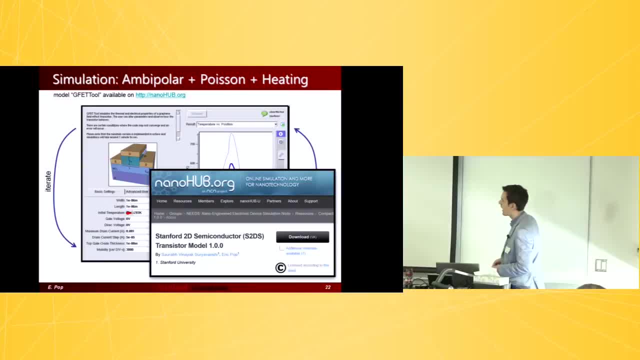 The other one you have to download and essentially it's written in Verilog A, But you can. this is a little bit more amenable for circuit simulations and that's what we're using it for right now. They're both electrothermally coupled and so on. 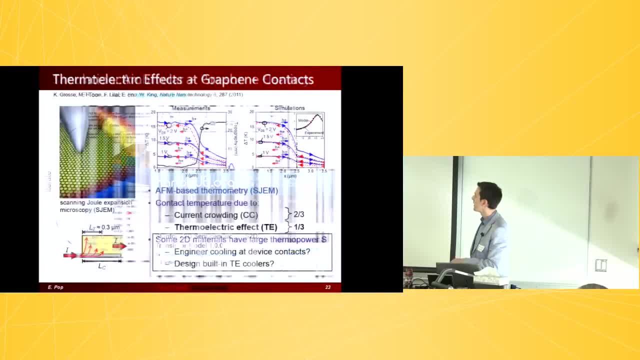 And of course you can tweak a lot of the parameters by hand. Okay, A little bit more on the on the thermometry side. You know we were not very happy with the infrared thermal imaging because the resolution is so poor, right. 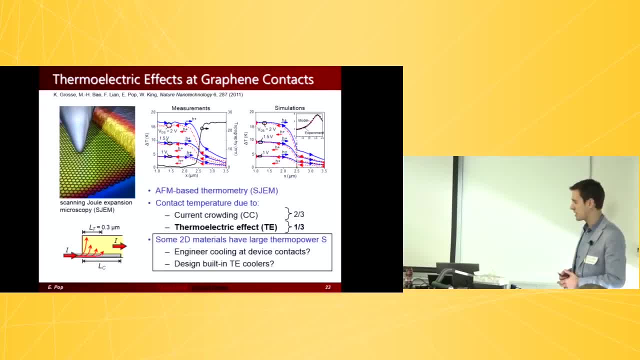 It's microns. It's about a micron or two Raman spectroscopy- same thing, about half a micron maybe. So we we worked with Professor Bill King at UIUC several years ago and we used an AFM-based method to measure temperature. 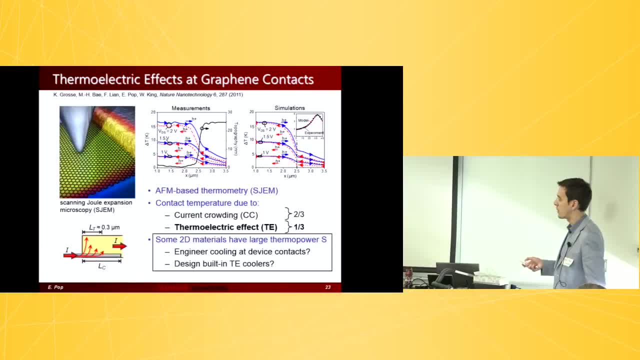 In this case, we essentially used an AFM tip to measure the thermomechanical expansion of the material itself In this case. I know this picture is a little misleading. This was done by an artist. Please forgive this picture. It's a cool picture, but it's actually misleading because the device itself 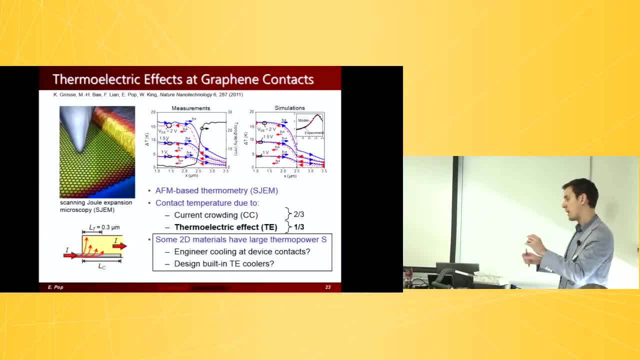 is covered by a layer of PMMA. So the thin layer of PMMA essentially acts as a, as a- you know, thermomechanical, you know- expansion layer. So as the graphene, or whatever this material is, heats up, the PMMA heats up and then the AFM picks up the thermal expansion of the 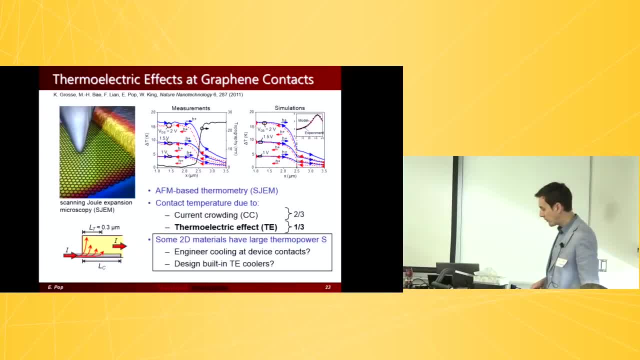 of the material, and then you convert that back to temperature. Long story short, we didn't see anything we didn't already know in the channel, So that was good. I guess The infrared imaging method actually showed us enough of that. But then we zoomed in on the contacts. 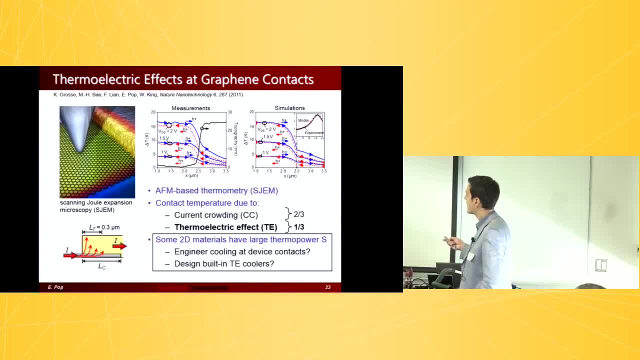 And when we zoomed in on the contacts we actually realized that we were seeing not only significant heating in the contacts, but we were also seeing cooling in the contacts if we were reversing the direction of current flow. So when the current flows into the contacts you get more heating. 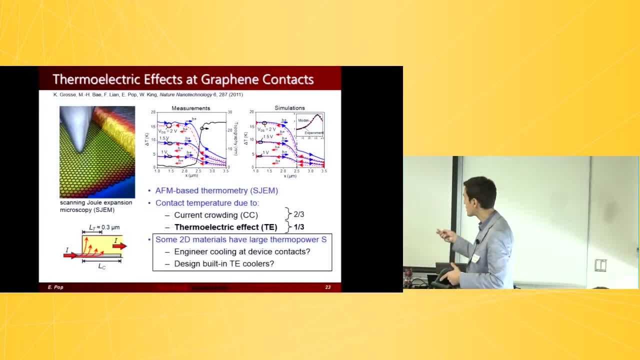 When the current flows out of the contact, you actually get less heating just right in the contact, And so this is actually. these are two effects happening inside the contacts. One of them is what you would expect, which is current crowding. 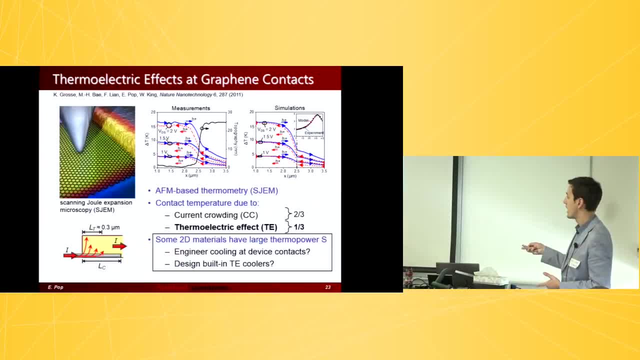 That controls about two-thirds of the temperature in the contacts. And then the other effect is a thermoelectric effect, which you know was actually really surprising. We saw it experimentally. Our models couldn't even explain it, But we saw it. and then, as soon as we put in the thermoelectric effects in graphene, 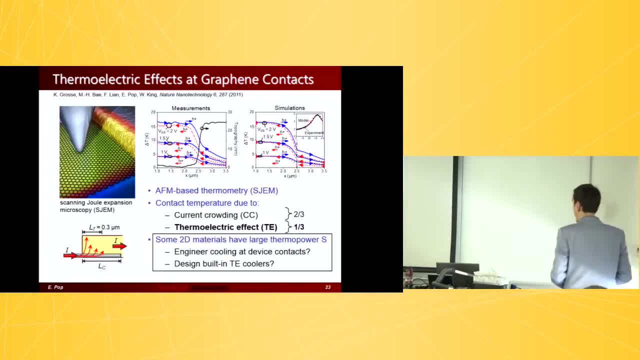 we actually got this and it worked. And what I find really fascinating is that, you know, graphene doesn't even have a very large thermoelectric power, as I'll show a little bit later, So this effect must actually be more pronounced in other 2D materials. 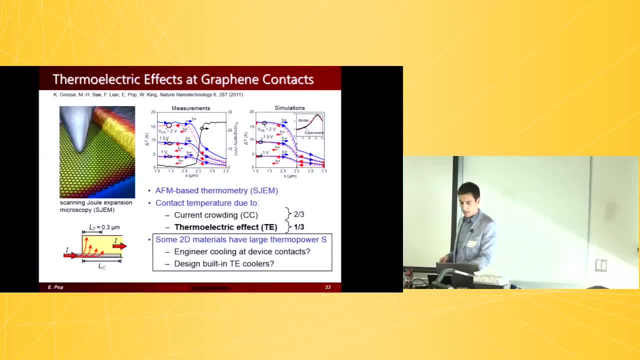 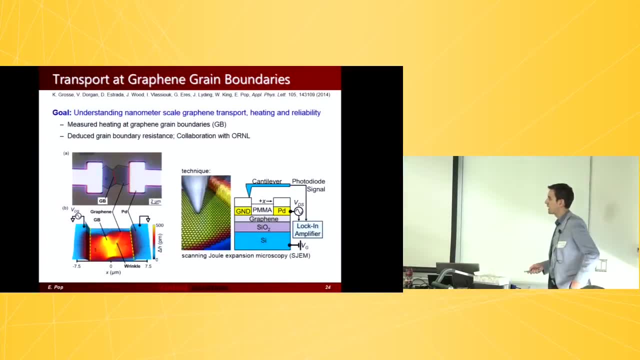 We haven't studied it yet, but it's perhaps something that we ought to do or you ought to do if you are interested. Okay, By the way, same you know, technique can also be applied to study heating at graphene-grain boundaries. 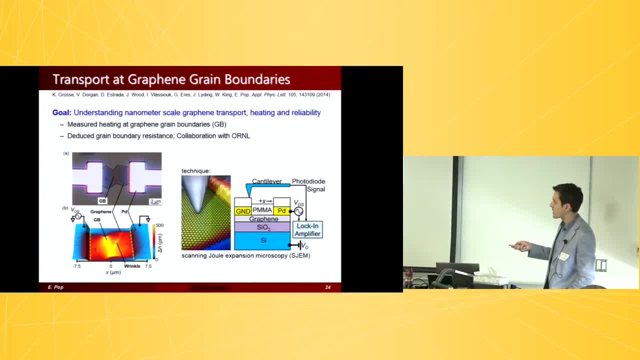 So here's a juncture of two graphene grains. This is a grain boundary. There's a wrinkle. You can actually see significant heating at the grain boundary. You can see a little bit less heating at the wrinkle. So you can kind of know which one is more resistive, which one isn't. 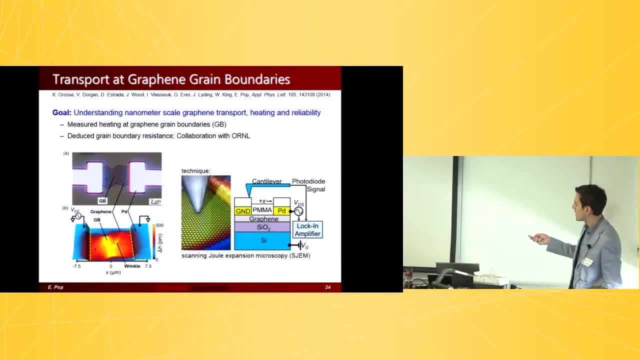 And this is actually probably a better picture. You can see here that the AFM tip essentially scans over the graphene covered by a PMA layer, and that's what's actually causing the thermomechanical loss. So it's actually causing the thermomechanical expansion. 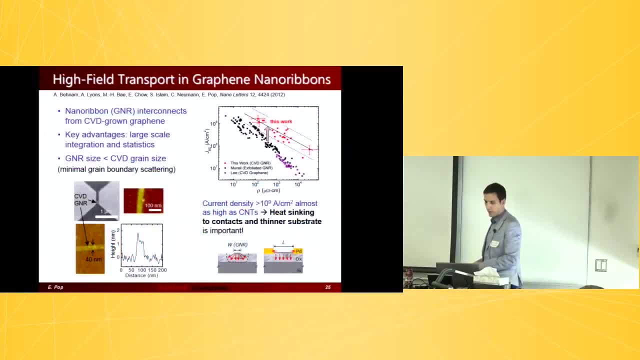 which we can then pick up with the AFM. Okay, A little bit of thermal engineering went into this work. Graphene nanoribbons: we were interested in them for interconnects, of course, And what we realized is that actually, by engineering the heat sinking into the contacts, 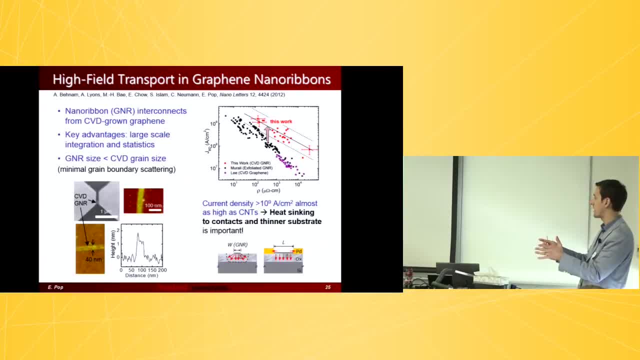 by essentially making short channels. so this is not significant engineering. but yes, we realized. yeah, if you make short channels you can actually get a lot of heat sinking to the contacts. And then if we make thin oxides for the substrate, 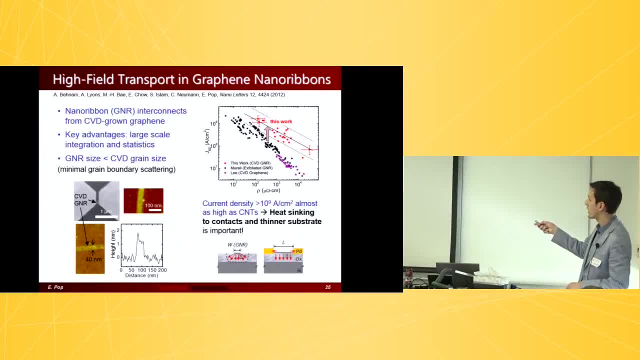 you can actually get more heat sinking into the substrate. So we were actually able to get significantly increased current densities, basically more than a gigaamp per square centimeter, through these graphene nanoribbons. These are actually CVD-grown graphene nanoribbons. 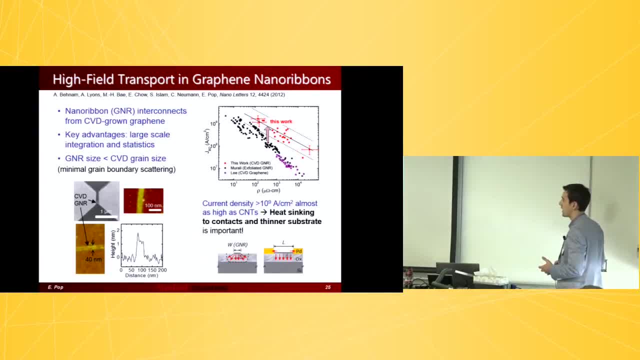 so they're not even particularly great for low-field measurements, But actually at high field they were quite impressive. They were almost as good as carbon nanotubes as far as current density is concerned, And this is basically just going to show you. 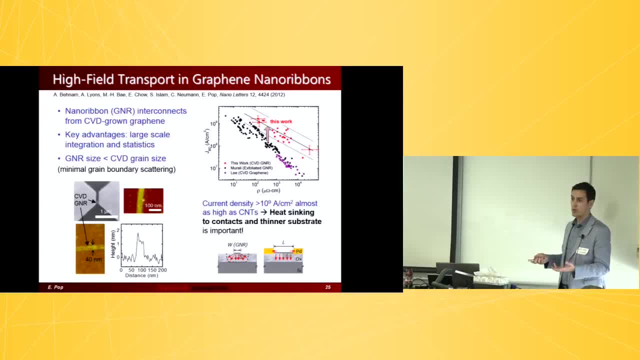 kind of a simple example to show that just a little bit of thermal engineering can actually really help you with some of these 2D materials can help you sink more current, for example, if you sort of engineer the dimensions and the materials around them just a little bit. 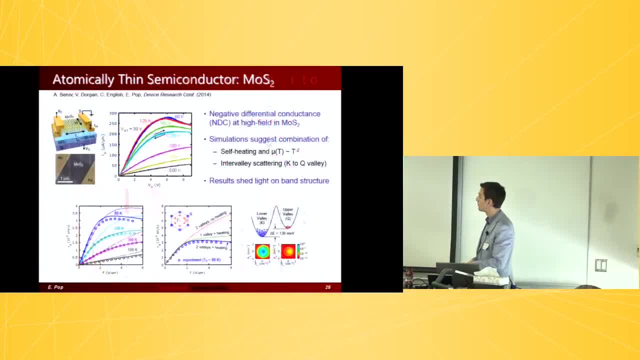 You can actually get quite a bit of increase in current Some similar work in MOS2, which we've been pursuing recently. we've been seeing some strange effects at high field and low temperature in MOS2.. You can see this negative differential conductance. 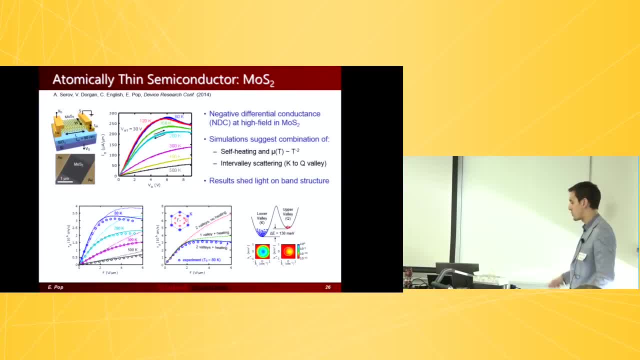 The current goes up and then the current comes back down And, of course, us being who we are, we said: well, this clearly must be self-heating. We've done this in graphene. Of course, self-heating must play a role in MOS2.. 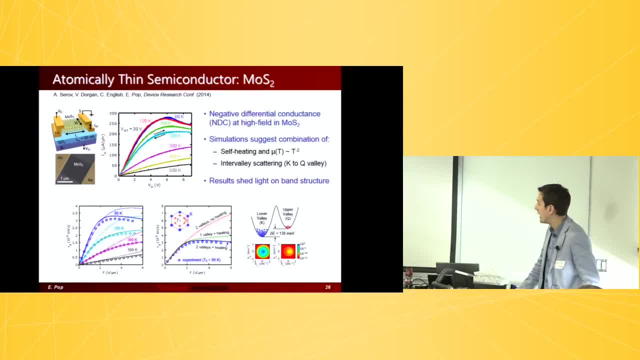 But it turns out we weren't able to explain it purely through self-heating. And that's when we started digging a little bit more through the band structure of MOS2, and we realized that there's probably a lot of intervalley scattering that is actually happening between these k and q values. 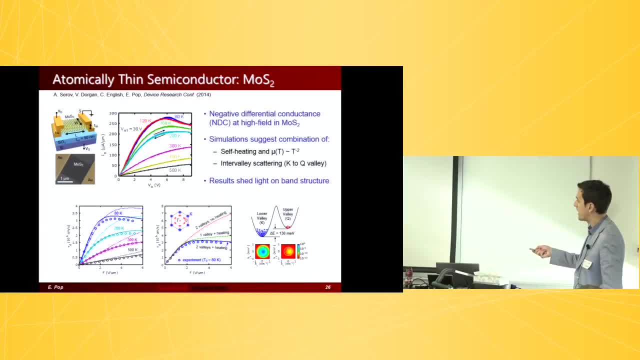 which I mentioned a little bit earlier. So you can see that if you include heating or if you include two valleys, you can't reproduce the experimental data, But if you include both the valleys and the heating, we're actually able to reproduce the experimental data across a wider range of temperatures. 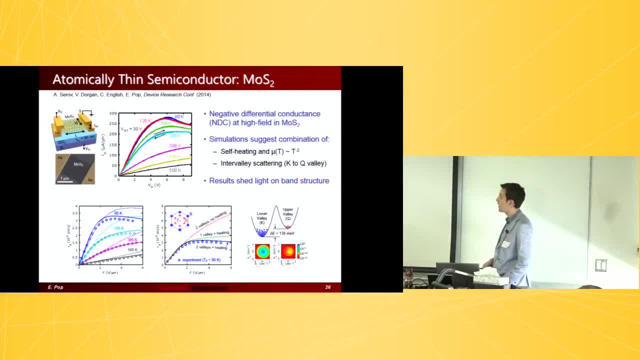 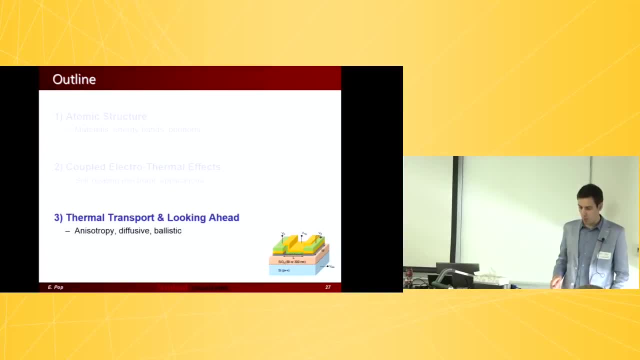 and across a wider range of fields, of course. So the last part of my talk is more purely focused not only on the thermal properties and a summary of them, actually really trying to wrap up- but also looking ahead and seeing what new functionalities we could enable by engineering thermal transfer. 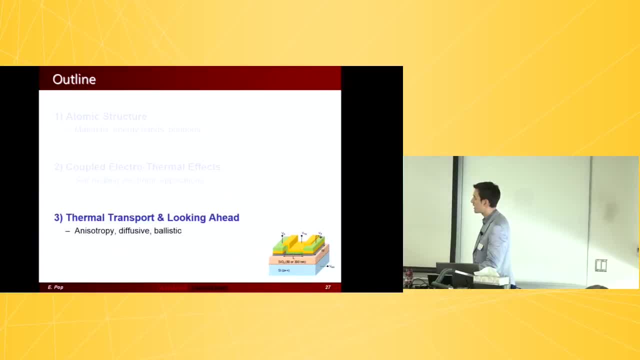 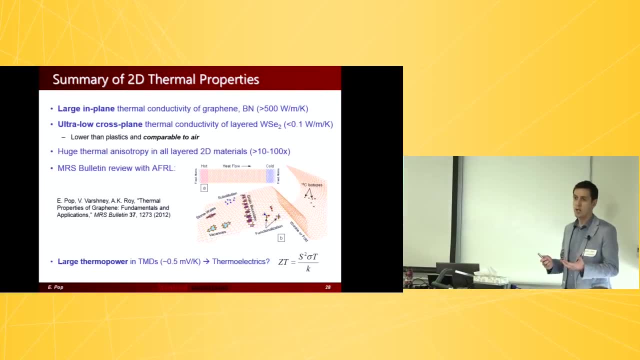 besides the ones that I've already shown you, which are fairly simplistic at the device level. So here's a summary. If I were to summarize, maybe, this talk on one slide, perhaps this is it. The takeaways are that there are some really large in-plane thermal conductivities. 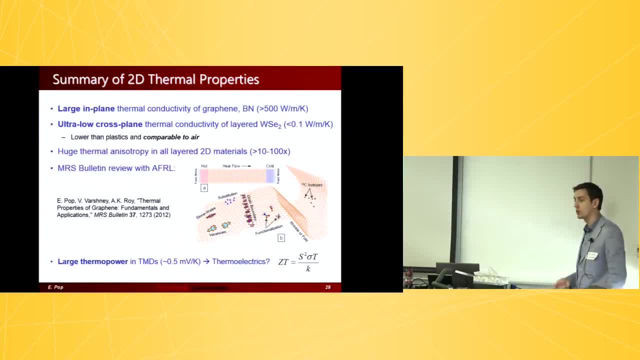 for graphene and boron nitride, really large, larger than metals, larger than copper, for instance. Copper is about 400.. These things are about 500 and above at room temperature, of course. But at the same time as I hinted about 15 minutes ago, 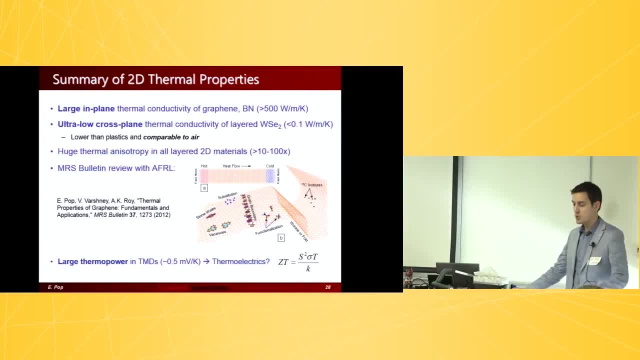 the cross-plane thermal conductivities are extremely low. This has to do with the very, very weak coupling between layers and the weak Van der Waals coupling between the layers and the environment, as you can imagine- And there's actually some data from a few years ago showing that tungsten diselenide. 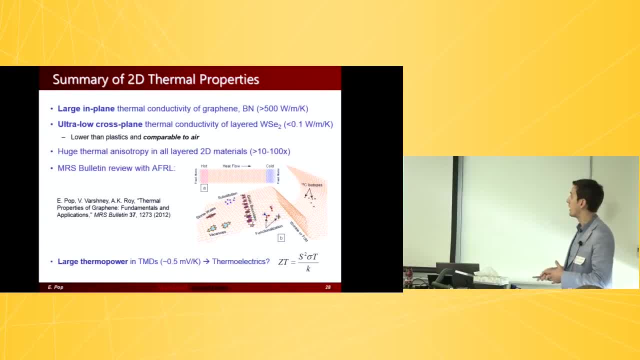 has actually thermal conductivity, cross-plane, of course, lower than 0.1 watts per minute And it's actually lower than a millimeter Kelvin, which is actually lower than some plastics and almost comparable to air. So this is kind of – it's very mind-boggling in a way that a material could have such – 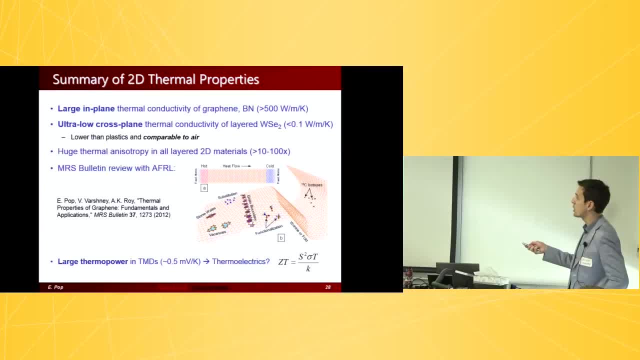 this is a solid material that has such low thermal conductivity cross-plane, So there's a huge amount of thermal anisotropy pretty much in all layer 2D materials period. We wrote a little review paper with Air Force Research Labs collaborators. 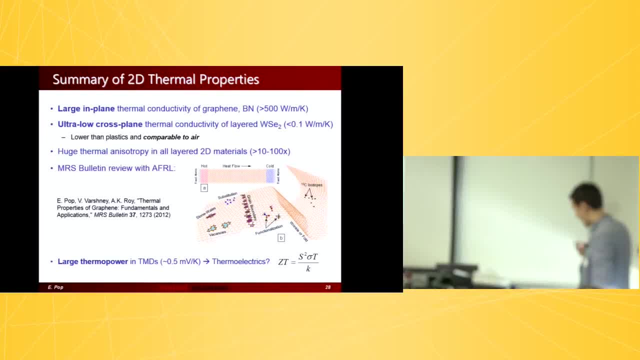 This was more focused on graphene, so we're writing another one right now that's more focused on TMDs. It hasn't come out yet, but some of the figures I'm about to show you are actually from the new paper that we're writing up. 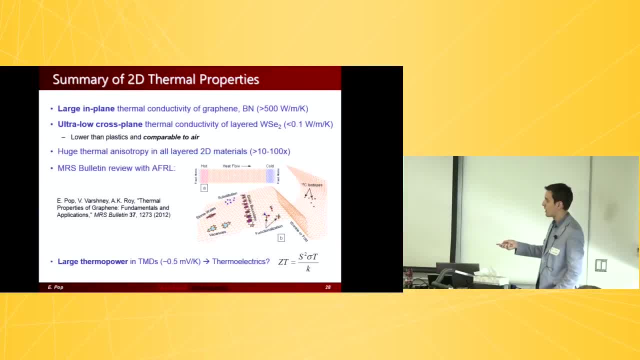 And actually, before I move on, I just want to point out that there's been some measurements of thermal power in these TMDs and people are getting really large numbers. But I want to put those into context because I think there's been a lot of rush to say. 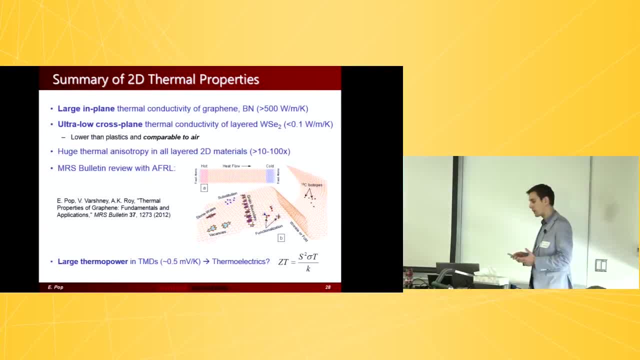 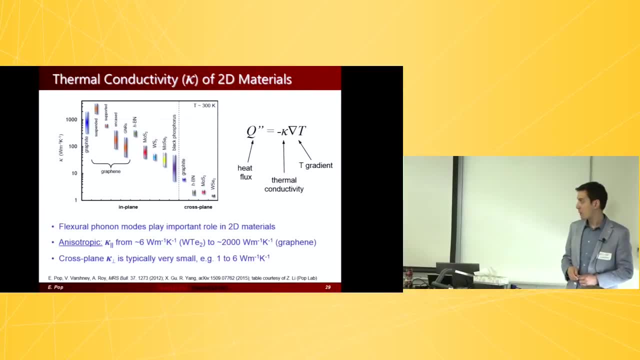 hey, you know, these actually have like amazing thermoelectric properties, but really we should probably put that into context, as I'll show in a moment. So here's a summary – this is a summary from the upcoming review paper – 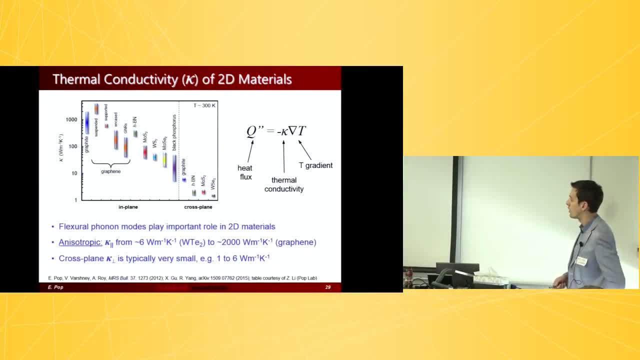 a summary of the thermal conductivity of a whole family of 2D materials, and we had to – absolutely had to – split these by in-plane and cross-plane measurements. So you see, these are the graphite suspended, supported, encased graphene nanoribbons that we've measured. 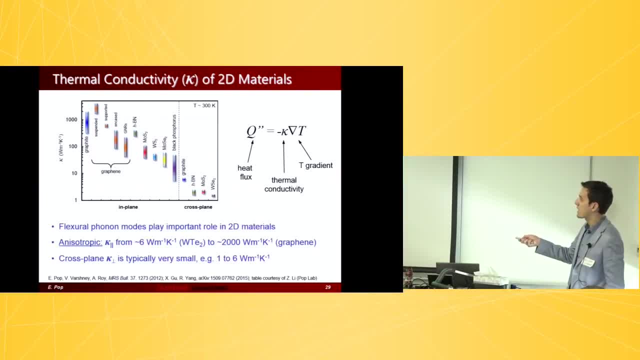 This is the graphene Boron nitride. pretty good, Notice, the vertical axis is logarithmic. This is a huge, huge range for thermal properties. Thermal properties do not, you know, vary like electrical properties, They only vary – you can only really vary them in solids by three or four orders of magnitude. 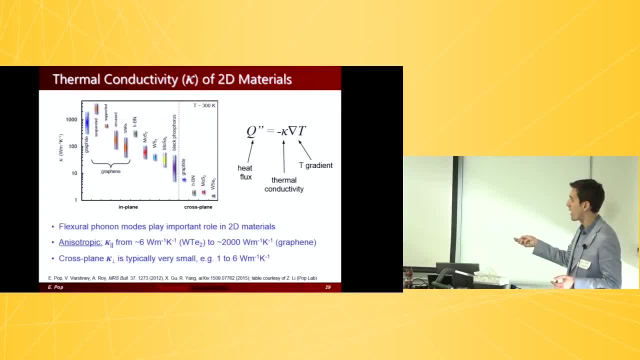 This is it for pretty much all solids, right? Maybe you can go another order of magnitude lower in really really disordered things or plastics, The TMDs, black phosphorus, pretty low thermal conductivity. But then if you want really low thermal conductivity, of course you have to go cross-plane, right. 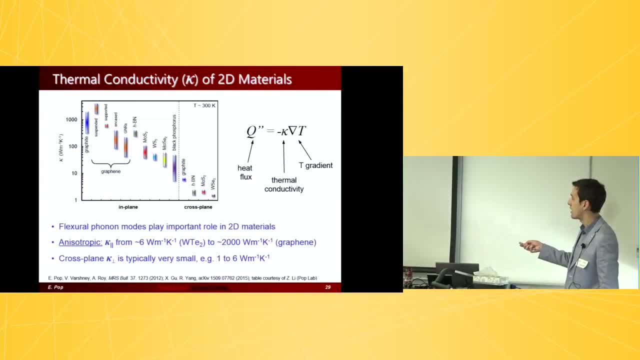 So even graphite has terrible conductivity, cross-plane. Even boron nitride, some of the TMDs and so on, right. So again, the take-home message here is this: anisotropic thermal nature of 2D materials, right. 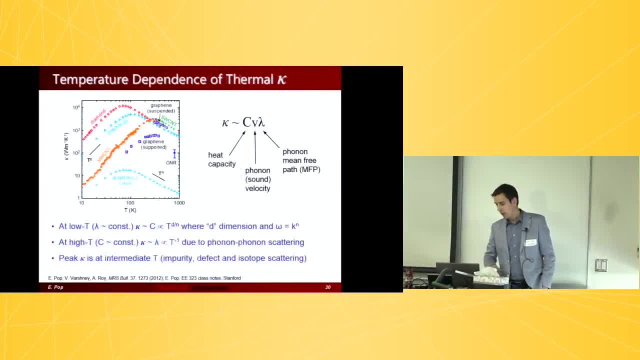 Very, very low thermal conductivity. Another –, by the way, everything I've shown, unless I mention it specifically, everything I show you is room temperature, because that's generally where I really kind of you know inhabit. literally is I like room temperature? 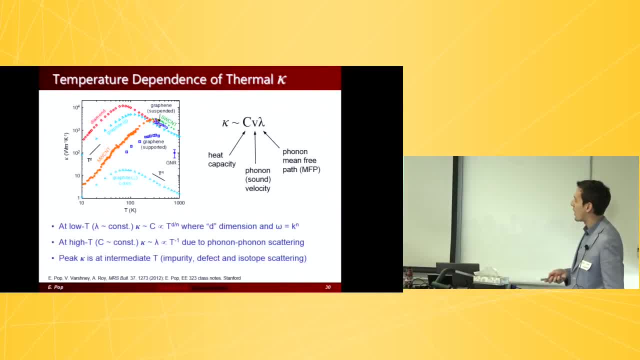 So – but here's a bit on the temperature dependence of thermal conductivity. So the temperature dependence of thermal conductivity looks basically like an upside-down V or upside-down U, depending on which letter you like better, And so at low temperature it scales as the heat capacity, which I already covered, right. 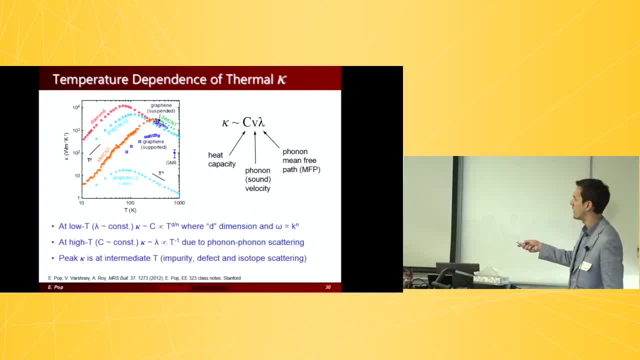 It goes – but this is really low temperature. It's 10 to 100 Kelvin. So thermal conductivity scales as heat capacity, because you have more and more phonon modes which are occupied and so on right, But then you hit a temperature where you've sort of occupied all the phonon modes that are kind of relevant to occupy. 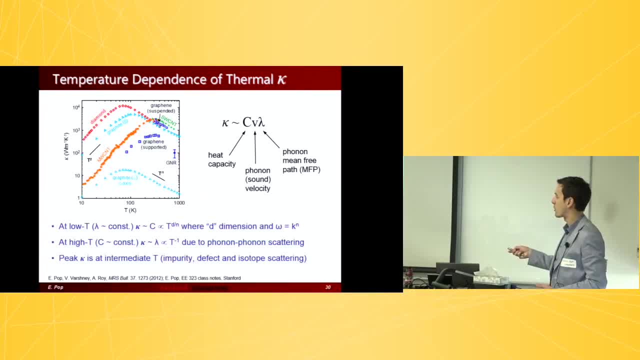 And so then phonon-phonon scattering really starts to come into play, And then you start getting this thermal conductivity that scales as 1 over temperature, right? And so you see this above, you know, 1 over temperature Right. 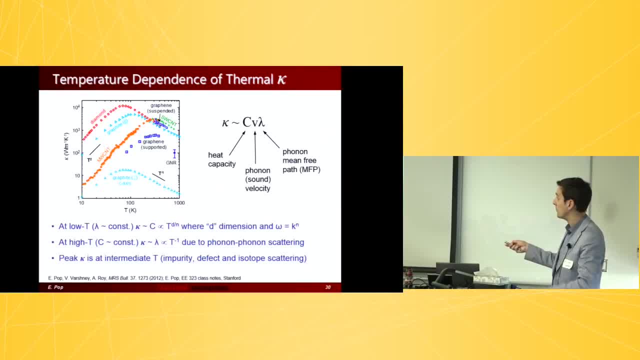 In graphite and pretty much all these nanotubes and so on, right, And this is due basically to what's called UMCOP phonon-phonon scattering, right. And so for most of these materials, 2D materials or otherwise, the peak thermal conductivity actually occurs at some intermediate temperature, depending on the impurity or defect scattering in the sample. 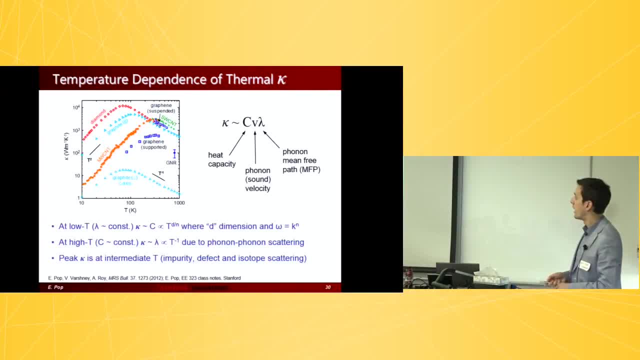 But this temperature you can – if you squint and you're in the back, you can kind of look like peak thermal conductivity is around a hundred degrees Right, Not at room temperature. At room temperature you're already on the downward slope, so to speak, right. 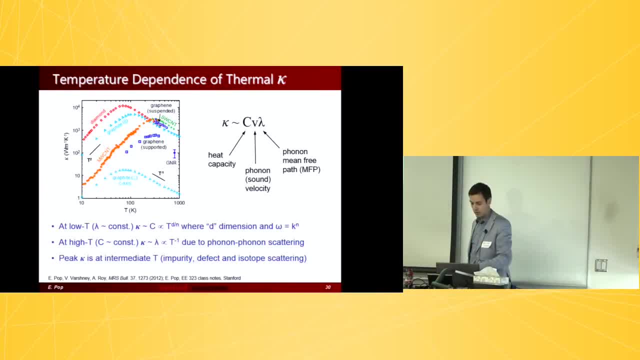 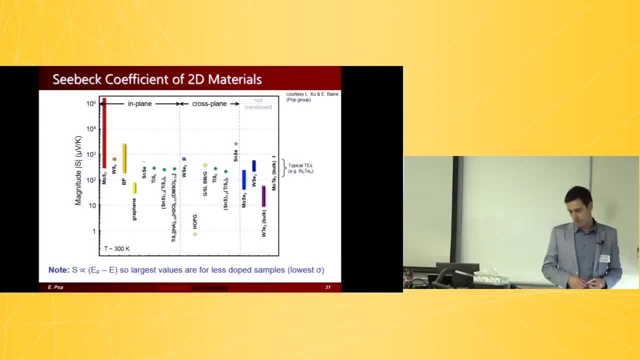 But certainly at a hundred Kelvin, pretty high thermal conductivity, Actually even higher, of course. So a couple of words on the Seebeck coefficient. This is, by the way, all at room temperature. So my students Lily and Elise went through literature and they just did this wonderful search of the magnitude of the Seebeck coefficient. 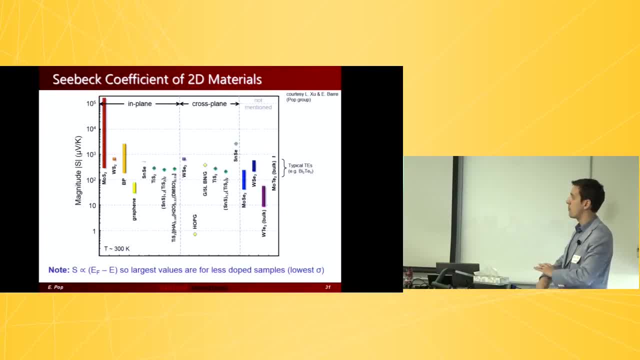 This is, by the way, all measured right, And so you see this amazing, amazingly rich data set which you know so far. the only way we can really group it is by in-plane and then cross-plane measurements. I think I'm running out of battery. 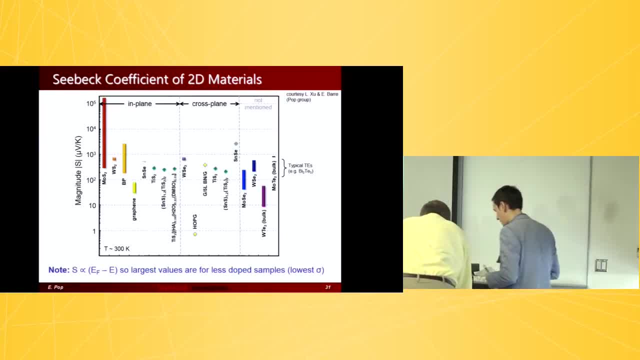 Do you have another one by any chance? Oh, there is a backup. No, there's just no batteries at all. Oh, okay, All right. Okay, that's fine, I'll just use the analog pointer, So anyway. so we just grouped these by in-plane. 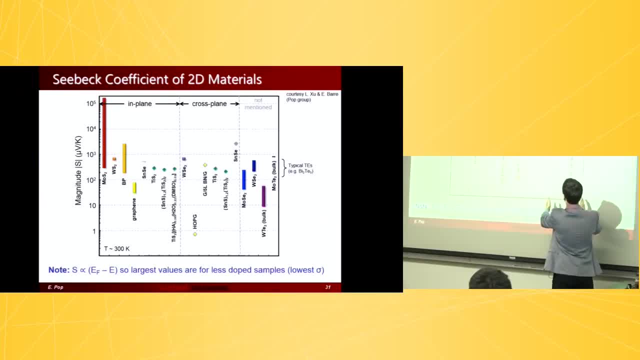 And then cross-plane measurements And then there's some bulk measurements here which were actually not mentioned, So I'm not sure To compare these. the Seebeck coefficient- the magnitude typical for thermoelectrics- is in that range about 100 to 1,000 microvolts per Kelvin. 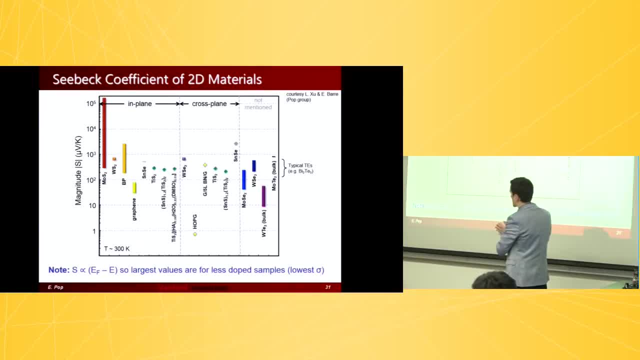 But what I want to remind you- and this is why I want to put this into context- is that the Seebeck coefficient of materials is proportional to the energy difference between the Fermi level and where the electrons or the holes are traveling. So if you have a really undoped material where the Fermi level is in the middle of the gap, the Seebeck coefficient is going to be huge, right. 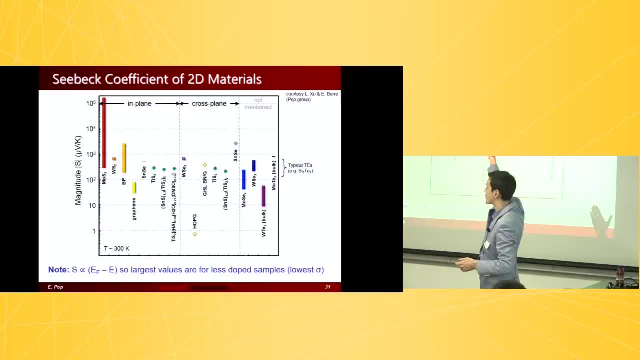 And so these very, very large values that were measured for MOS2 were actually for relatively clean, undoped samples, right. And so, if you remember the ZT formula that I flashed a couple of slides earlier, to actually have good thermoelectrics, not only do you need large Seebeck coefficient, but you also need large electrical conductivity. 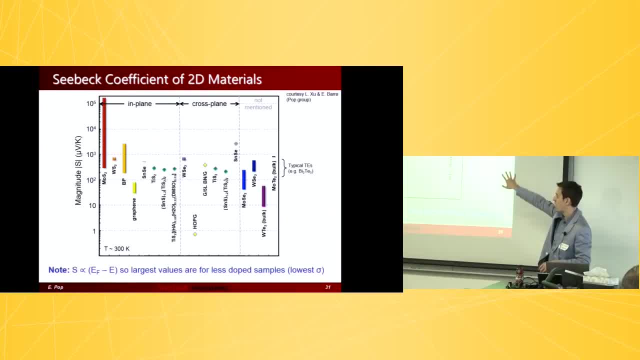 Okay. So the problem is that you know, just to kind of put these pictures into context, some of these very large Seebeck coefficients that were measured A- the electrical conductivity was not reported on the same sample. So I don't even know how to summarize this any better than we already did. 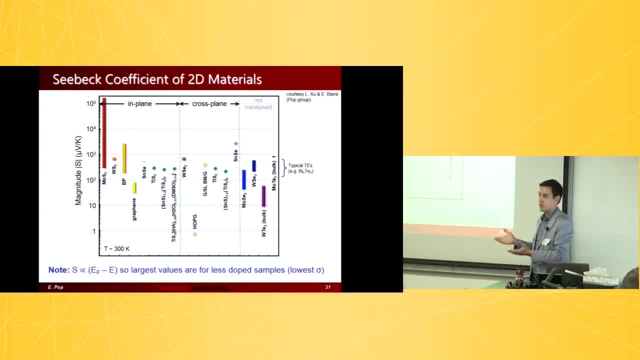 But B also. I know from basic physics that you know the range that we show. some of the largest ends of the range are actually for the least doped samples, right when you're actually gating them with a Fermi level in the middle of the gap. 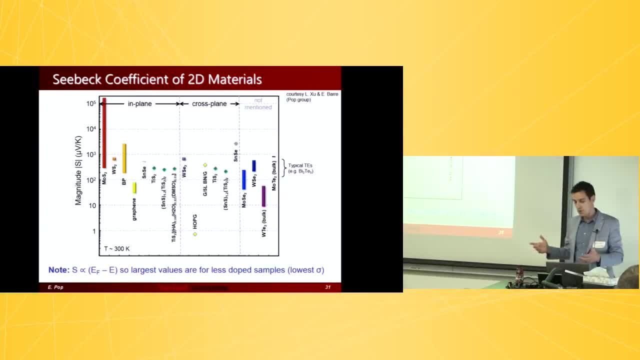 And those will have really, really low electrical conductivity. So of course they're not necessarily the most useful samples, But there's still some trends that emerge. For instance, tin selenide has some interesting thermoelectric properties, for instance. 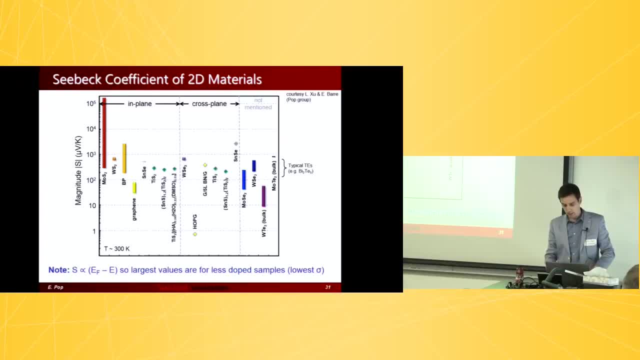 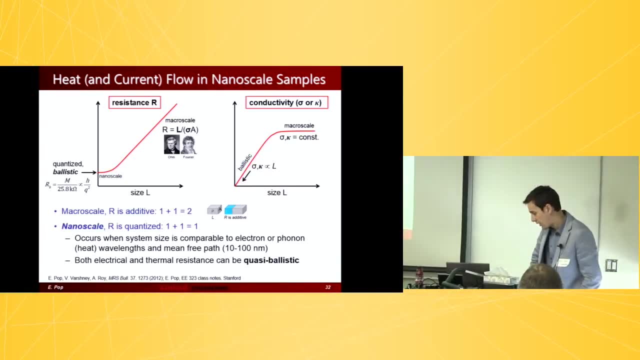 You know. so there's definitely, I think, a lot to be learned here as well. Okay, A couple of words about nanoscale samples. I think you know, I think a lot of us recognize that you know devices, transistors, interconnections and so on. they're not necessarily the most useful samples. 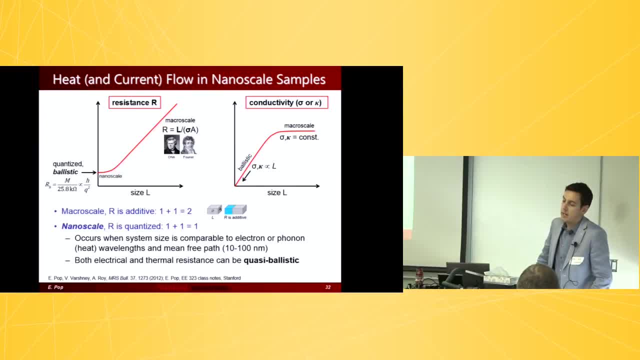 Okay, You know, they're sort of thank you. they're sort of very cool when they're, you know, less than a micron in scale, right, If they're bigger than a micron, it's sort of you know. you go to Intel, you give a talk and they sort of like: what's the point, right? 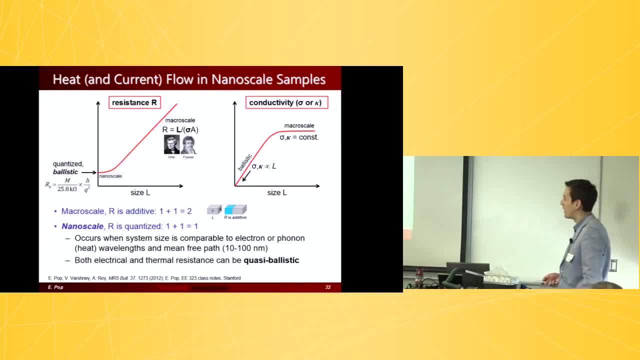 But if it's less than a micron right, or preferably less than you know, 50 nanometers or so. you know, things are kind of interesting, Plus the physics is also kind of cool, And so what you probably know from you know, I don't know. 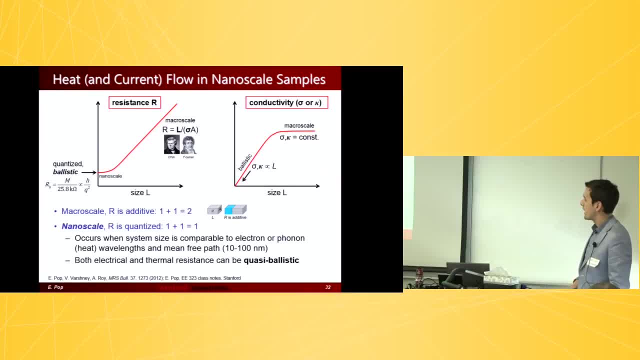 What you probably know from resistance, electrical resistance, is that you know Ohm and Fourier. you know Ohm's law, you know holds all the way until you reach nanoscale right. But the same thing happens with Fourier as well. 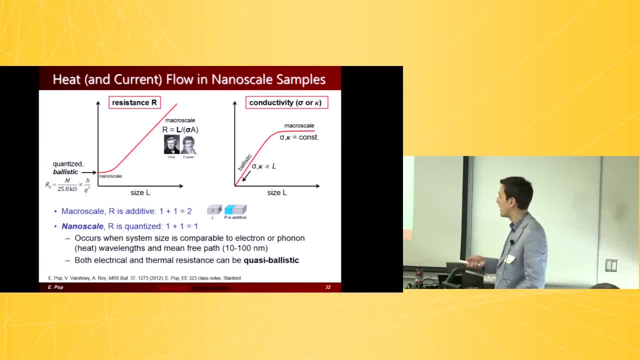 So, Fourier's, you know, thermal laws hold all the way until you reach a nanoscale, But then, when you actually get to very, very small dimensions, you can have quantized resistance, ballistic effects both electronically as well as thermally right. 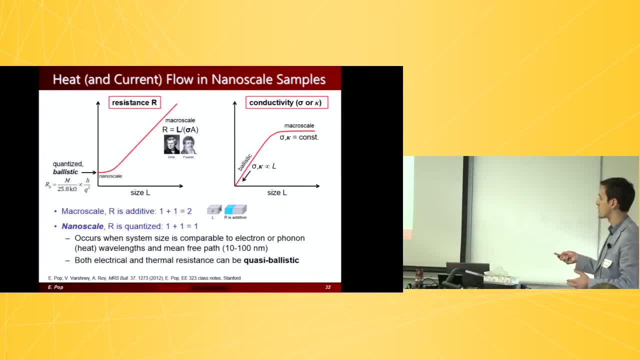 In fact there's some weird math. You know macroscale. you know you take a resistor. You add another resistor, You make it longer, The resistance goes up right. One plus one equals to two In the nanoscale. if you have two ballistic resistors and you know you take a ballistic resistor, put it in series with another ballistic resistor: you still have a ballistic resistor. 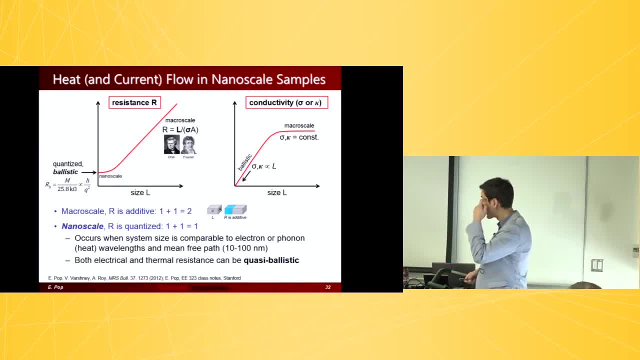 So it's kind of a funny math that one plus one is equal to one. essentially, That's what that means. When do these things happen? These things happen at dimensions of 10 to 100 nanometers, right? So that's basically when these things are occurring. 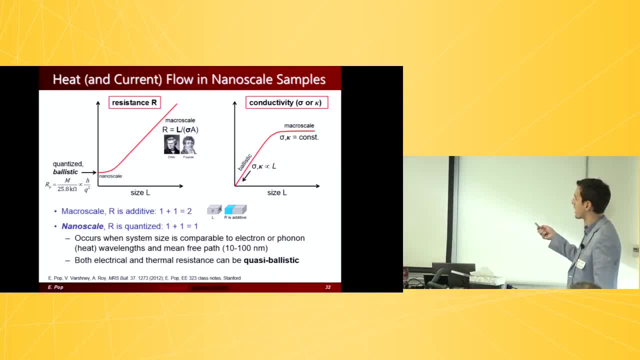 And I do want to point out the difference between resistance or conduction. So if you convert between resistance and conductivity using just that simple equation in bulk, in the macroscale of course conductivity is a constant. But actually in the ballistic regime- and this is a little counterintuitive- in the ballistic regime the conductivity actually goes to zero. 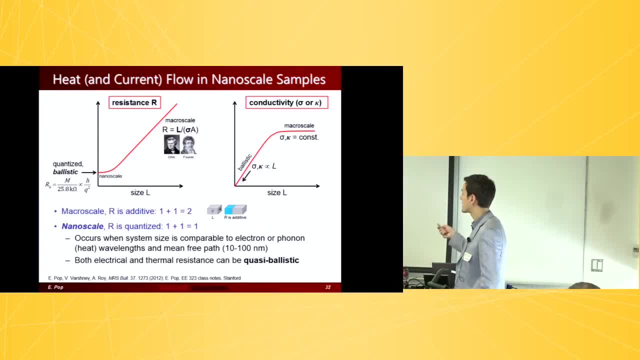 And it scales linearly with the system size. Otherwise, if the conductivity doesn't go to zero, you're not going to obtain a constant conductance right. And so I remember as a student, the first time I saw this, I said: wait a second. 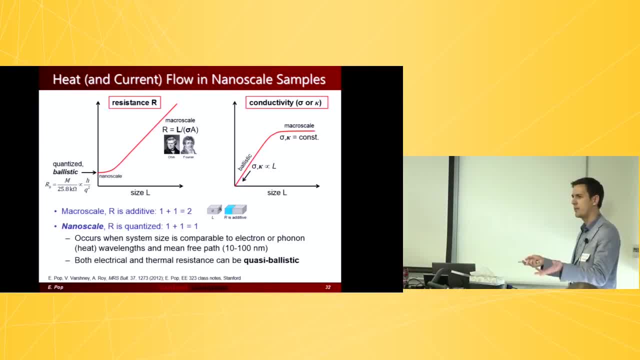 If it's ballistic, shouldn't the conductivity go to zero? If it's ballistic, shouldn't the conductivity go to infinity? Actually, the conductivity goes to zero because the conductance goes to a constant And the math is actually right there on the slide. 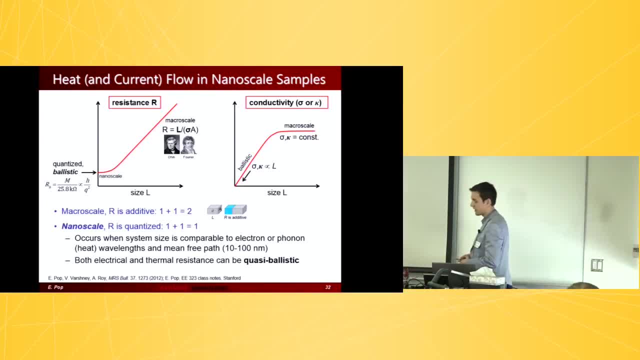 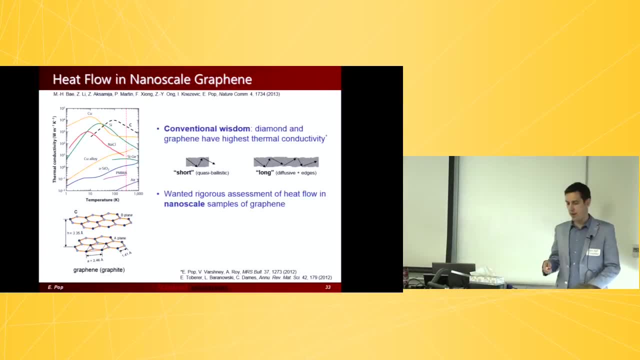 It's very, very simple, But that's something that I think you know sometimes perhaps slips through the cracks, And so we look for these kinds of effects in graphene, Because the conventional wisdom would be that, of course, diamond and graphene are going to have the highest- you know the best- ballistic effects: thermal ballistic effects at room temperature. 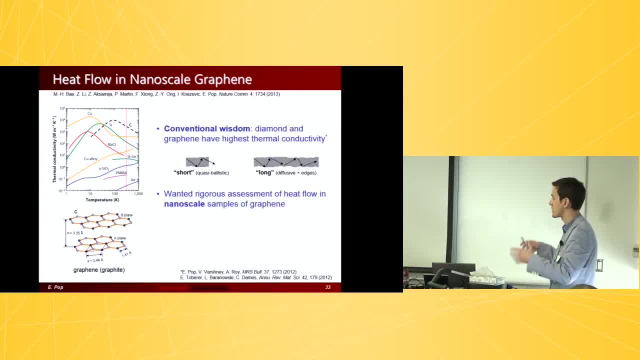 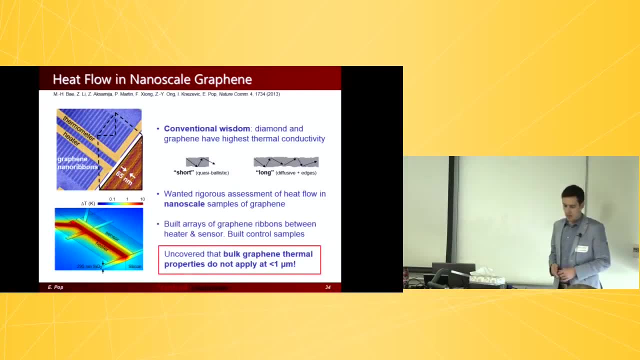 Because they're the most thermally conductive, they have the largest phonon, mean free paths and so on right, And we built these test structures which you know. this whole project was probably one of the longest projects in my lab because so many things went wrong while we were doing this. 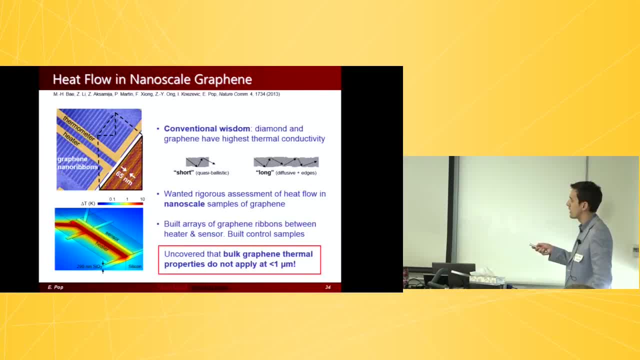 But we put heaters, We put thermometers. These are graphene ribbons. Some of these are nano ribbons, Some of them are just ribbons. right, I'm showing one of the nano ribbons here, But we also had much larger ribbons. 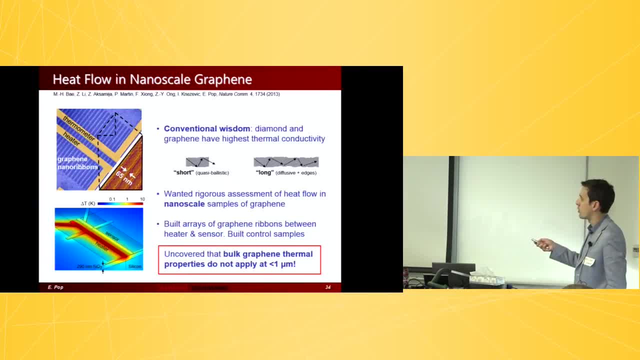 And the array ensures that we get enough heat flow between the heater and the thermometer. It kind of looks like a thermal transistor. if you will right, It is a source and a drain, except there's a heater and a thermometer. And again, if there's one take-home message here, it's this boxed red thing- is that we uncovered that the thermal properties of bulk graphite or graphene that I showed you earlier really only apply in samples greater than a micron. 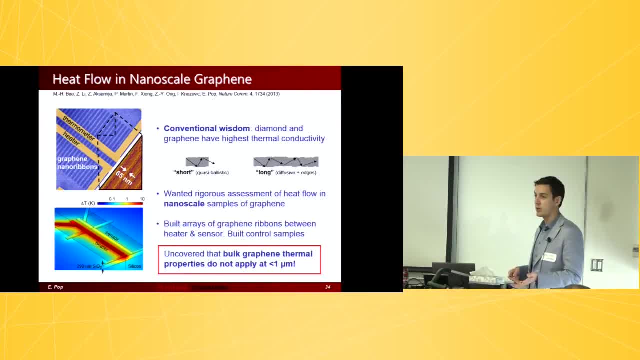 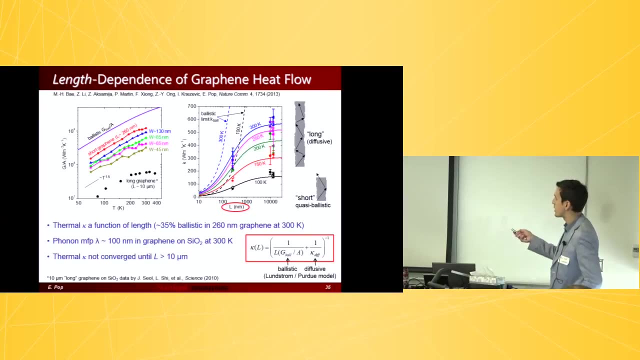 If you go in samples less than a micron, you actually can't use the bulk thermal properties I showed you earlier The thermal conductivity. Why? Because you have these ballistic effects and you know weird edge scattering effects happening. So, essentially, I know this is a really busy slide so I'll just refer you to this paper from three years ago. 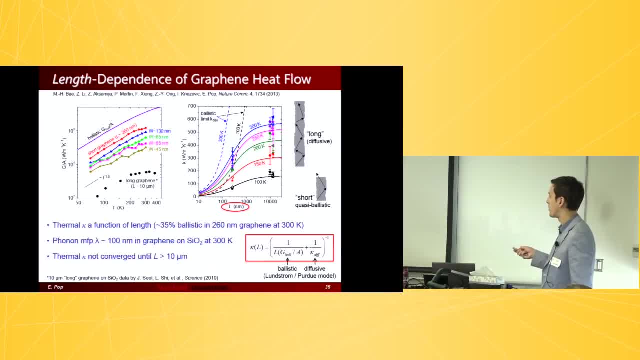 But to make a long story short, the thermal conductivity becomes a function of length. That's actually a ballistic effect which you kind of expect, just based on what I said earlier. The conductance is starting to become quantized And therefore the conductivity appears to increase. 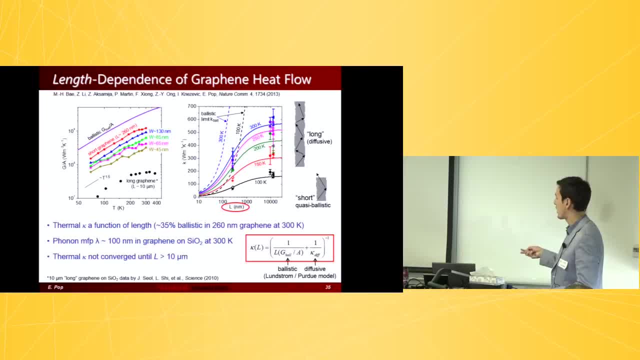 So essentially decrease, Right. And so actually there's a very, very simple model following Mark Lundstrom's work from Purdue, on how to kind of bridge the diffusive and the ballistic regime, And actually that seems to fit the data very, very nicely. 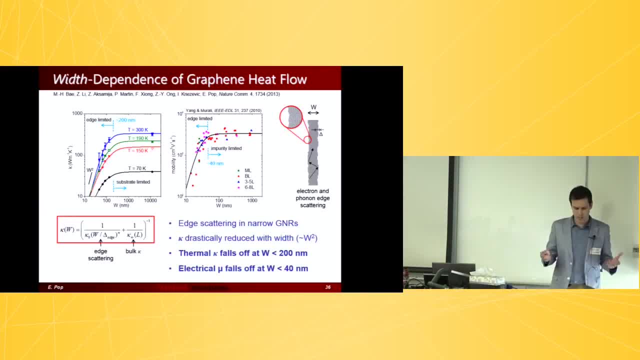 And then the other thing is the width dependence, And the width dependence is maybe a little bit more classical in the sense that, yeah, if you have ribbons they have edges. You know, If you have ribbons, the edges are not perfect, because we etch these by oxygen plasma. 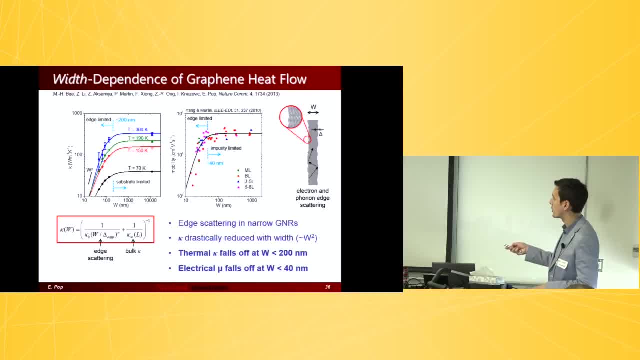 Right, And so the thermal conductivity is actually going to decrease as a function of width, And the thermal conductivity falls off at widths less than about 200 nanometers. So when these ribbons are narrower than 200 nanometers, the thermal conductivity drops precipitously as W squared. 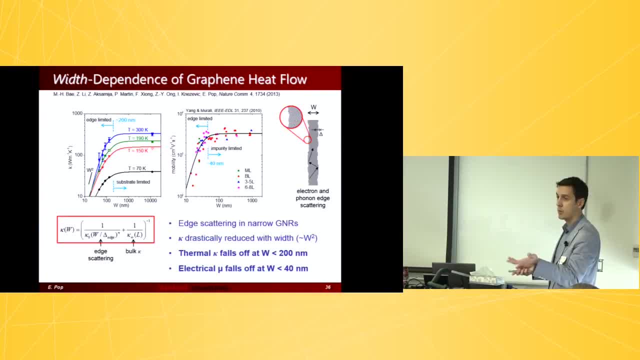 And then if it's above that, it's actually limited by scattering with the substrate. Very similar stuff is actually seen electronically, Except electronically. the mobility seems to decrease. So electronically the mobility seems to fall off for widths below 40 nanometers. 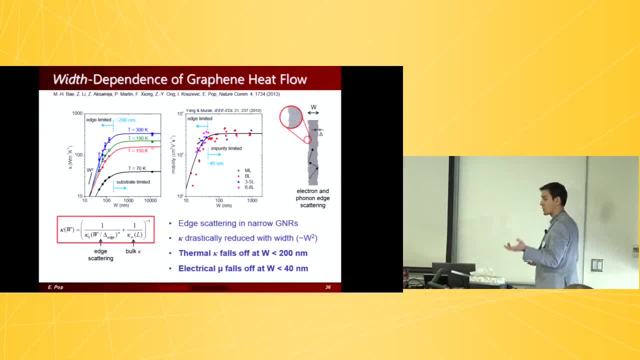 So clearly the difference is between a thermal regime and the electrical edge regime. is that: Is that my timer? Yeah, No, but Okay, But it's. But might as well be Yeah, Yeah, Yeah, Yeah, I've got. 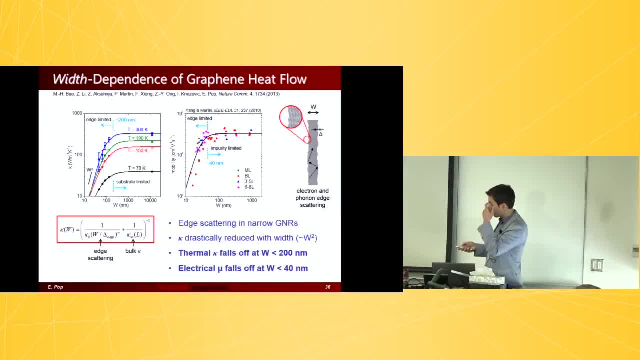 It was serendipitous: Two slides. Yeah, I've got two slides, I think, of technical content. I'm done, Yeah, So the fact that the electron mobility falls off at larger scales, the electron mobility falls off at smaller widths, actually has to do with the 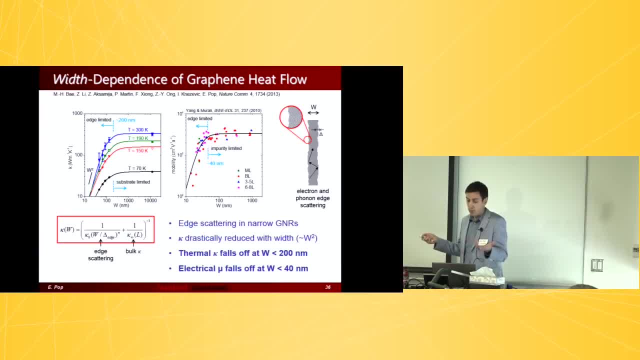 With the phonon and electron mean-free path being different. The phonon mean-free path is actually longer. So you start seeing nanoscale effects in phonons before you see them in electrons, at least in graphene. This, I'm not going to describe this slide too much. 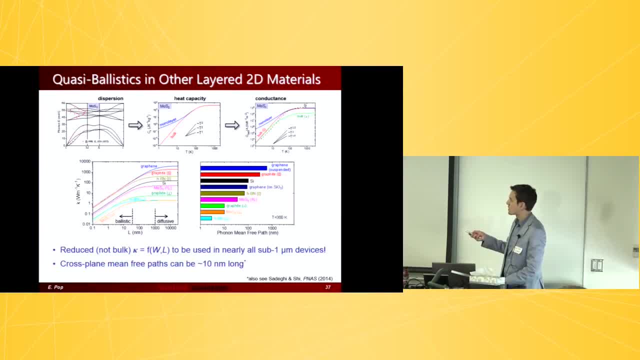 Again, it's from the upcoming review paper, But we essentially look at these ballistic effects in a whole host of other 2D materials, Distinguishing between where the ballistic regime is and where the diffusive regime is. And again, if I could just come up with a single, 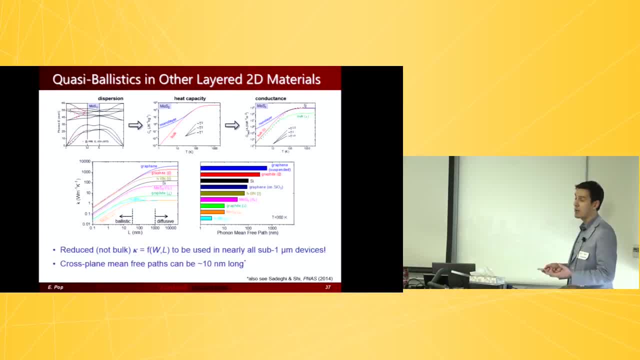 Simple take-home message is that it's really really probably not a good idea to use the bulk thermal properties in almost all submicron devices, Right? Not even Not just in graphene, but even in, you know, submicron devices not based on graphene. 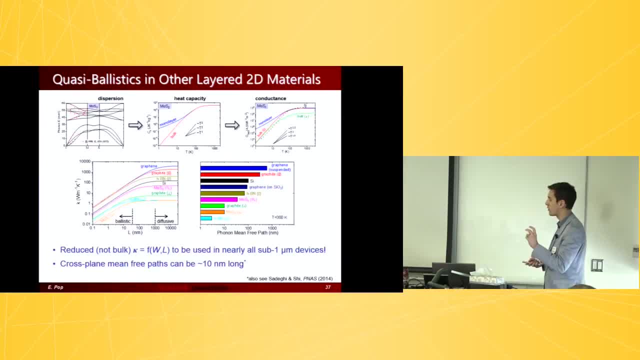 Even in MOS2, you probably ought to adjust the thermal conductivity for these quasi-ballistic effects. Not only that, but the cross-plane mean-free paths. So even in mean-free paths cross-plane could actually be spanning, you know, something like 20, 30 layers. 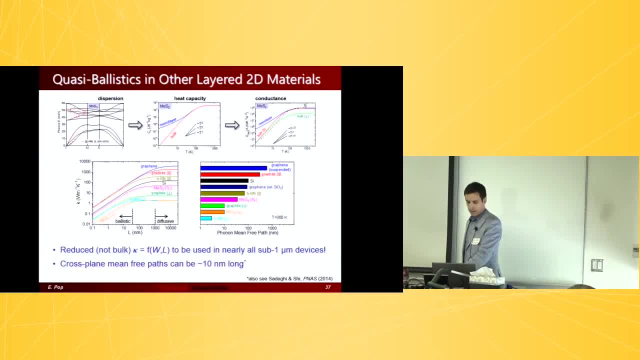 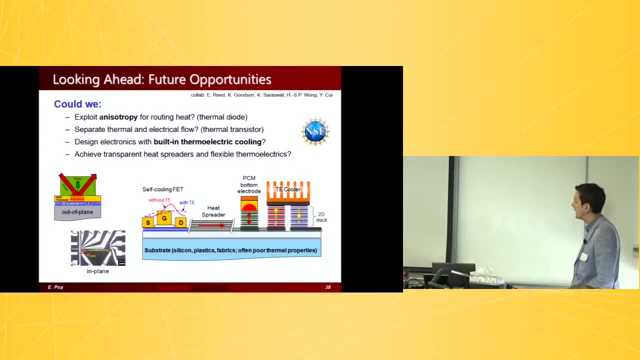 Because the cross-plane mean-free paths are actually quite long as well. Okay, So just a couple, Just two words, Not really technical slides on future outlook. We have a little NSF program, an NSF EFRI, that's sort of built around these ideas. 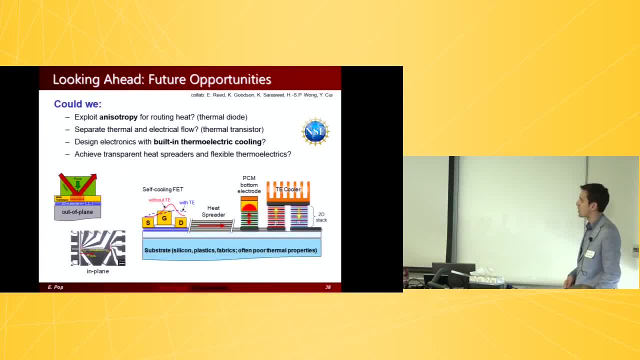 And so some of the ideas are: you know, how do we exploit anisotropy? How do we, you know, leverage this built-in thermoelectric cooling? You know, can we do something really wacky. By the way, this is what I call. 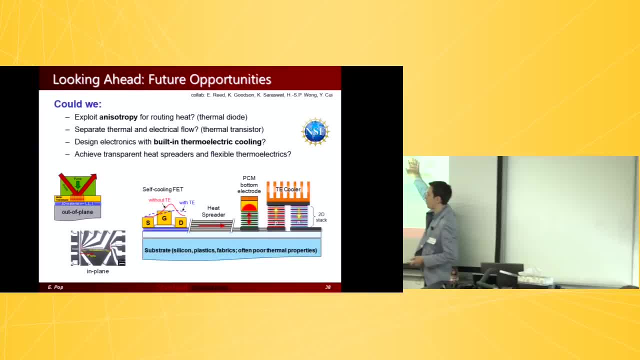 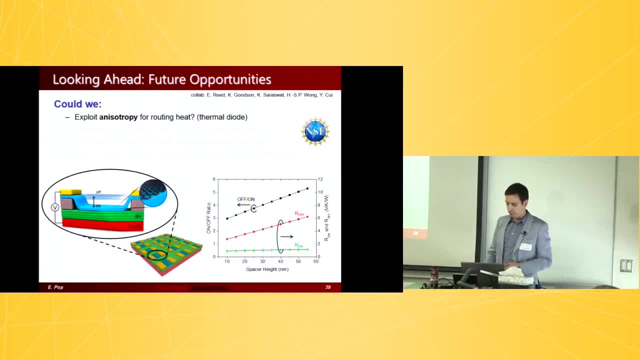 What I showed right here is what I call a PowerPoint device. Right, This is sort of a wishful thinking of some of the devices we could build, But we'll see if we can build them. And, you know, an example of something that we're trying to build right now is trying to build essentially a graphene MEMS device. 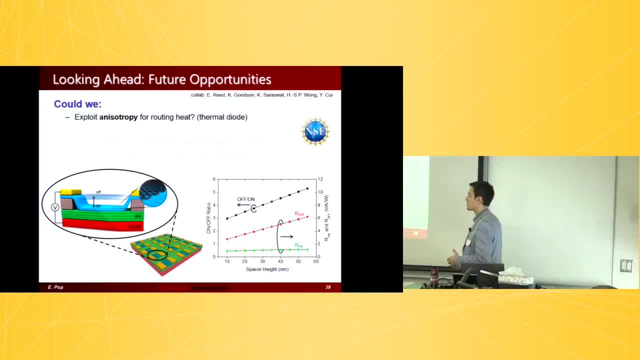 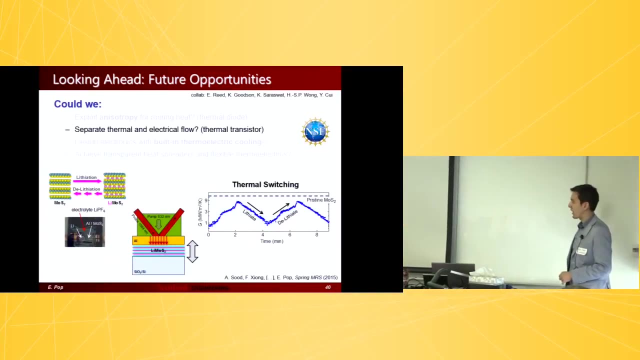 that leverages the flexibility of the material but also leverages its high thermal conductivity. So it's essentially a thermal switch that could be used in some analogous way to an electrical switch Right, But for routing heat, obviously. Another thing that we're building right now is we're working with some battery experts who have taught us that if you jam lithium ions inside MOS2,. 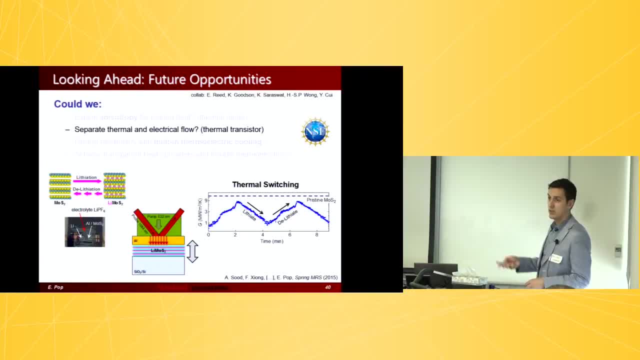 you can actually control its thermal conductivity by a lot. So this is actually also a thermal switch. It's more of a thermal transistor, because you can think of the lithium as sort of gating the thermal, the heat flow Right. So lithium goes in, kind of slightly increases the separation of the MOS2 planes. 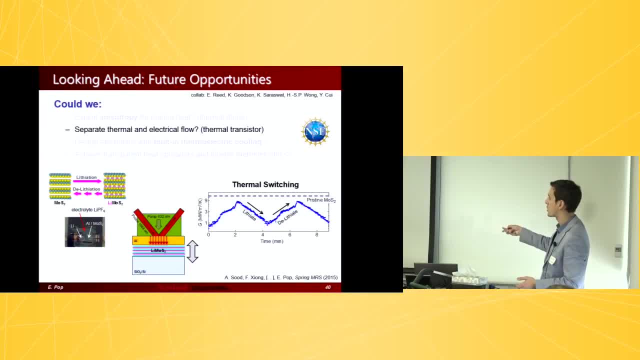 and the cross-plane thermal conductivity of the material actually gets modulated by almost an order of magnitude, which is quite remarkable. It's not very fast, mind you. This is time scaled in minutes, Right, But it's nevertheless. you know, it's remarkable. 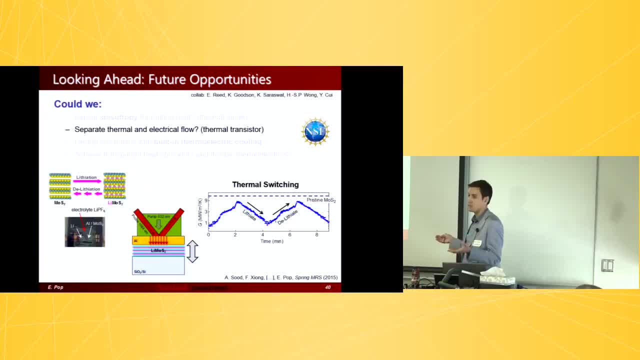 You know you can't do this with silicon. I can't modulate the thermal conductivity of silicon by an order of magnitude. and then you know, reversibly at all, At least I don't know how to do that. Okay. 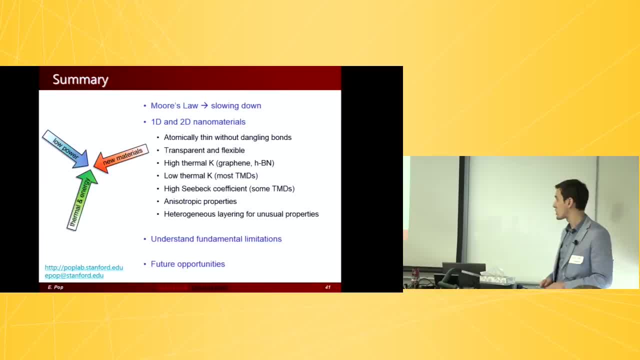 So just to summarize, you know some of the take-home messages are on 2D nanomaterials, especially 2D nanomaterials, Atomically thin of course, Some of them are transparent. Most of them are flexible. 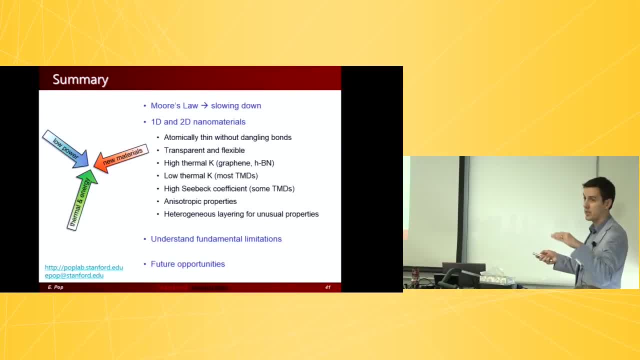 High thermal conductivity for some, especially in-plane Right Low thermal conductivity for most of them, especially out-of-plane Some high Seebeck coefficients. There's a big asterisk there, because the highest Seebeck coefficients are going to be at the lowest carrier density. 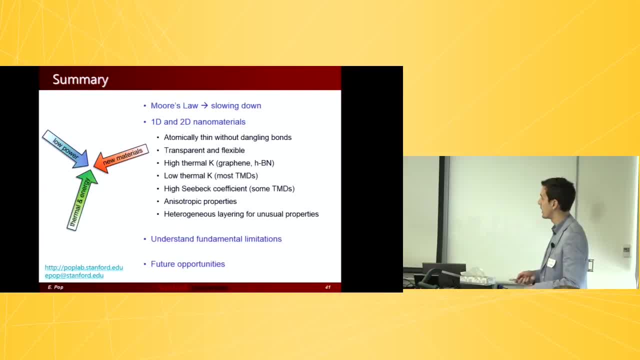 so not necessarily in a useful regime for thermoelectric. And then you know, I think there's a lot to be done with heterogeneous layering and really trying to understand the fundamental limitations of some of these things, as I'm sure you also saw in some of the previous talks. 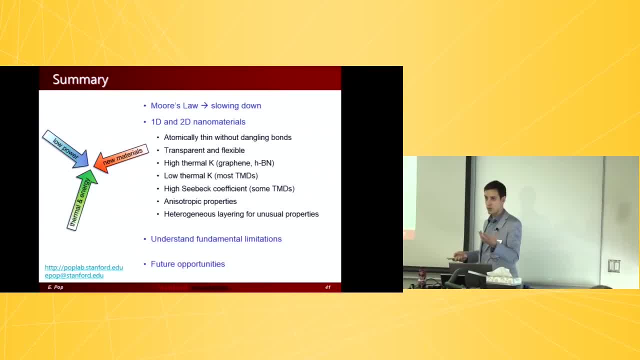 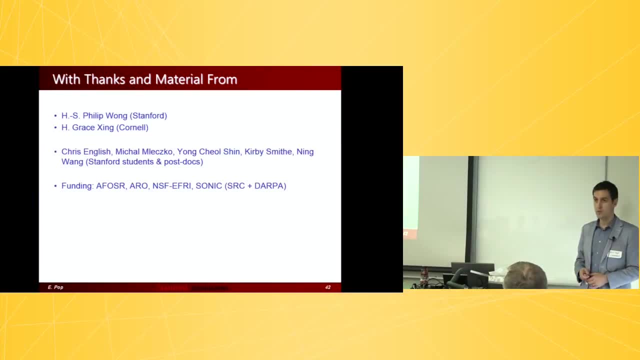 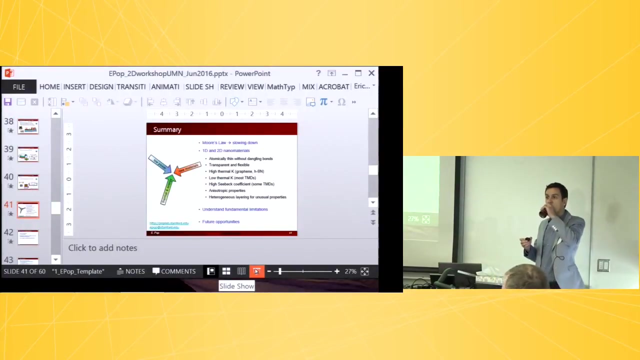 And so if you have other questions, I will take them right now or I'll accept emails later, And I just want to thank some of the people that have helped me with material for this talk. Thank you, Questions. Yeah, so the question was: why is the phonon mean-free path longer than the electron mean-free path? 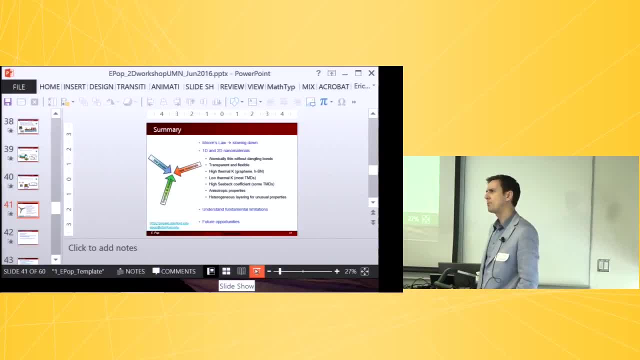 That's in graphene. by the way, That's only in graphene and boron nitride. probably That's the way the math works out basically. You know, in MOS2, the phonon mean-free path is probably comparable. It's the electron mean-free path. 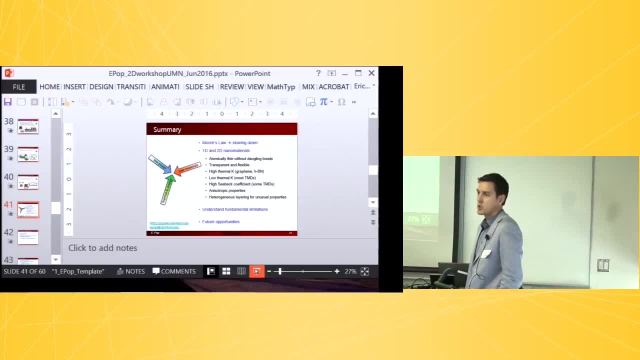 But in graphene the phonon group velocities are so large, the bonds are so strong that the phonons just propagate for huge distances before they scatter. So what do you mean by the mean-free path? I'm sorry, what's the question? 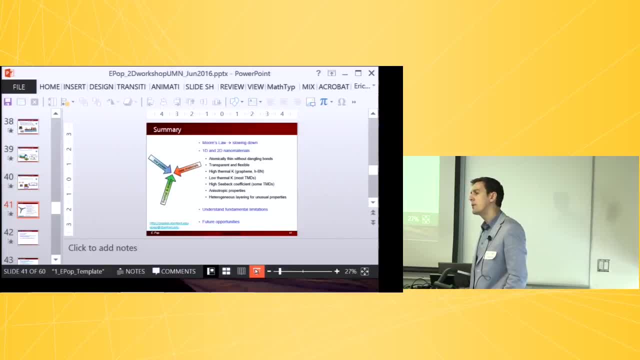 What do you mean by the mean-free path of phonons? The question is, what limits the mean-free path of phonons, Other phonons, so you have phonon-phonon scattering, Scattering with a substrate. If you have suspended graphene, you don't have a substrate. 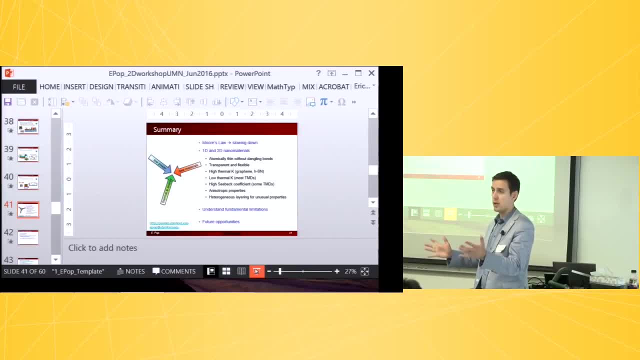 But if you have graphene on a substrate, or MOS2 on a substrate for that matter, you have scattering with the substrate, phonons as well. So you have phonon-phonon scattering with a substrate. Impurity scattering also limits it, of course, a little bit. 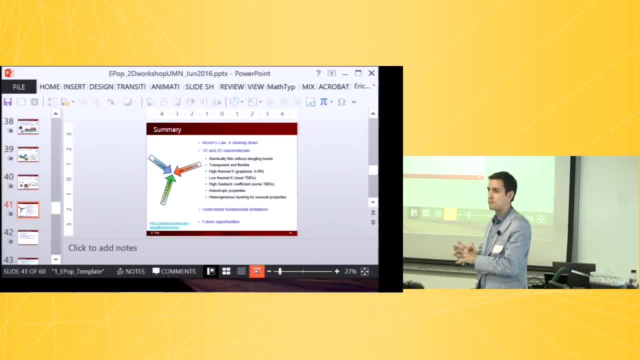 But at room temperature and above it's mostly phonon-phonon scattering. It's either with a substrate or with intrinsic phonons. Yeah, Two questions, Mm-hmm About the velocity right. Yes, So those are very nice measurements. 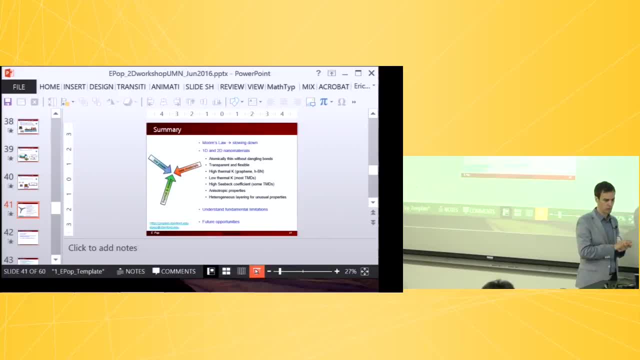 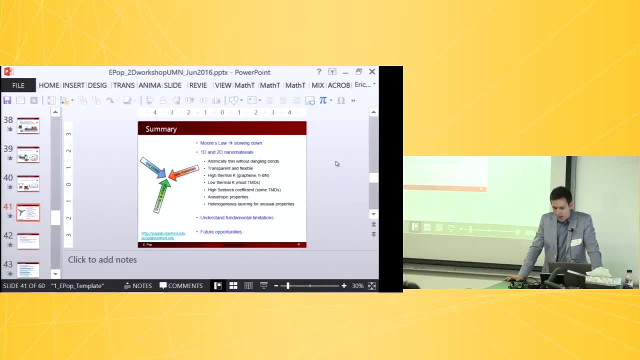 Is the velocity saturation? have you looked at other materials And I assume it's related to the optical phonon energy. but does it correlate with the optical phonon energy and effective mass? Which velocity are we talking about? sorry, You had drift velocity. 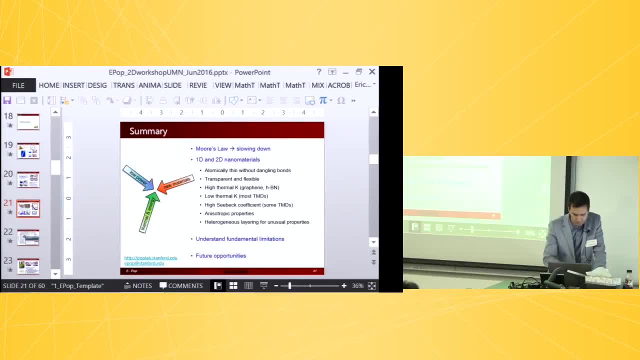 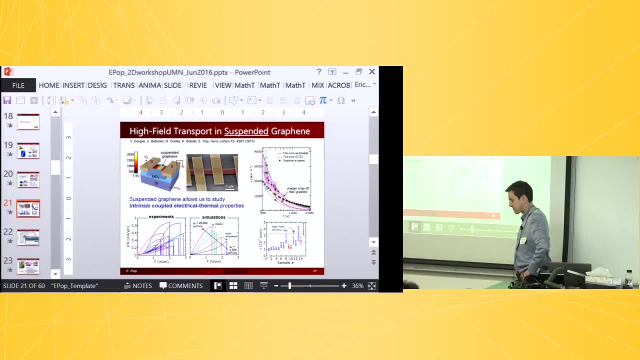 Oh, yeah, yeah, drift velocity on suspended. yeah, Near the start. Yes, yeah, yeah, yeah, this plot, That's right. yeah, yeah, So does it match up with optical phonon energy kind of theory? It does, yeah, yeah. 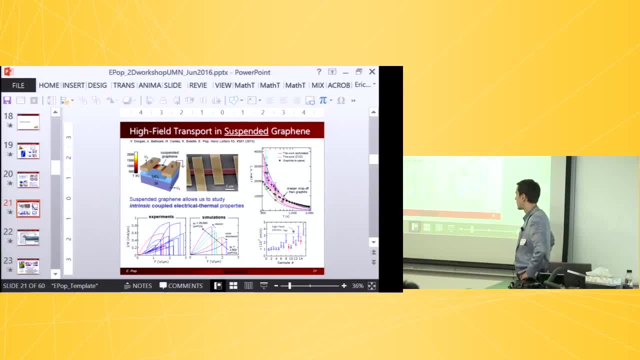 And you might have used that in your paper. I did yeah, Yeah, yeah, we did yeah. So the question was: how does the drift velocity estimated here from suspended measurements match up with the theory right, And is it truly limited by which phonons right? 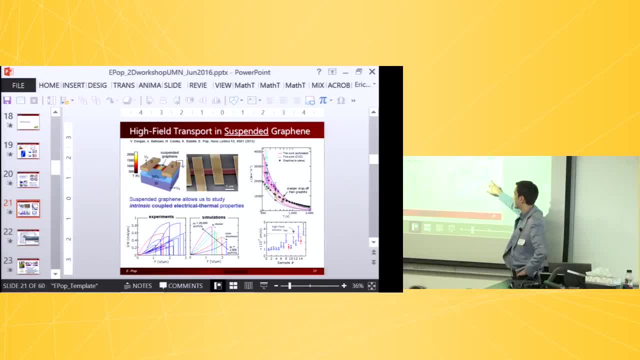 Yeah, so the dashed line right here is the calculation based on the intrinsic optical phonons in graphene, right? So that's right. So this should be that. So this is about 3 times 10 to the 7th right. 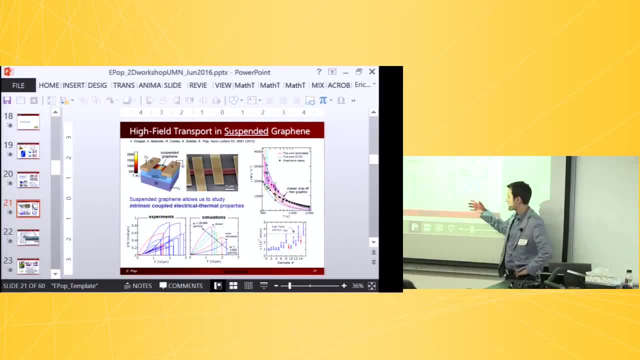 And so because we were struggling with lots and lots of samples and they were not really all the same, we said we're just going to take all the samples we made and put them in the paper. And so here's a measurement, actually by sample number. 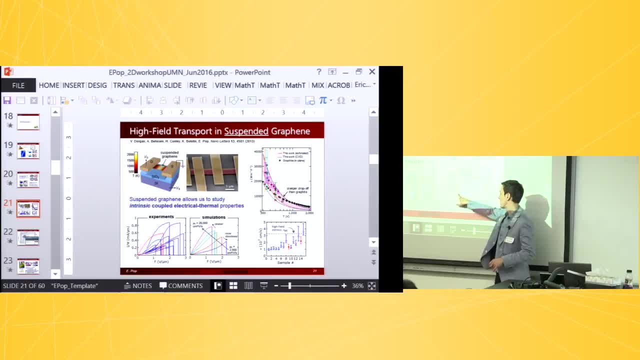 And you can see that some of our- probably our- more disordered samples were estimating only 10 to the 7th, but from some of the better ones, with error bars and whatnot, we seem to be approaching what I think is the intrinsic limit for the material. 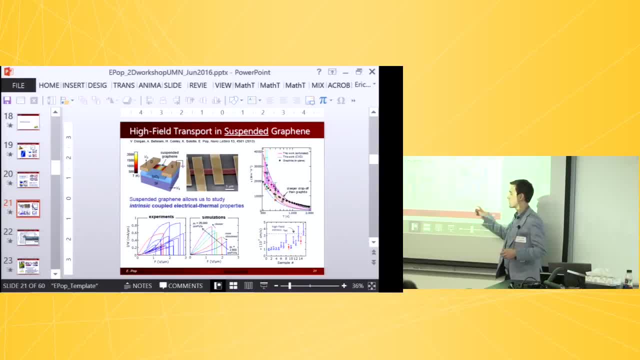 So non-uniform, That's right. That's right, Yeah Yeah, Because these measurements are done at high field, high temperature on a suspended sample And these are actually not pulsed. We've done some pulsed measurements as well, but these are not pulsed because there was not significant hysteresis here. 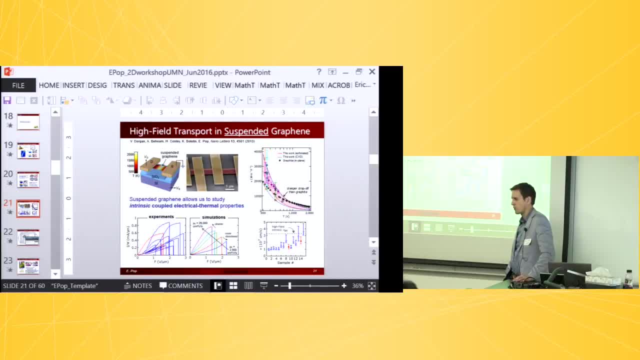 So the pulse measurements are probably better. if you have, I mean, they're obviously good. if you have hysteresis, You're not going to be able to get rid of the thermal component in pulsed measurements because this is just too fast thermally. 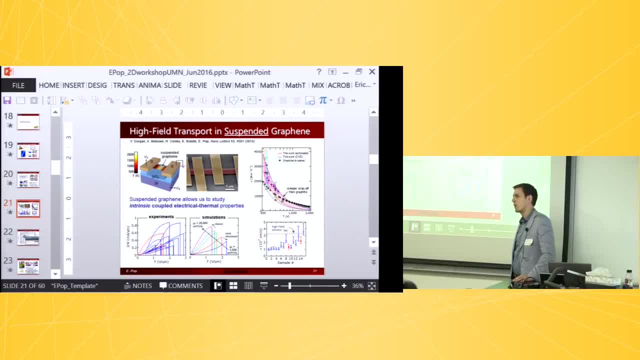 You know the heat will get out in less than a nanosecond And there's just no way we can. we can't do pulse measurements right. So from a thermal point of view, these measurements are always steady state. from a thermal point of view right. 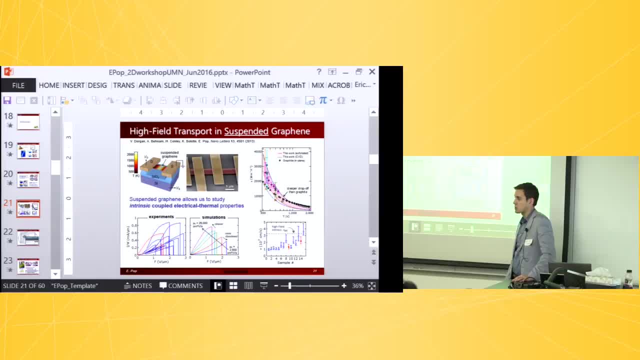 But electrically, yes, if you have charge trapping, of course pulse measurements will help. Yeah, Yeah, But I was thinking thermal. but you're right, Right, Okay, So maybe it's best to move on to our last talk. So let's thank Eric again. Thank you. 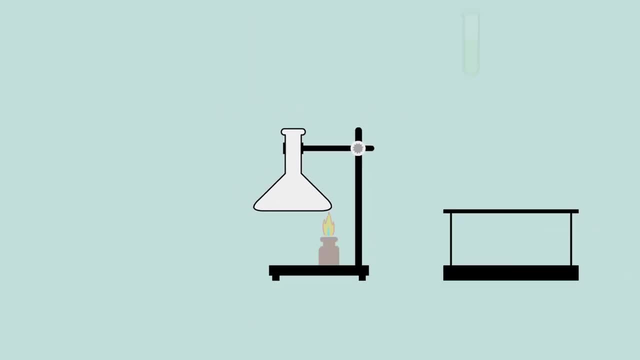 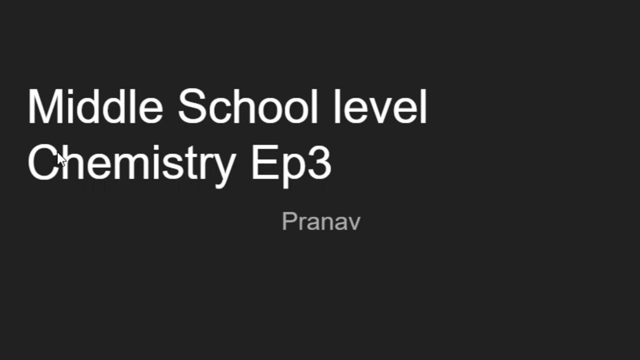 Hello, my name is Pranav and I'm going to be teaching you middle school level chemistry, And today we're going to be learning about some basic bonds and how to balance some equations. Keep in mind that there are actually many types of bonds, but we usually refer.